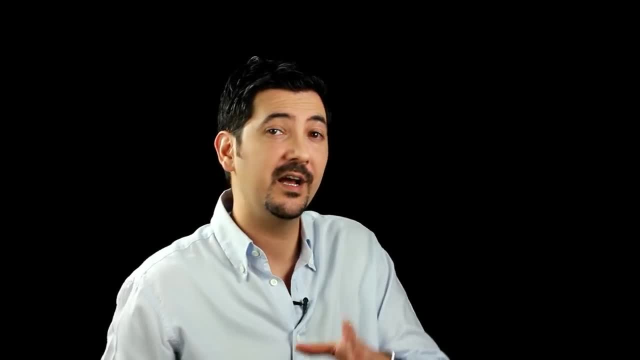 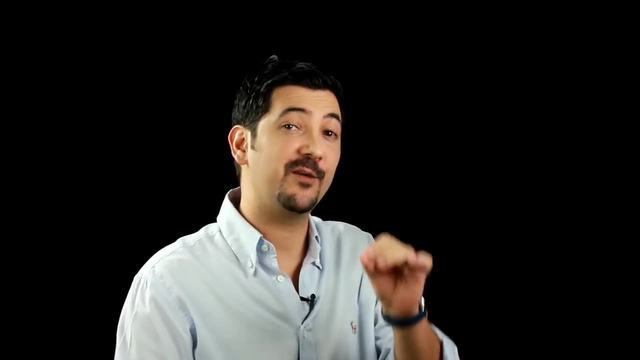 I've never seen any professional in my 10 year management consulting career who hasn't run a project. It just so happens that sometimes they don't know they were managing projects, But they were projects indeed. So if you're looking for a simple enough framework to understand project management, 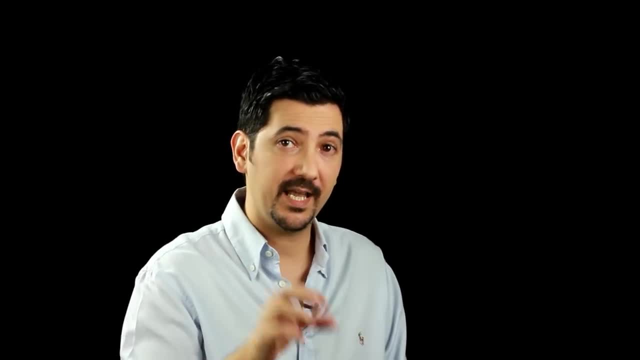 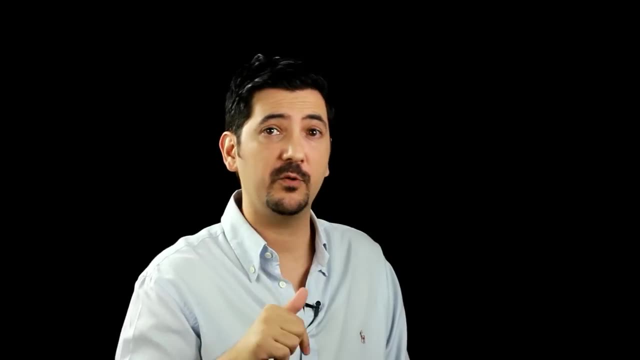 and implement it at work, then you're on the right place. By the end of this video, I'm confident that you'll be able to add project management as a skill in your resume. Also, this video is for you if you're preparing for your PMP exam or CAPM exam. 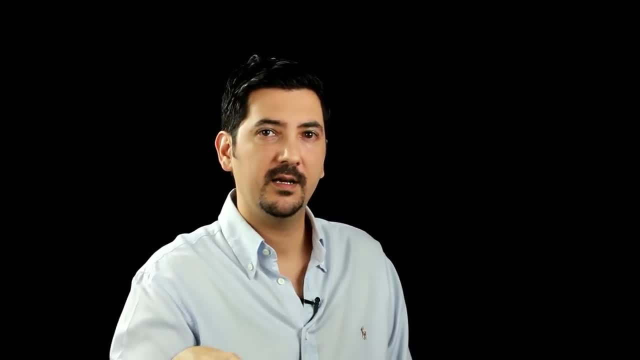 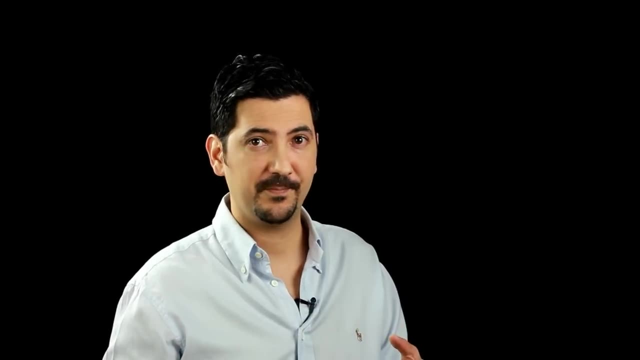 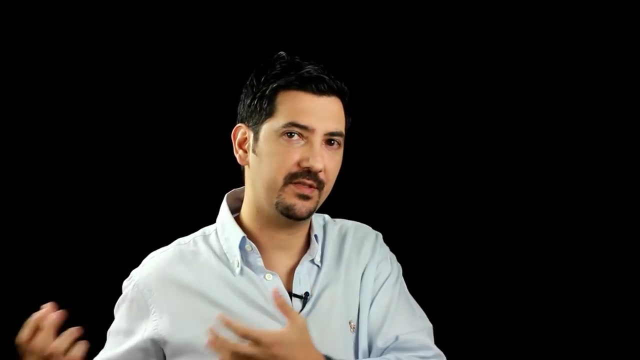 Once you finish this mini course, the PMBOK guide will be a lot easier to understand. See, the PMBOK guide is over 500 pages long. It's a very, very long and quite boring book, I must say So obviously I can't share everything in this short video that exists in PMBOK guide. 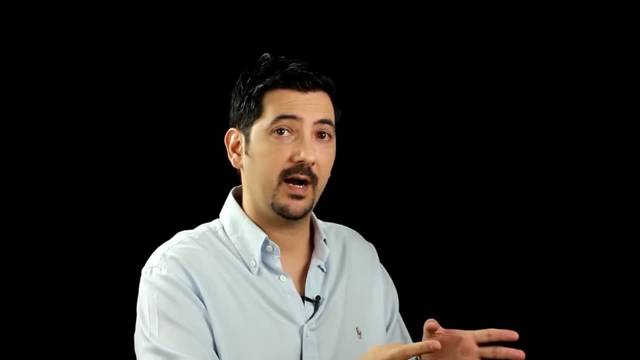 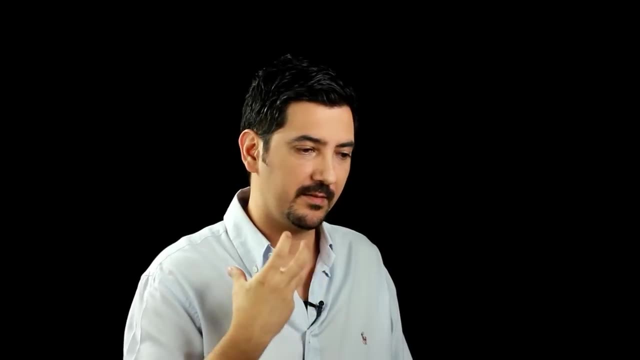 but if you watch this video without skipping, the PMBOK guide will be so easy to follow for you, Because it's all about understanding the fundamentals. Everything else just becomes very easy to follow. When I took my PMP exam around 6 years ago, 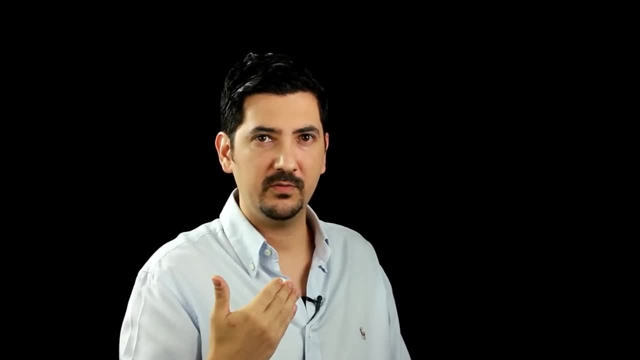 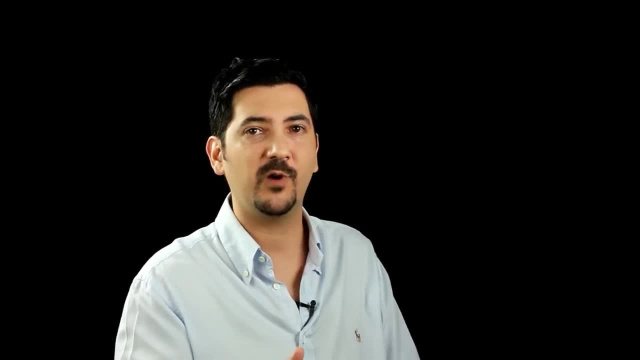 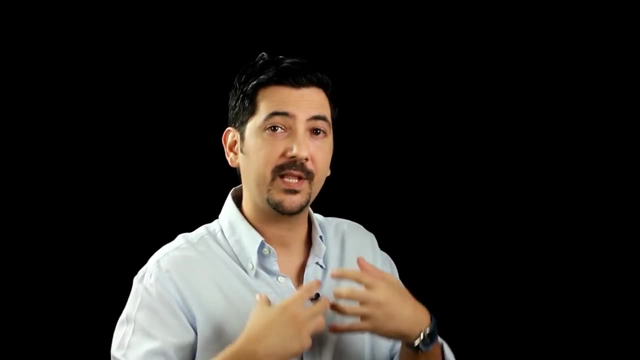 I almost aced it. I scored one of the highest points at that time, And the only reason why I scored so high was not because I spent hundreds of hours studying. On the contrary, I just understood the fundamentals, And once you understand the building blocks, as I said earlier, everything else becomes. 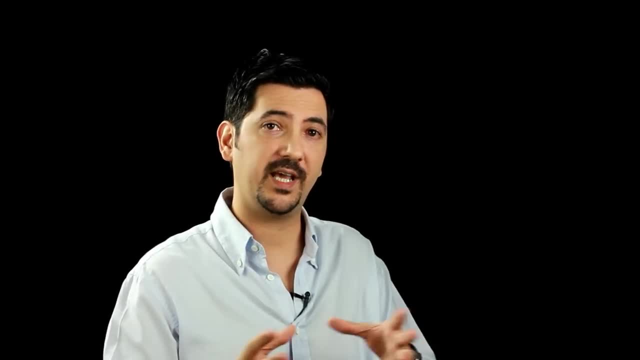 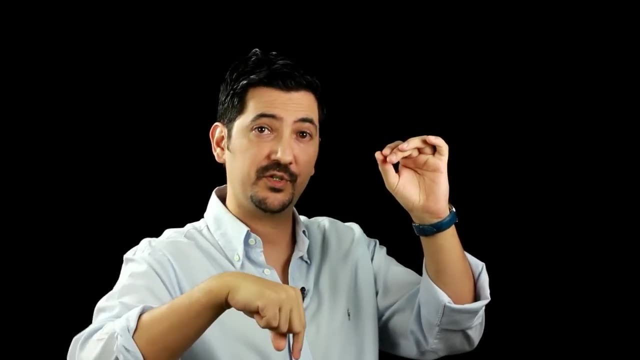 so easy to follow, So I suggest you watch the entire video without skipping. but if you're interested in learning just certain elements only, then you can look at the description box for the index of the video. Good, So let's get started. 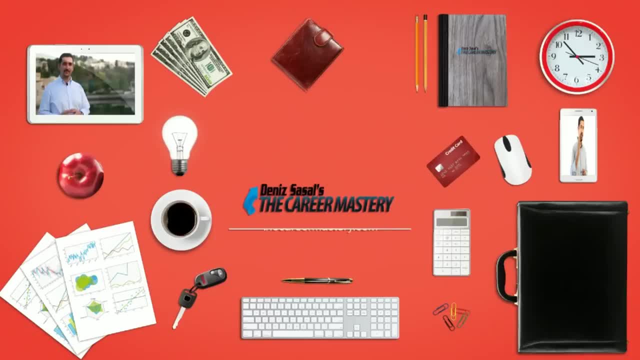 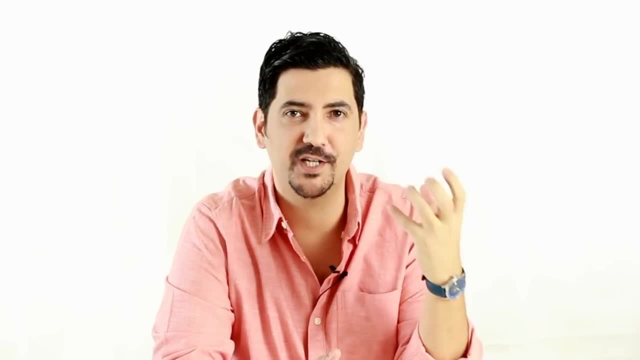 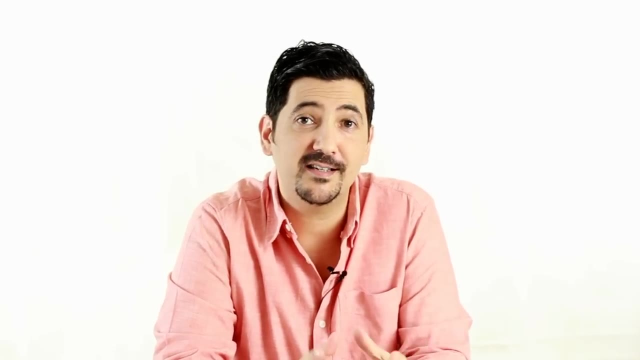 I mean, what is even a project? It definitely has a sexy tone to it, right Project? I wonder how it sounds in French, Roger. So here's the definition: Project is a temporary handover to create a unique solution. 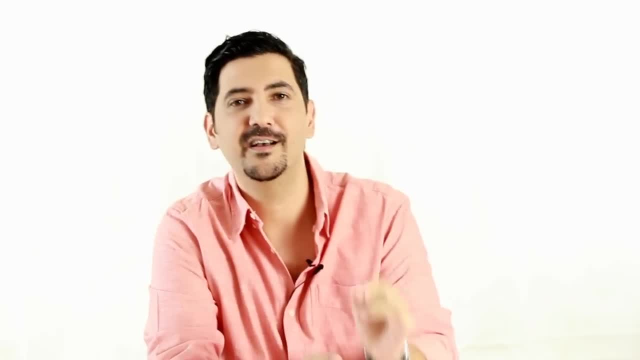 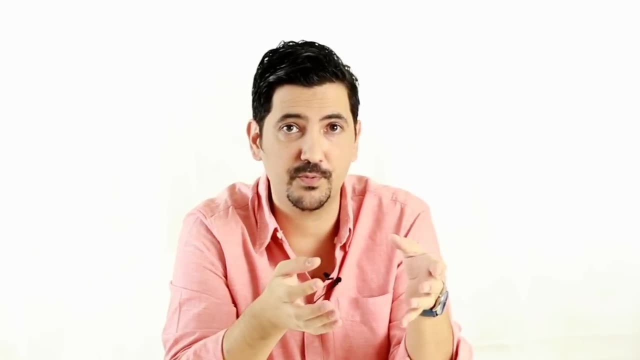 Yeah, but that's operations, No, No, No. A project and operations is fairly simple. A project ends, So it's temporary. You implement your project, You close it, You create a unique product or service or whatever the outcome you wanted. then you're done. 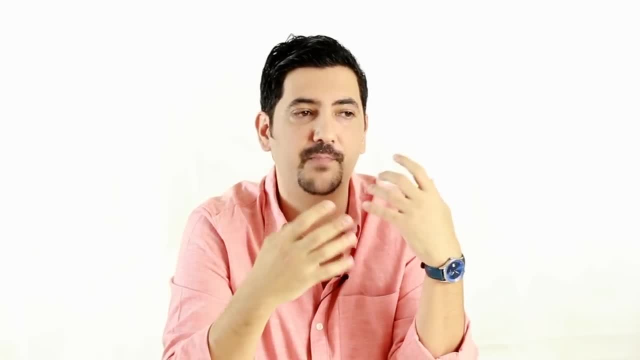 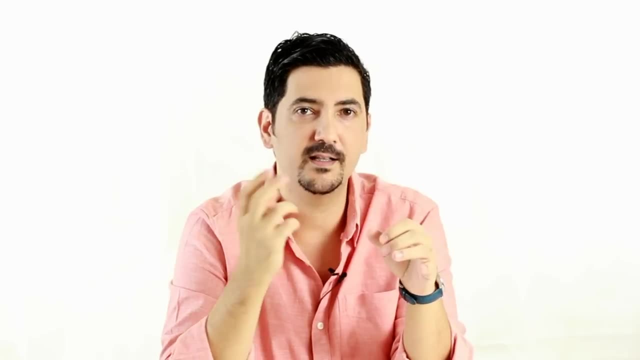 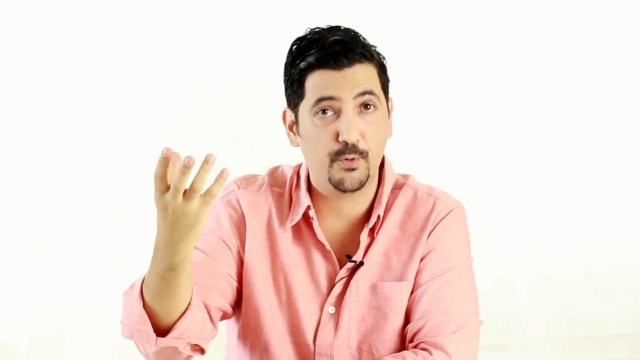 Whereas in operations it's an ongoing effort, it's repetitive. So you may have also heard about the terms program and portfolio. Let me just quickly explain them here as well. Program is multiple projects put together, Combined, And portfolio is similarly multiple programs put together. 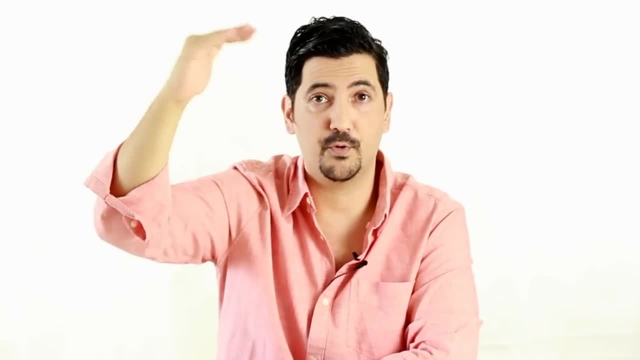 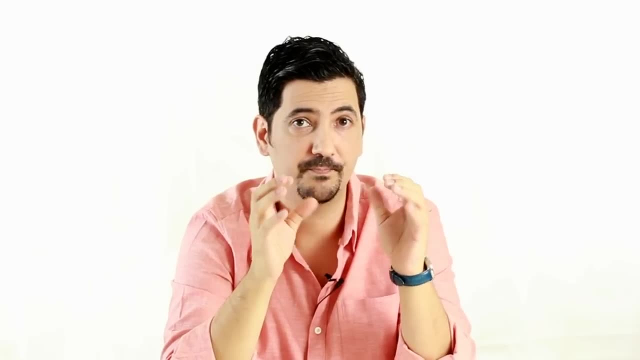 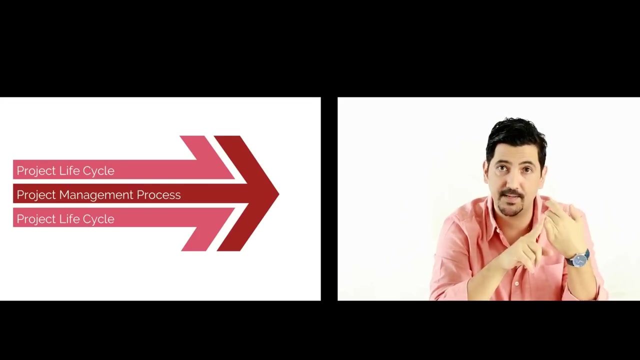 So it's basically project program and then portfolio. Now, before I go further and dive deep, you need to understand something very crucial: To run any project, you need two methodologies. The first one is a project lifecycle and the second one is project management process. 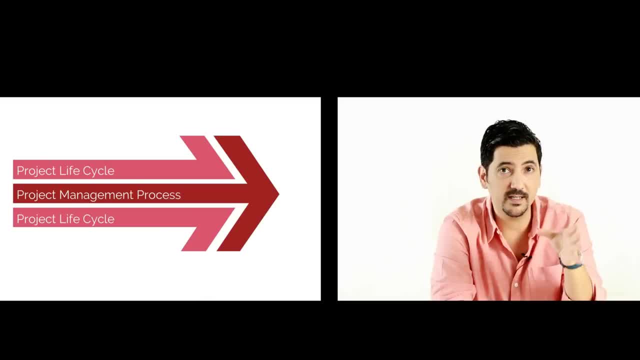 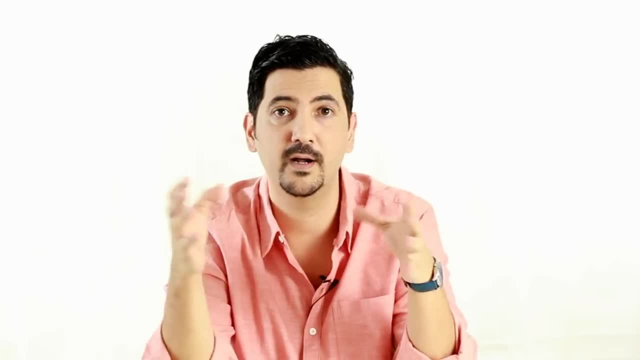 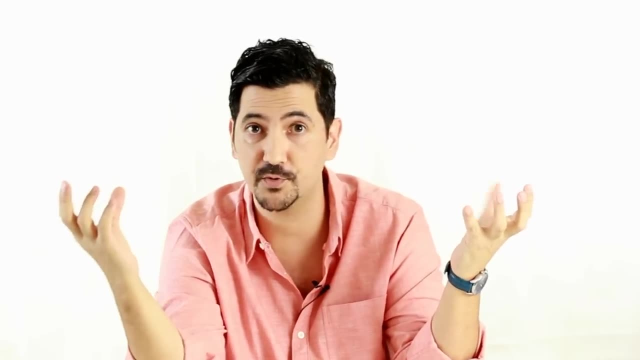 Most people confuse these two. OK, If it's not clear, you can kiss that PMP certification goodbye. It's absolutely amazing how many content creators in YouTube or elsewhere confuse these two. They are not interchangeable. You cannot afford to confuse a project lifecycle with a project management process. 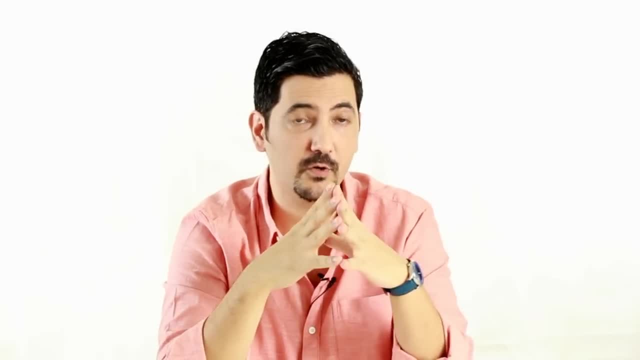 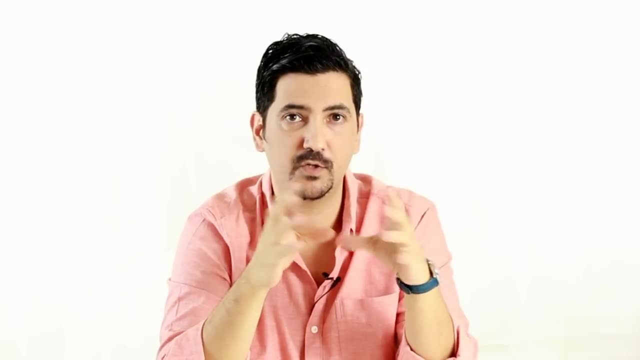 But don't worry, I'm going to make it very simple for you. So let's start with project lifecycle. Project lifecycle is unique to a project, to an industry, to your needs. It's highly customizable. Think of it like this: 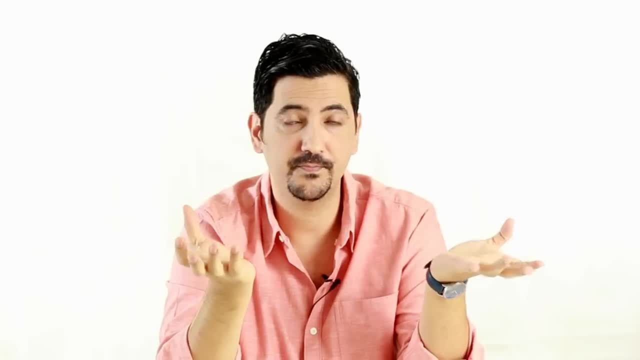 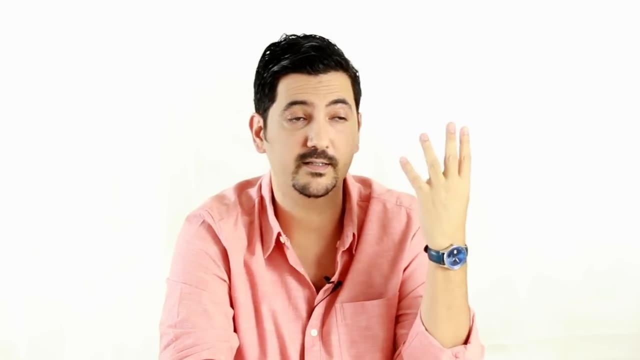 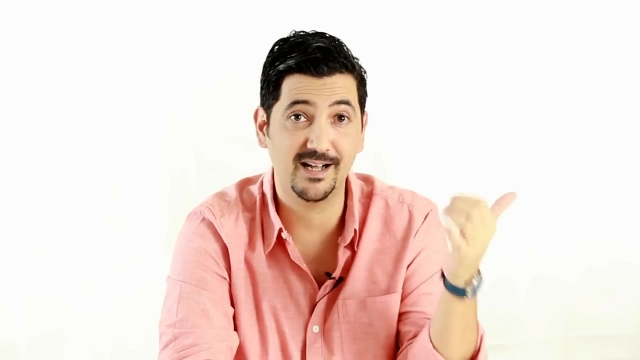 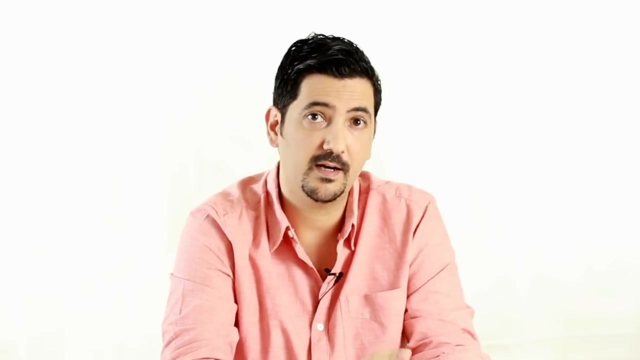 A human development is a project, isn't it? So your lifecycle is conceiving, birth, childhood, then teenagehood, adulthood and then death. Easy stuff, right. So now, if it was an IT project- I'm not an IT, but it would probably look something like: 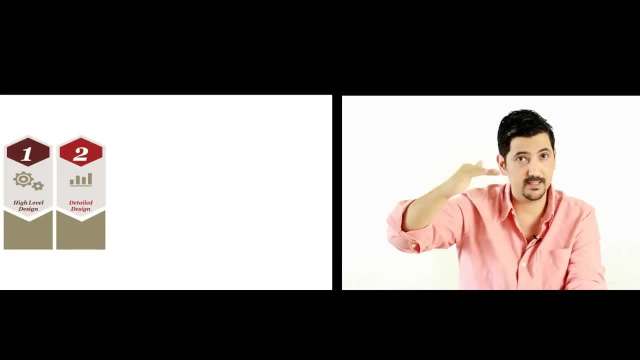 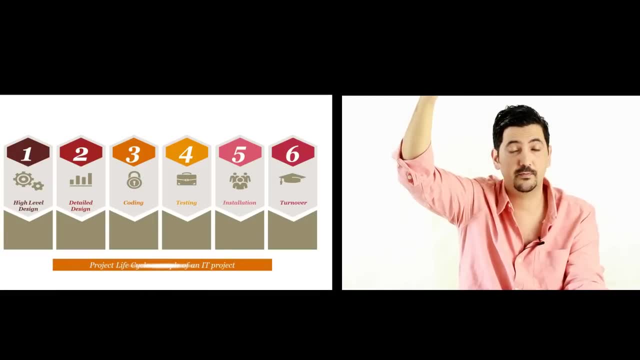 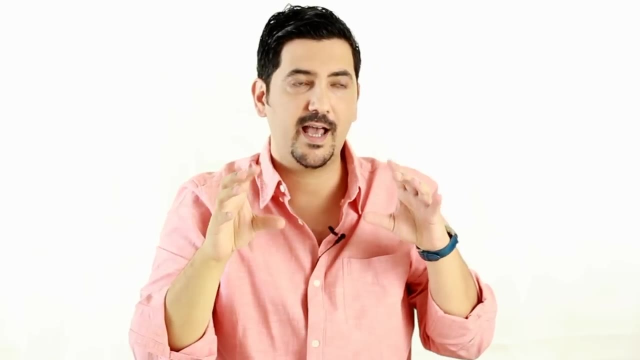 this. It would be high-level design, then detailed design, then coding and testing, installation and then finally, probably a turnover if it was done for a client. So this is project lifecycle, And here is probably where the confusion comes from The term cycle. 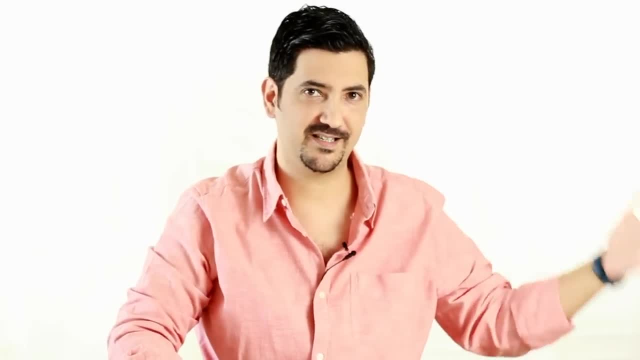 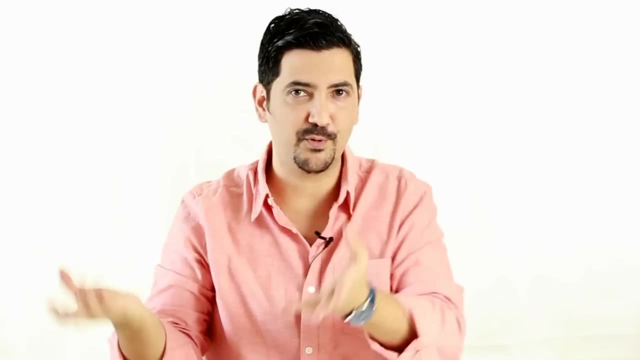 That's what's confusing, Because after you die, you don't get to be conceived again and be born again, I think. But who knows? Or once you hand over the product to the client, you don't get to be designing that again. 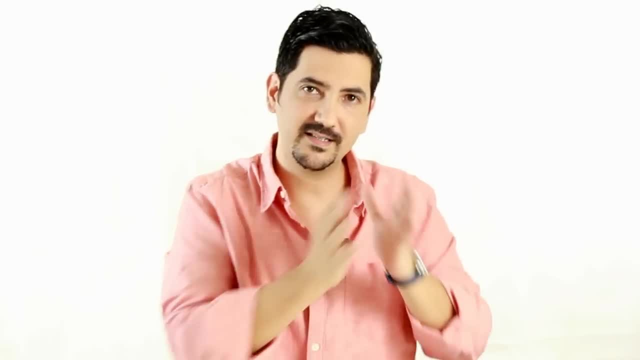 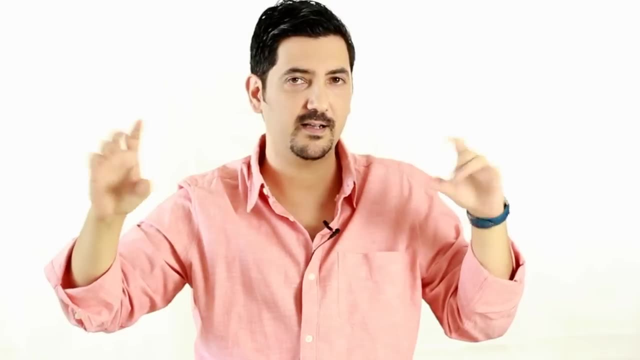 So it's not actually a cycle, it's just a confusing term they use. It's sequential, It's the sequential steps of various phases of a project, And these phases- I'm going to repeat it again- are unique to your own project and 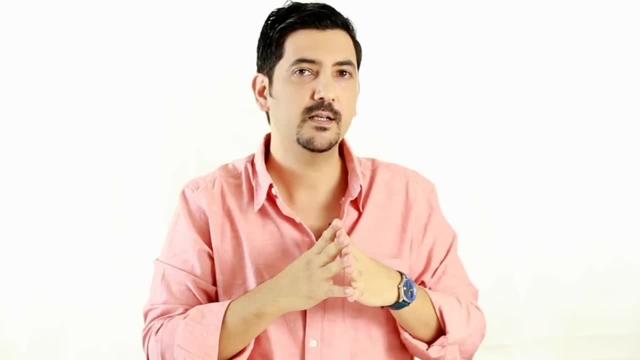 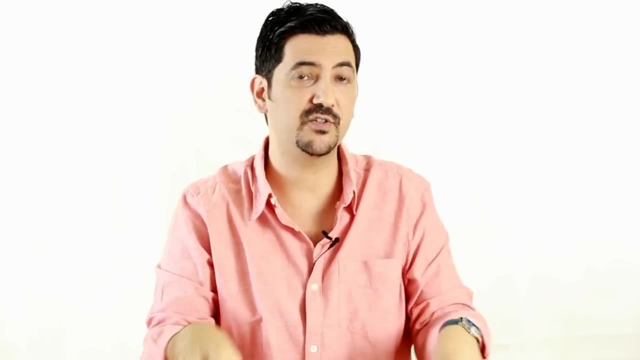 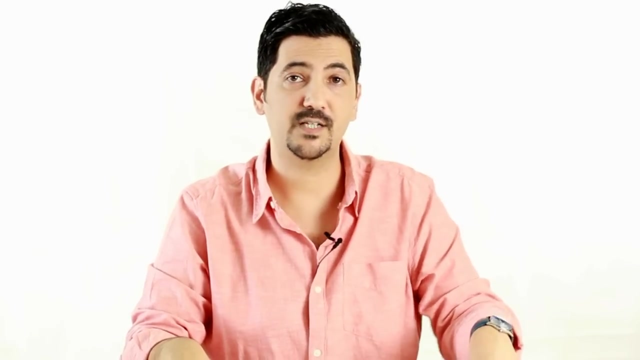 your needs, So you create your own cycle. So a project lifecycle may have one phase or multiple phases. Like the examples I gave earlier, There is no single way to define the ideal structure for a project. For example, one company may treat a feasibility study as first phase of a project, another. 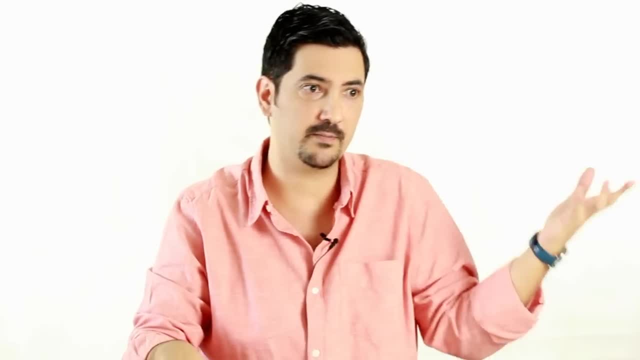 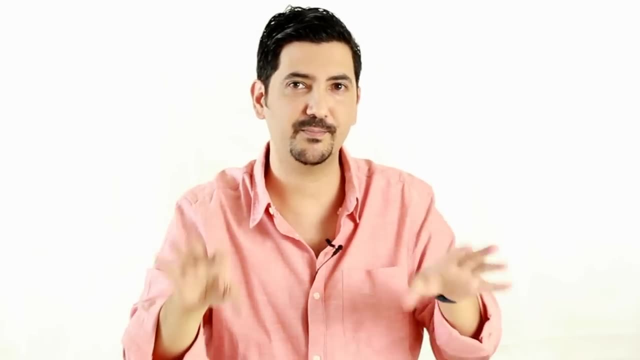 may treat that as a third phase of a project and another may not even include it at all. It's custom made. I know I said this multiple times- custom made, but you'll soon understand why I had to repeat it multiple times. 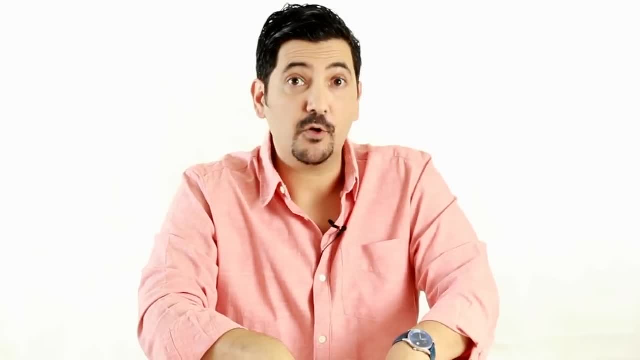 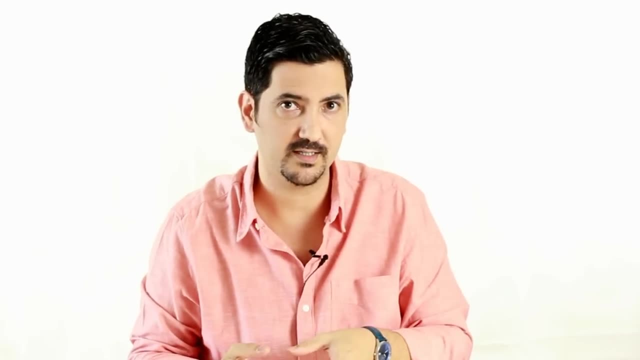 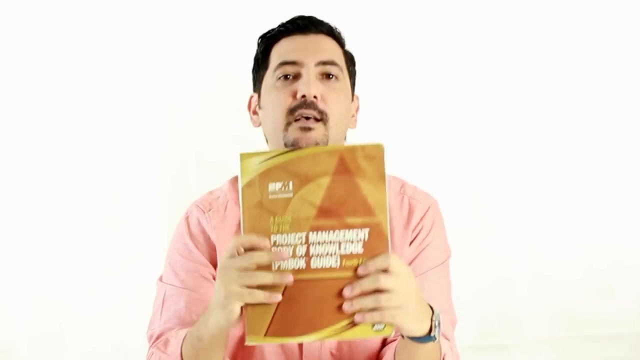 Just be patient, Just bear with me. Now let's talk about the second element that you need to run any project, And that's the project management process, Your process groups. See if you're following PMI's project management body of knowledge, then your process. 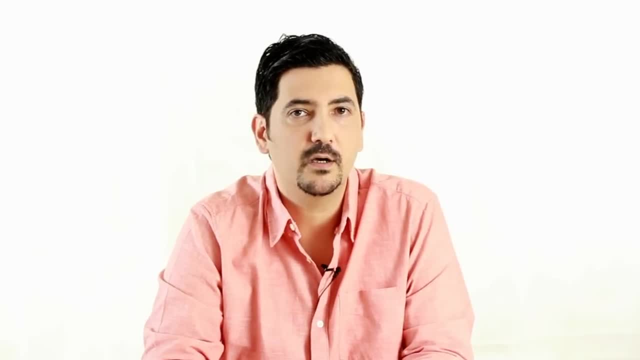 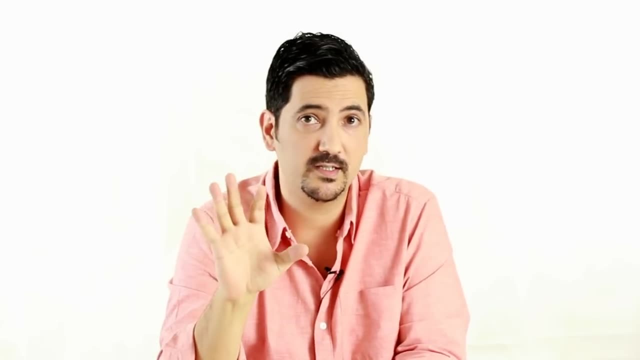 groups aren't quite customizable. So you can customize the processes, but not really the groups. We're going to talk about that soon. So we have 5 process groups to learn here: 1. We have Initiation, 2. We have Planning, 3. 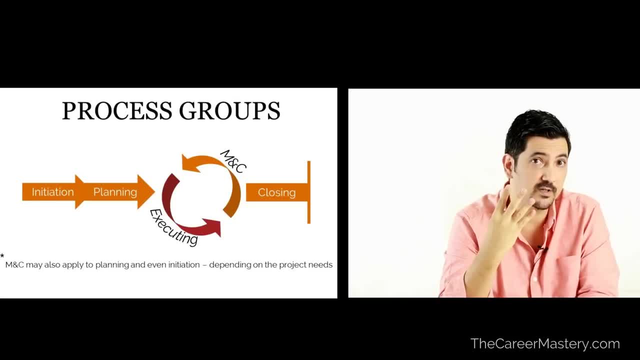 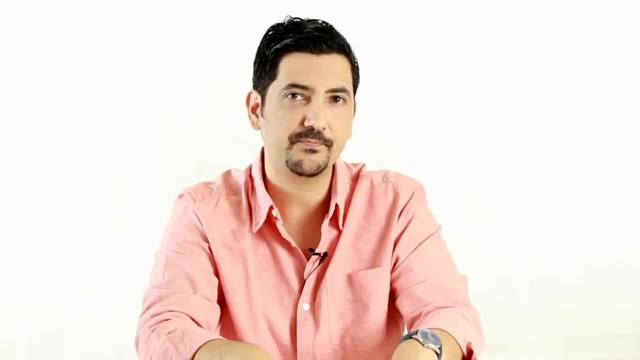 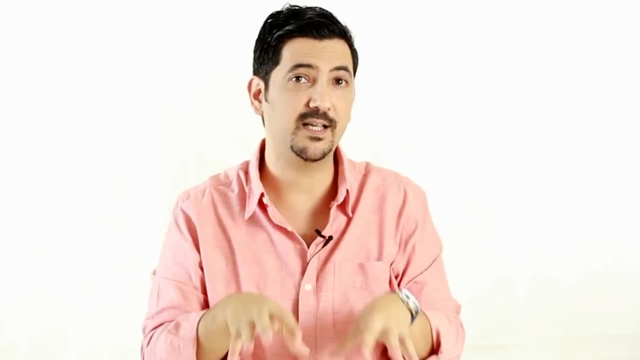 We have Executing 4. Then we have Monitoring and Controlling and finally Closing. These are kind of set in stone. You can't really play around with them that much. Now, here's where all the confusion arises. For those of you who are interested in taking a PMP test, I will now tell you the single. 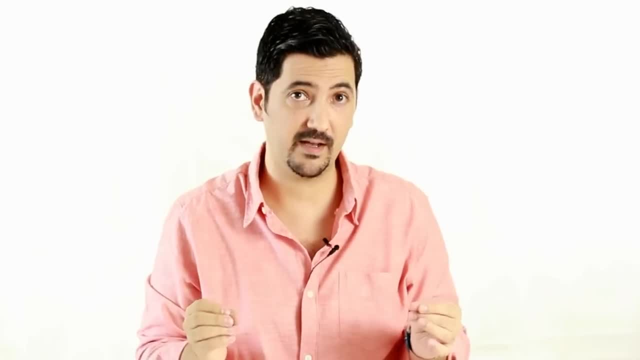 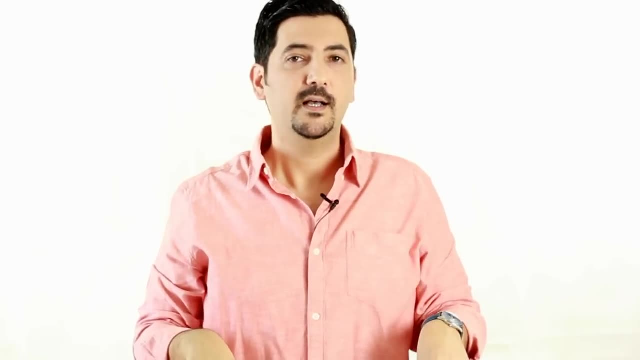 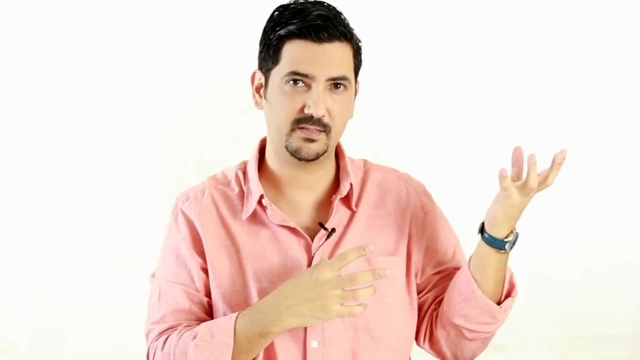 biggest reason why most test takers fail, And it's all because of confusing lists. This is what I am about to share. So remember how we talked about that: the fact that project life cycle is highly customizable. You know, I bored you to death with it. 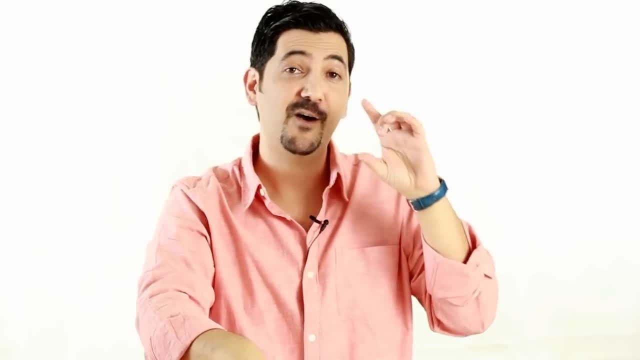 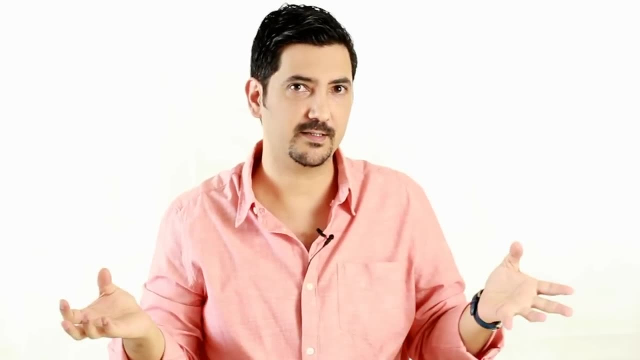 Customizable, Customizable, Customizable. So now what we do in real life is for small projects. we really dumb things down. We simplify things Instead of attaching process groups to every single thing. We simplify things, We simplify things. 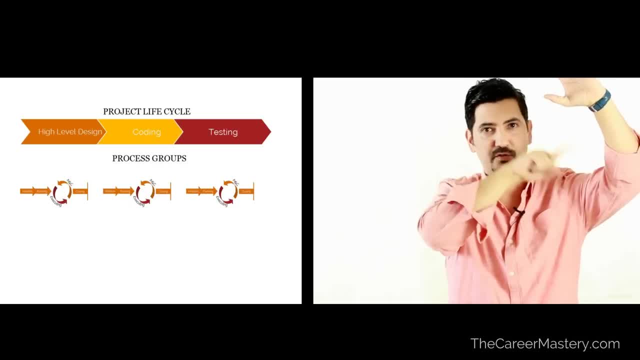 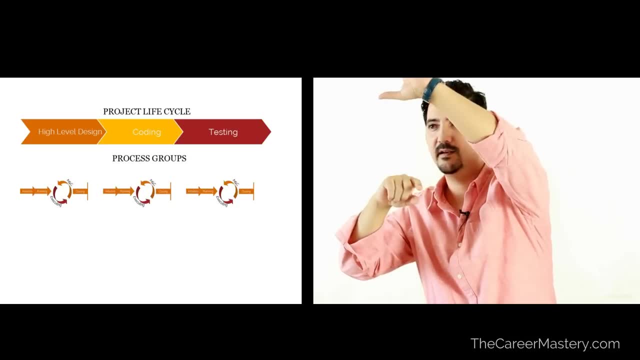 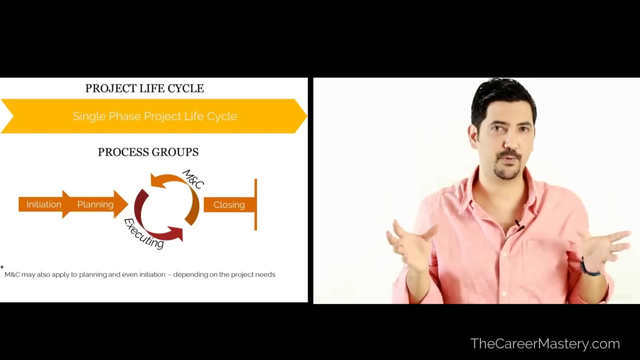 We go through the whole phase of a project life cycle: Conceiving process groups, Development process groups, initiation, planning, Execution, MNC and Closing, Then death. Instead of doing that In real life, we attach the process groups to a single phase project life cycle. 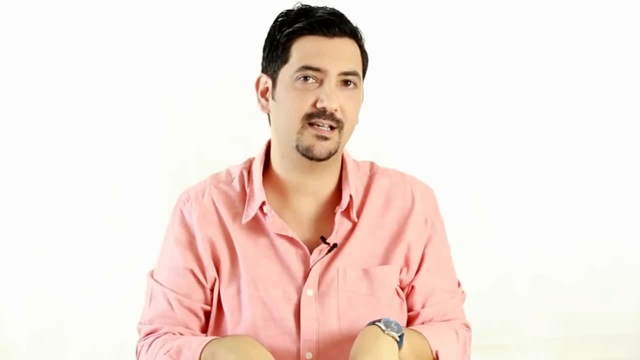 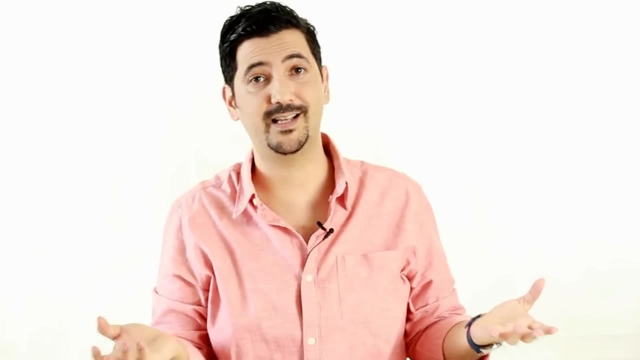 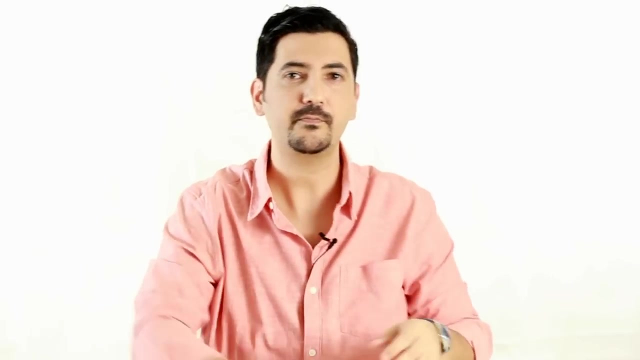 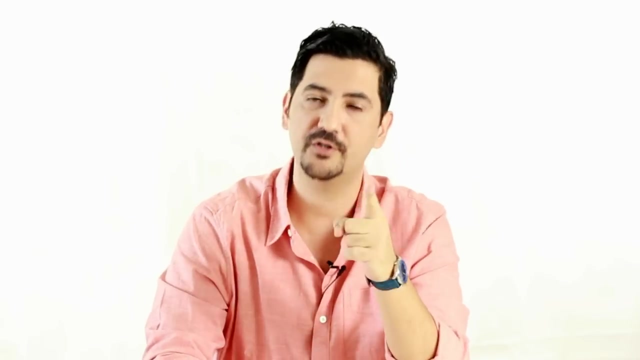 Now, I hope this is clear. This makes things easy to run the project. for us, It's less complication. I mean, make things more complicated than they should be. Your project life cycle isn't Initiation, Planning, Execution, Monitoring and Controlling. 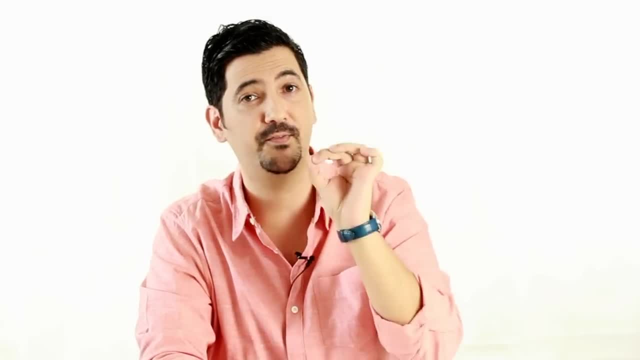 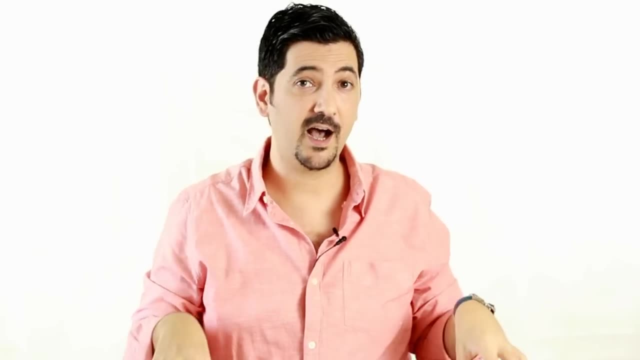 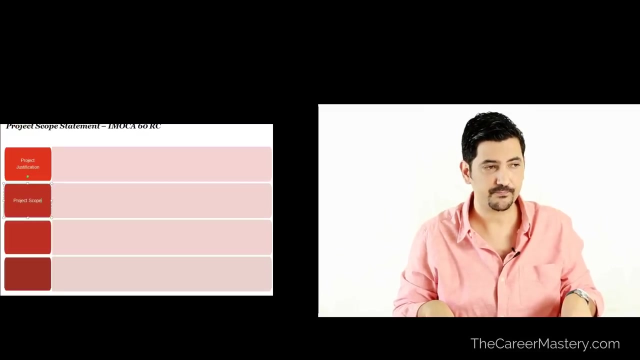 and Closing. If you don't get this right, I guarantee you that you will fail the exam. Now we are going to talk about the process groups, And while I am explaining that, I will also simultaneously run a project for you to demonstrate how it works in real life. 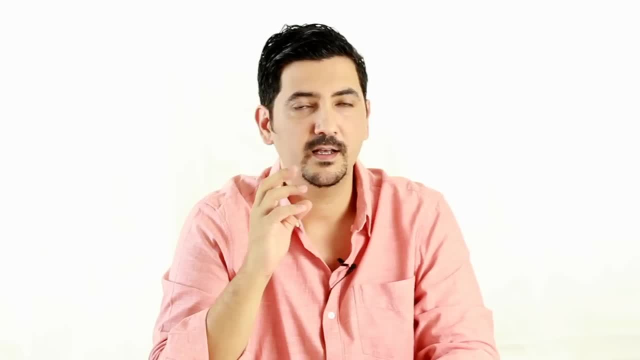 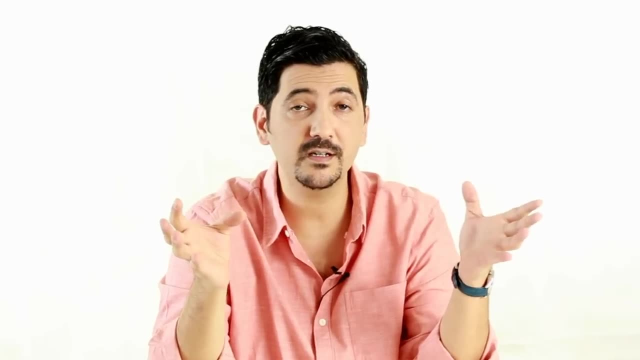 But before I get there, I want to share something very quickly with you. It's about PMP. If you are looking to get a PMP or CAPM degree so you can advance in your career and get better jobs, don't, Don't do that. 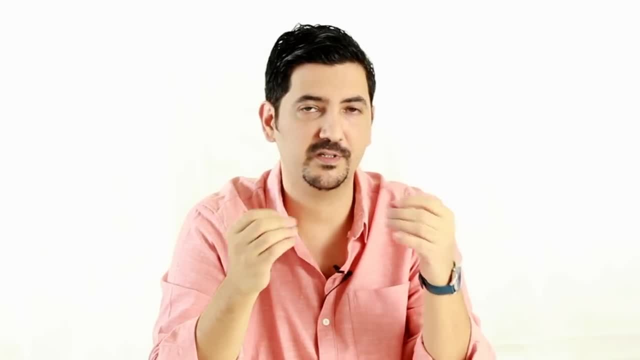 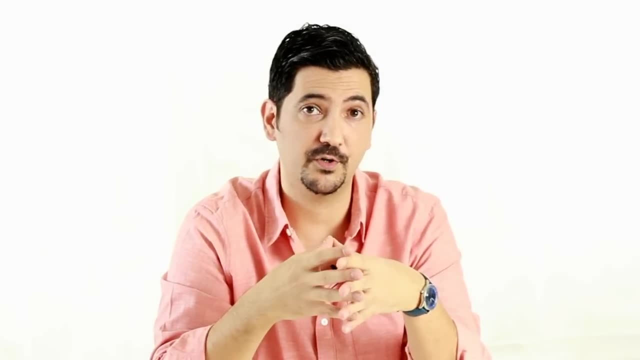 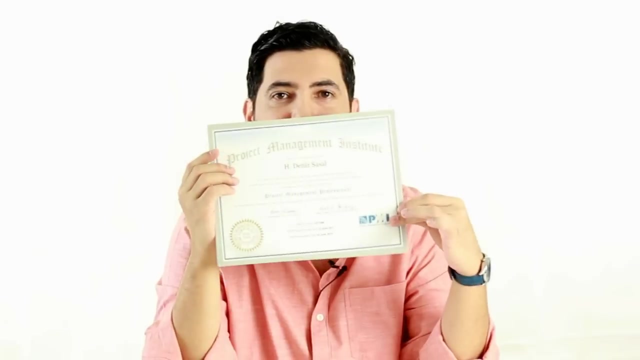 It won't really help you as much as you think. Learn project management. It's awesome, It's an incredible field. It's an incredible complementary practice. Everybody should learn project management. But don't you think that by getting a piece of paper like this or this that you are going? 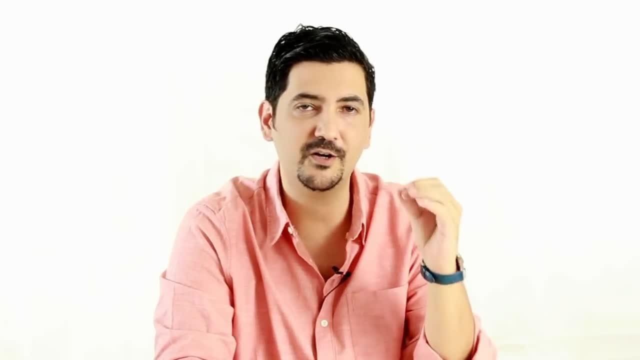 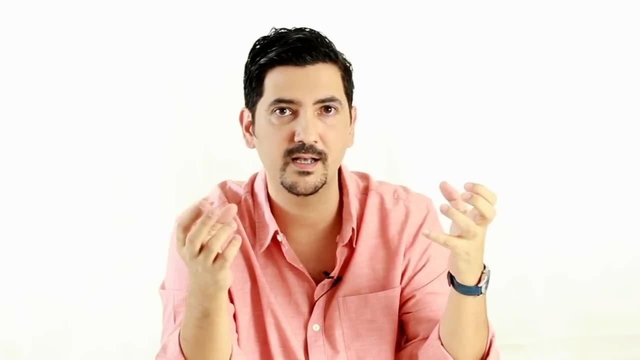 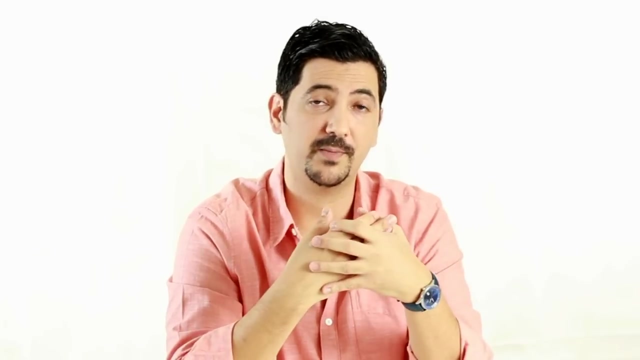 to advance in your career. Don't do that. It's not going to work, Because every company has their own methodology and have their own terminologies and frameworks. You know. So if you are looking to get a PMP or CAPM degree, I suggest you check out my LIG program. 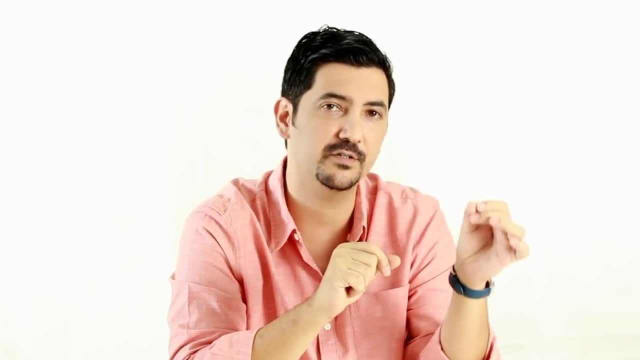 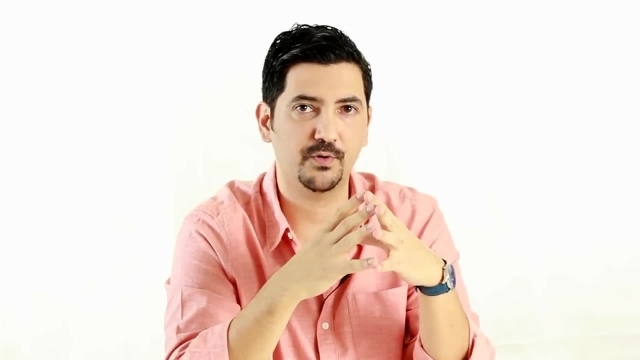 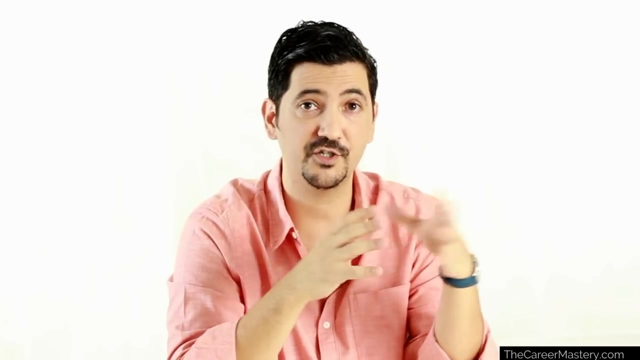 and let that program show you how you can achieve the career you deserve. It sounded a bit like an advertisement break, but it's not. I am very passionate about my LIG program and the results are overwhelmingly positive. So you can go to TheCareerMasterycom and you'll see a link to register to LIG if 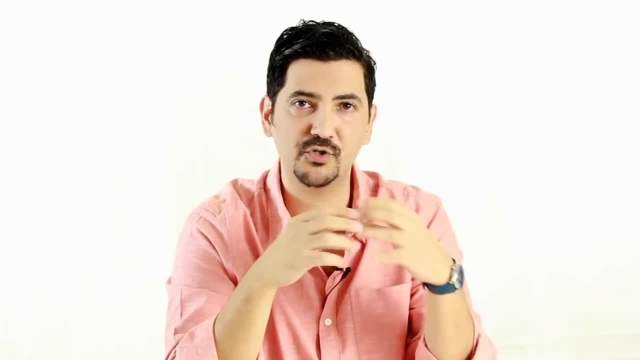 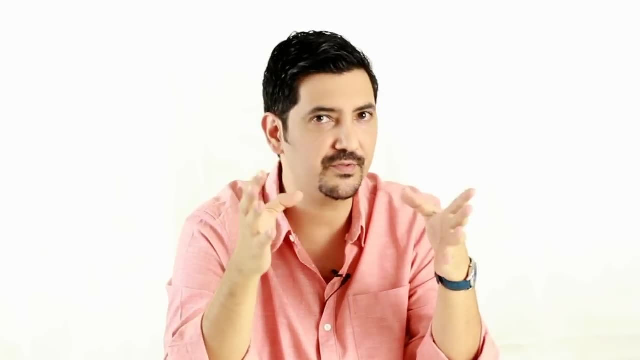 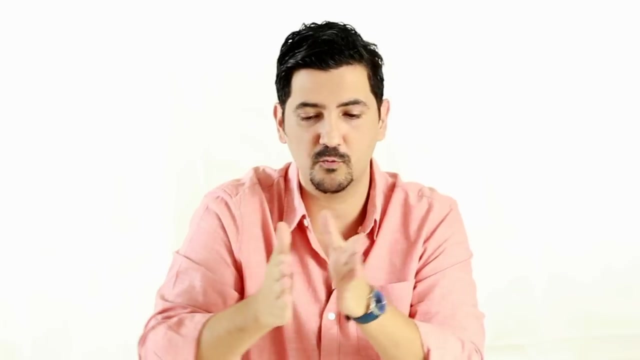 it is active by the time you are watching this. Okay, Most multinational firms have their own in-house methodology to follow, So you'll have to unlearn a lot of the things to learn their way. For example, my employer, PwC Consulting, has a complex methodology for every single work. 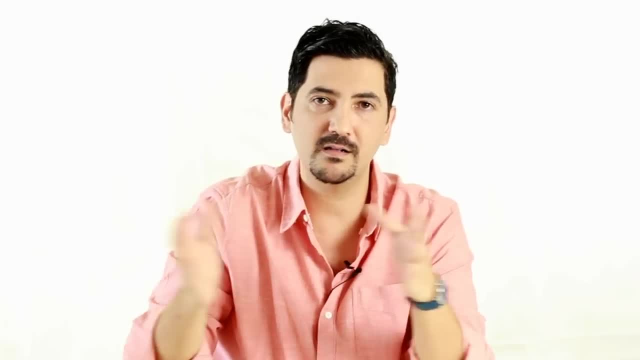 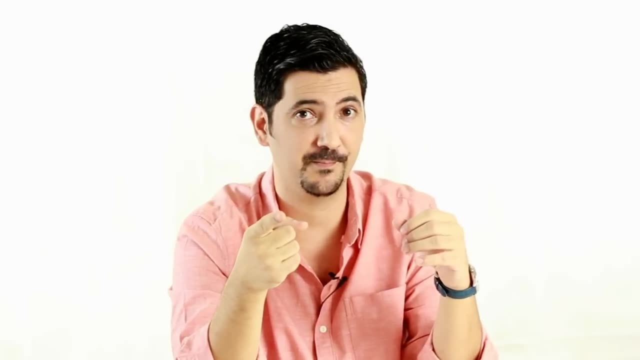 we deliver. It's the best in the world and miles better than PMI's framework or PRINCE2 methodology. So your future employer will have its own methodology as well, But still don't confuse these two. Learn the fundamentals of project management. 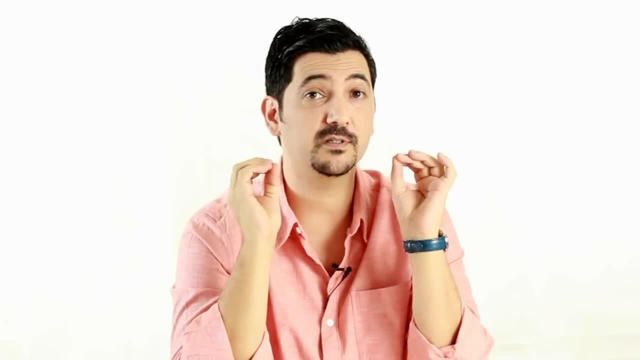 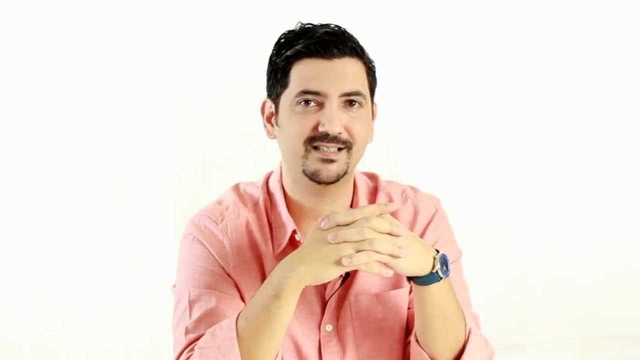 You know, learn everything I'll share in this video. Project management is awesome. It's an incredible practice, But a certificate Not so much. It's highly debatable, Okay, So let me continue. Oh, and one final point on this. 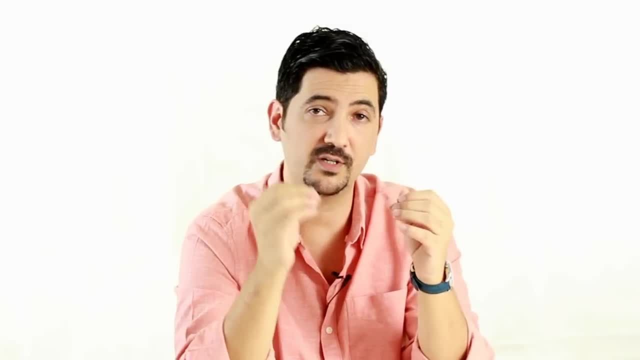 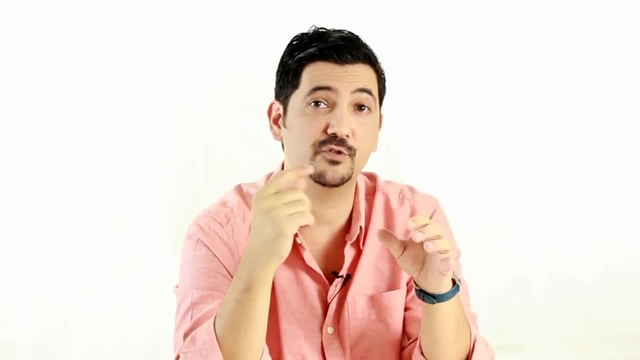 I have a pretty amazing bonus and a guarantee, So if you don't get the results or the jobs you want within 30 days, I will personally work with you free of charge, to get you to where you need to be. Okay, Sorry for the break. 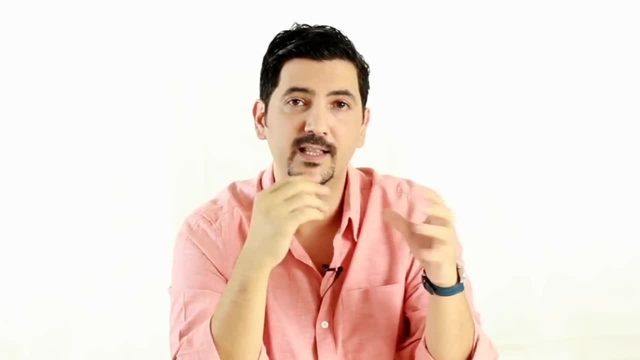 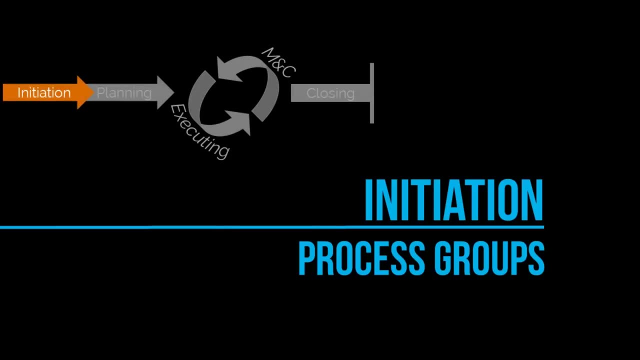 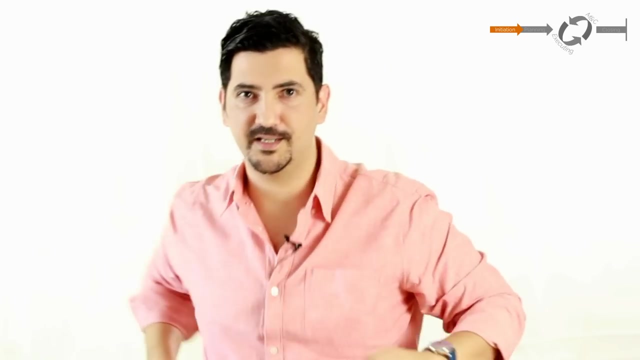 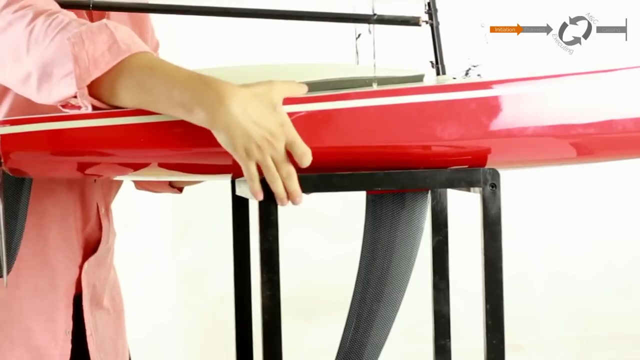 I felt compelled to share that. Now let's start with the first process group, And that's Initiation, To make things very grounded. I will use the construction of this boat as an example. I hope you can see this. It is a huge, huge boat. 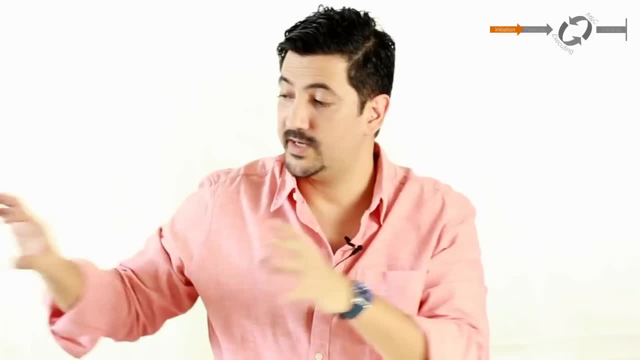 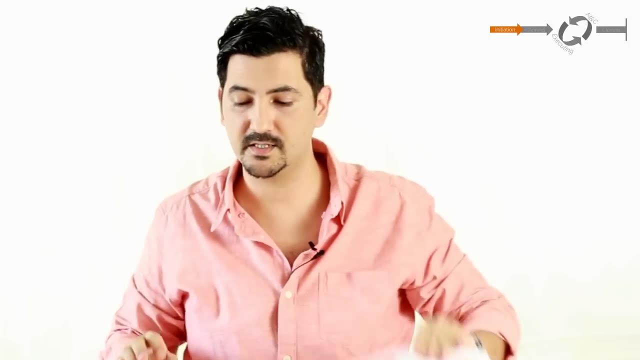 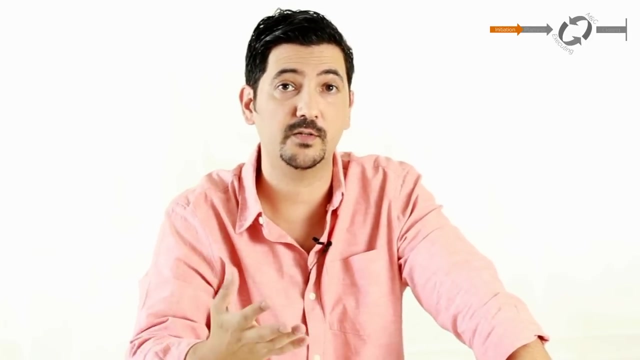 Alright, Okay, So yeah, This is the boat I did last year And I think it's going to be an awesome example to run this session with you. I mean, I could give you examples from my own work history, Obviously. as a manager at PwC Consulting PricewaterhouseCoopers, I ran hundreds of 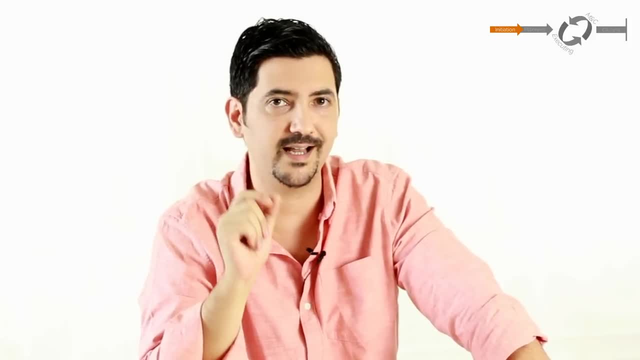 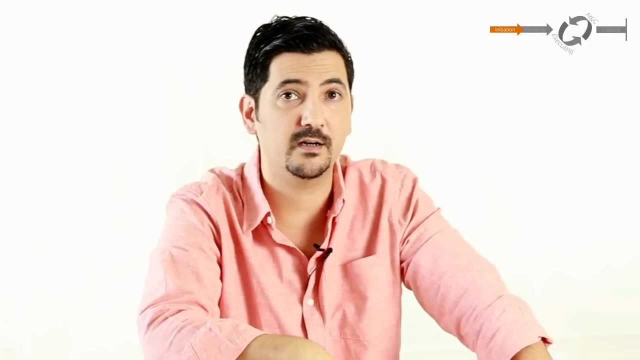 projects, But it would create a few problems. 1. I am under strict client confidentiality agreements. 2. We don't use PMI's framework, So I am going to teach you PMI's framework here, So it won't be very relevant. 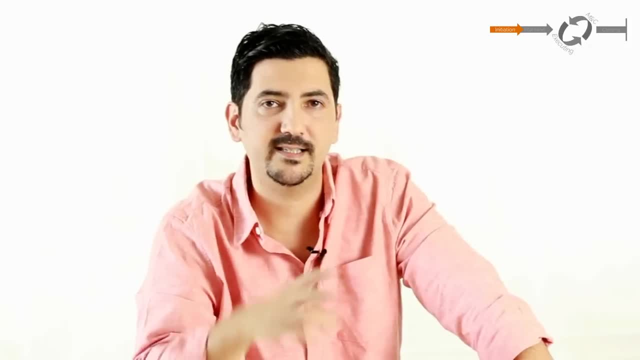 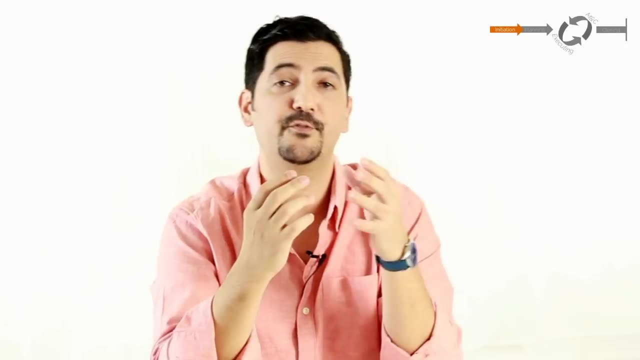 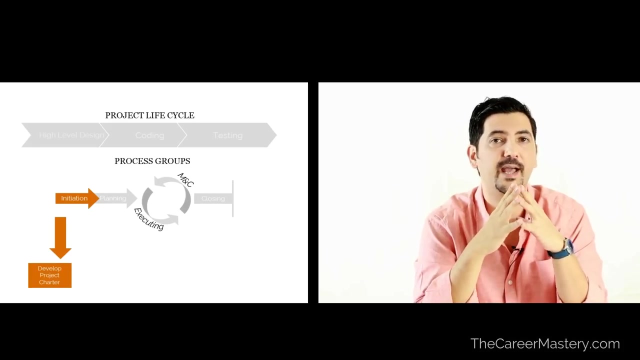 I think using this boat is going to be a lot easier. 3. If you have any questions about designing and manufacturing it with all the paperwork involved, it'll be awesome. So for Initiation Process Group, you have two important processes. The first process is that you develop a Project Charter. 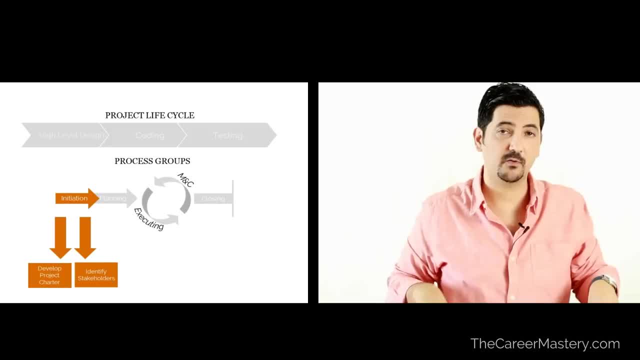 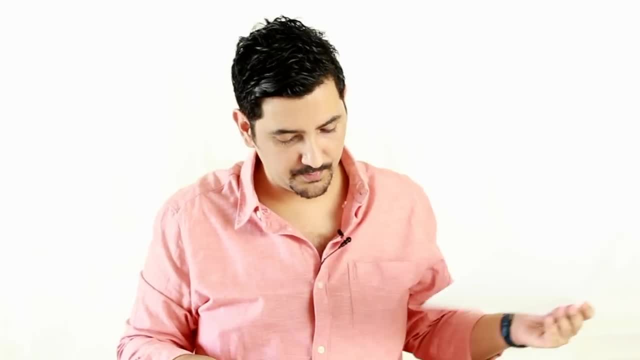 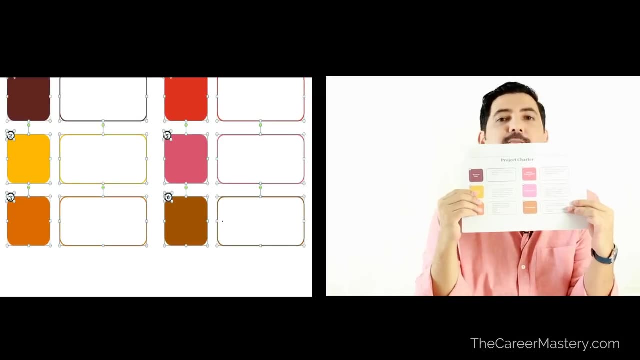 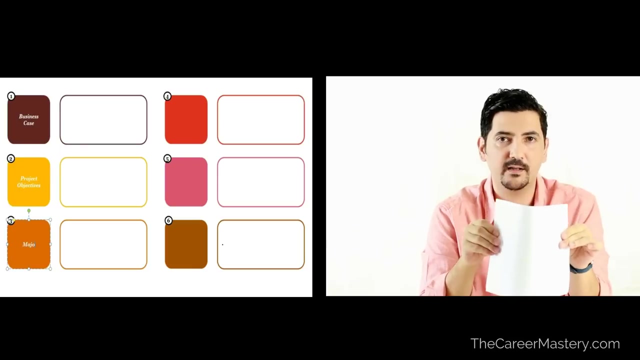 And the second process is you identify stakeholders. Now let's start with Project Charter. So Project Charter is a fairly simple document Outlining a few things. it's like a mini project plan- Very simple one, though Essentially, you are finding an answer to why you are doing what you are doing. 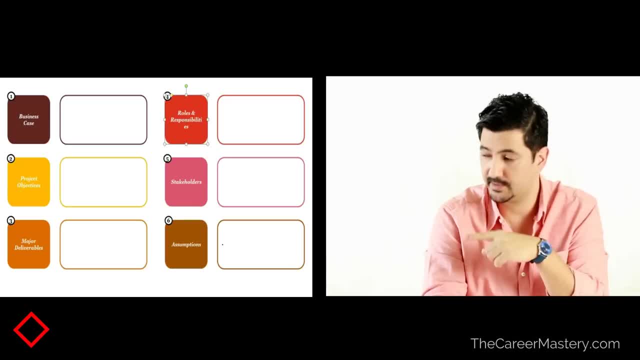 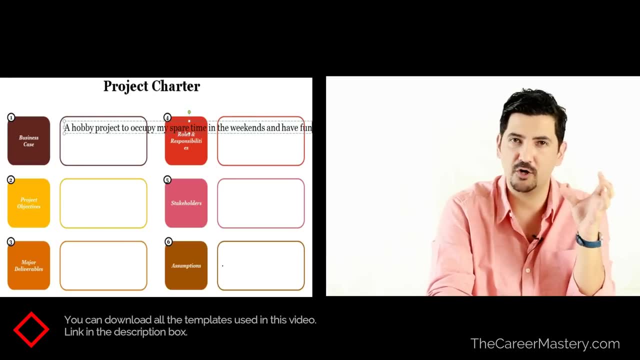 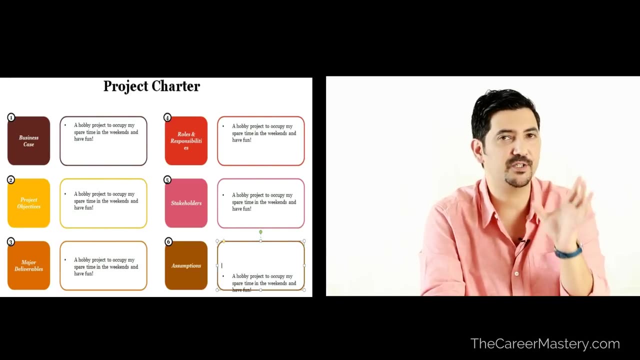 So in my case, if I have to develop a project charter for building this boat, it would include my objectives, scope, rough idea for the cost and time if I want to, and then key stakeholders and key milestones. That's pretty much it. 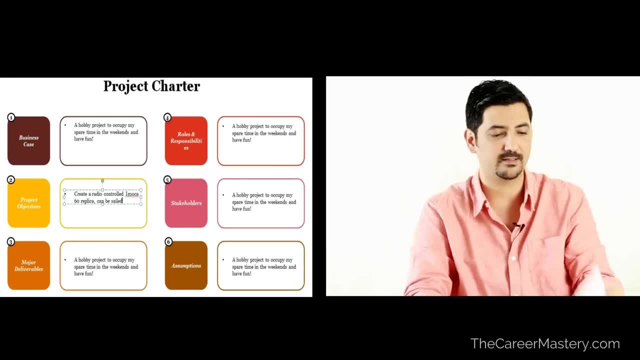 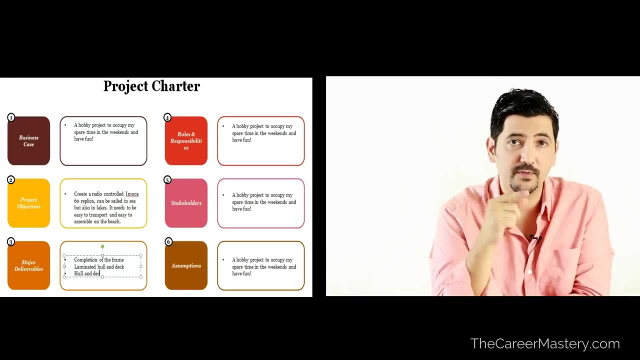 At the initiation stage. you don't want the document to be very detailed. See, this is only like 5-6 slides. it's fairly simple. Speaking of later stages, can you do me a favor if you liked the video so far can? 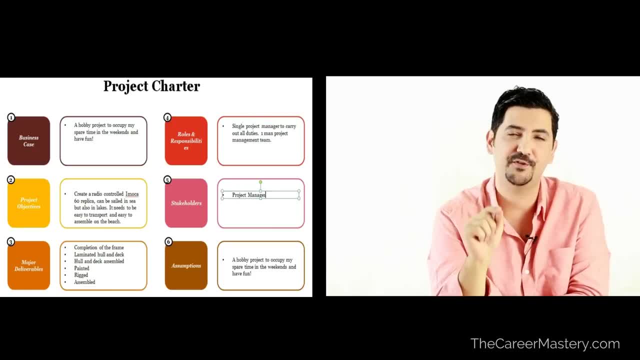 you please subscribe to my channel, Because if you don't, YouTube will not show my future videos to you. So please do that. Let's continue. In your case, Your project charter may be as simple as explaining why you consider the expansion to foreign. 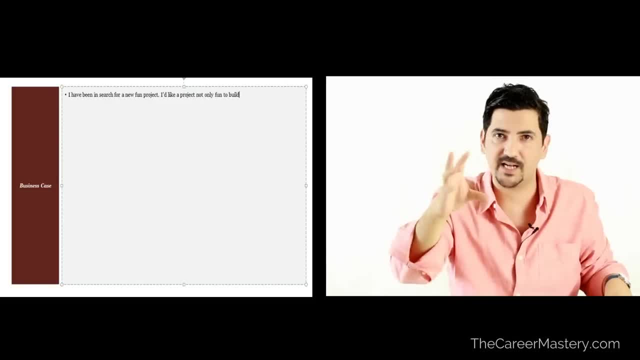 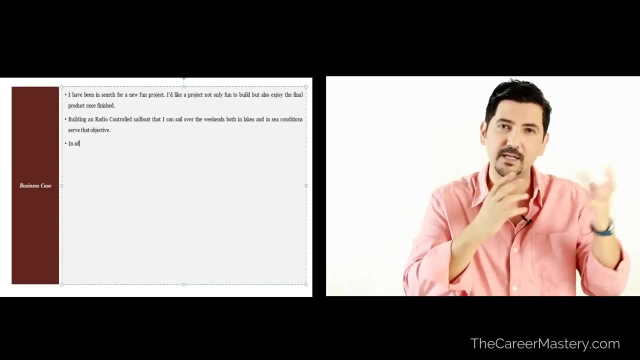 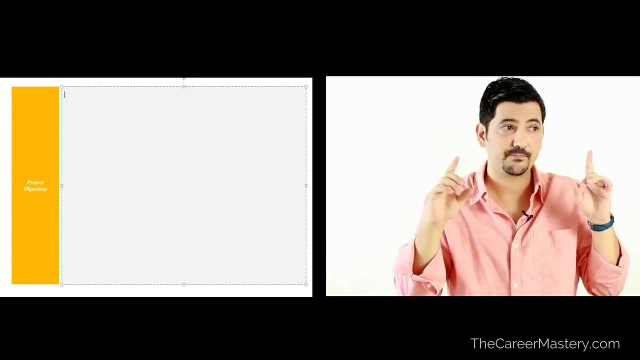 markets, Why you are considering building that new factory. I'll repeat once more: this is not the time to go into huge details. Talk about the business case and maybe high-level project objectives and major deliverables and the roles and responsibilities, But don't go into too much details. 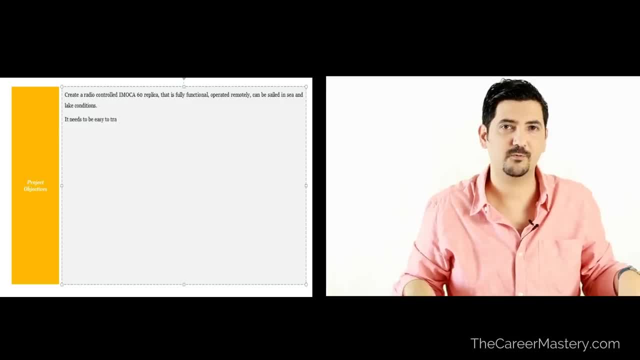 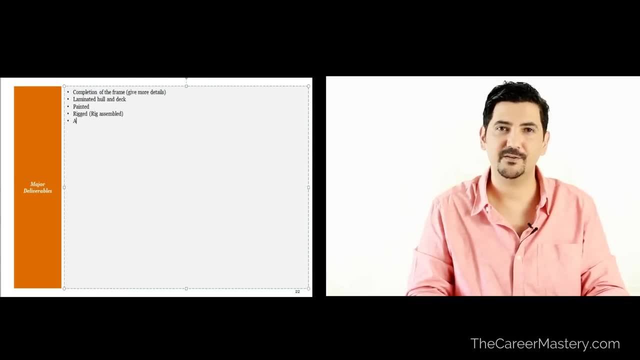 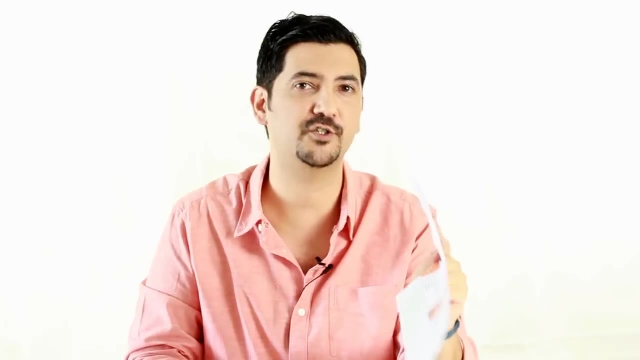 Then you would ask: I mean ok, Then why do you ask, Why do it If it's not detailed nor comprehensive? if it's just a couple pages, why even waste time to prepare it? And if you ask that, it would be a very smart question. 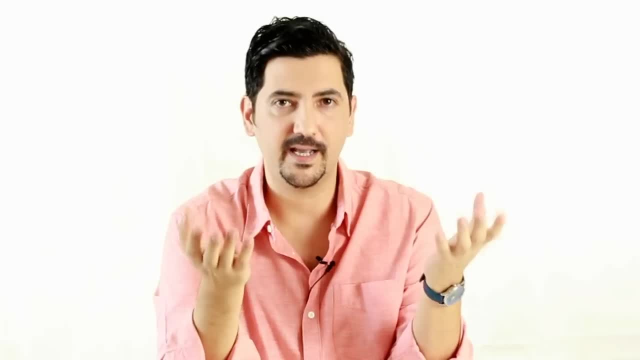 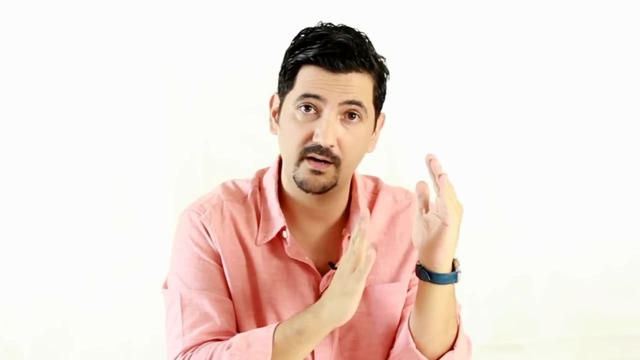 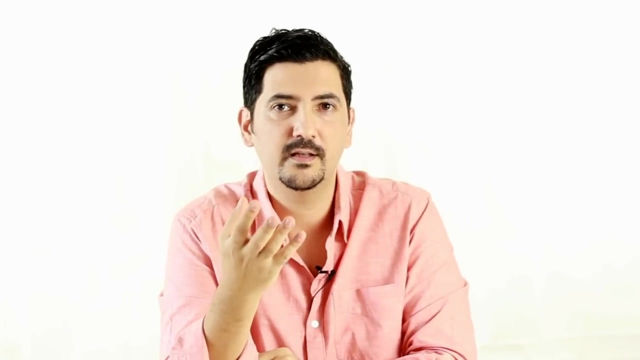 The reason why we do that is to have a buy-in, To have the permission, Because it's a checkpoint. We want the support from the leadership to spend more time and maybe more money to properly plan it. I mean, as a principal, are you my dear project sponsor? are you fine with me exploring? 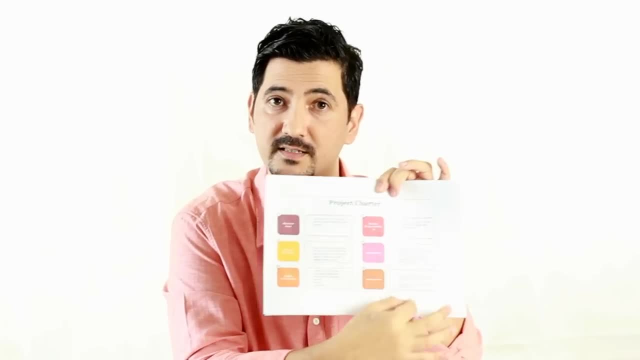 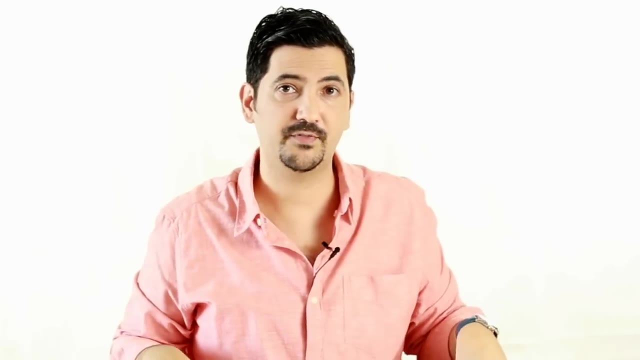 this project a bit more. Can you sign off on this? It's a checkpoint. Your project sponsor may not want this project at all in the first place. Why waste time? If they say no, you don't start planning. And, my friends, planning is no easy task. 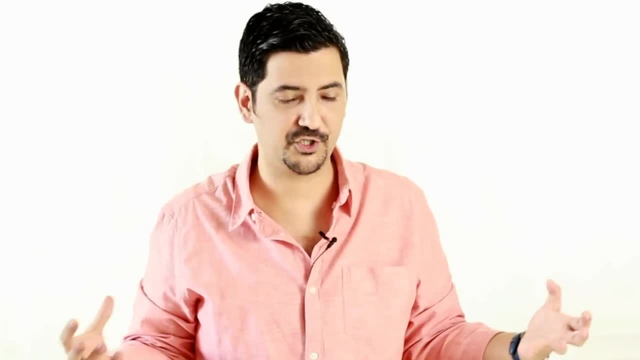 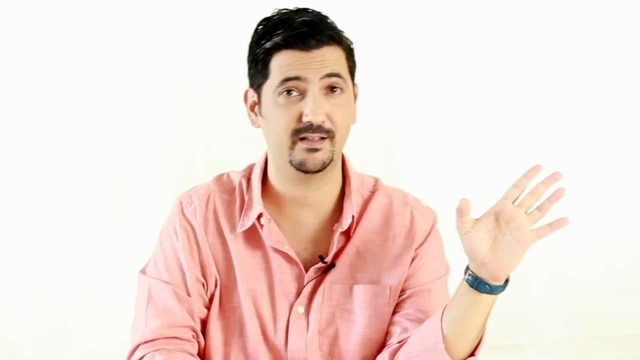 Planning is difficult, So it's a great opportunity. It's a great opportunity for the senior leadership to kill the project early on, before you spend so much time planning it. Maybe they don't want to expand into that market. Maybe they have their own reasons. 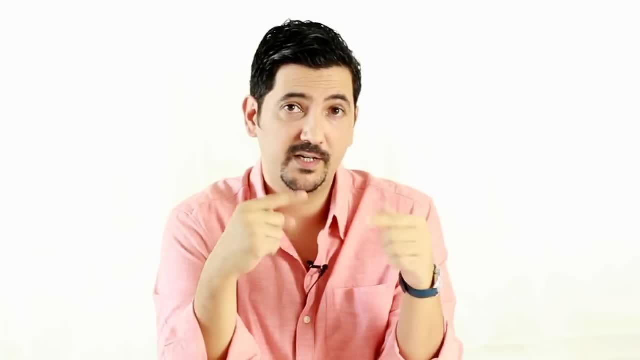 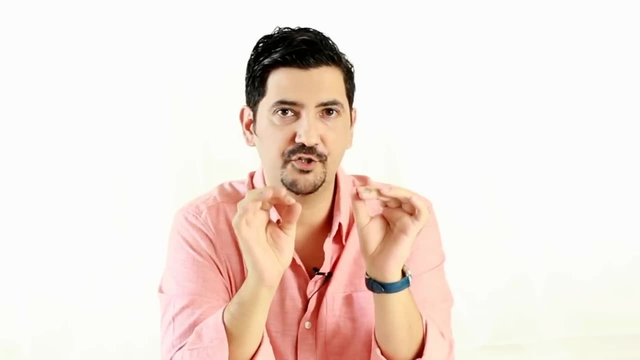 So they kill it off early on. But I want to open a deep note here and contradict myself a little. What you need to do or how much detail that goes into the charter heavily depends on what you do. What you need to do or how much detail that goes into the charter heavily depends on 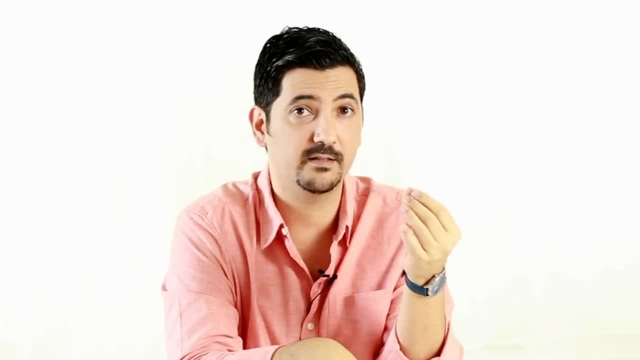 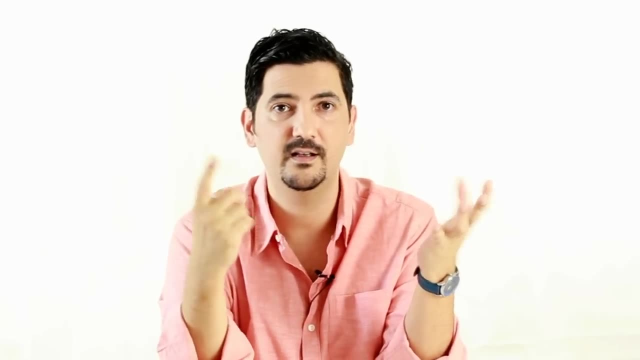 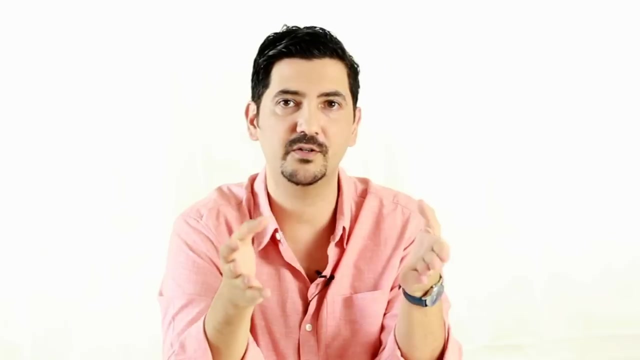 your project needs, project scale, your industry. So if your project is, let's say, creating International Space Station, obviously your initiation will include a lot more details. It'll be almost like high-level planning, And the reason for that is because planning such a project- the International Space Station- 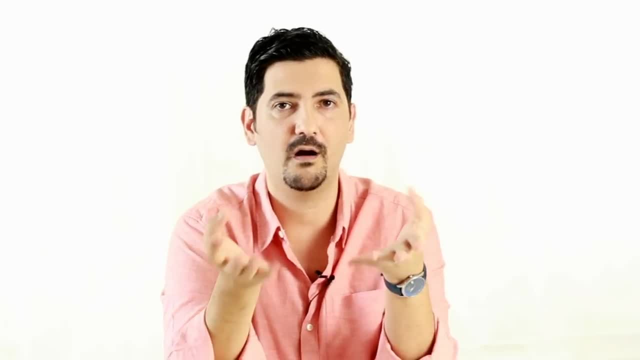 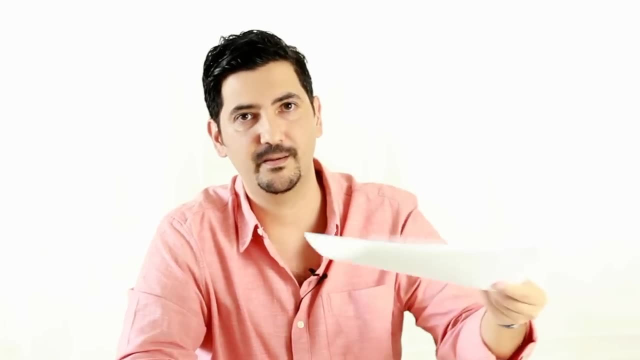 is over 10 billion dollars Just the planning. So obviously it will require you to present a lot more information to your project sponsor to get an approval for a 10 billion dollar planning. So far, so good. Good, Let's move on. 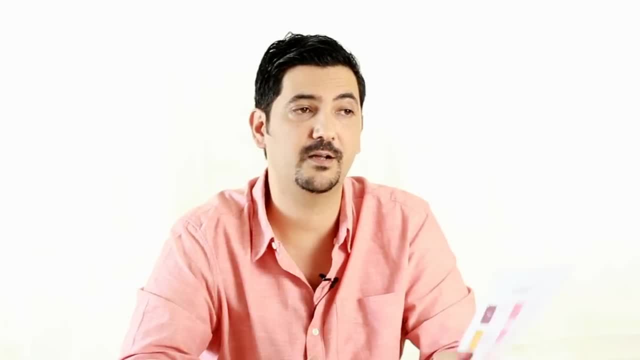 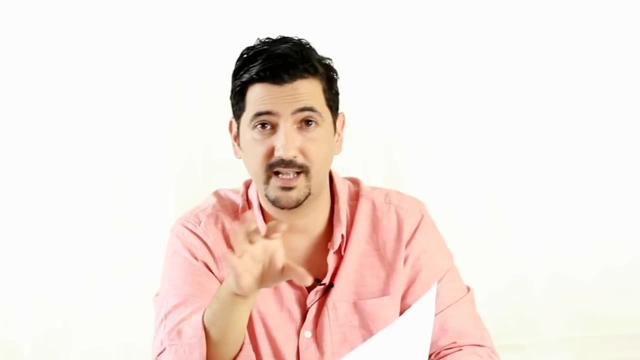 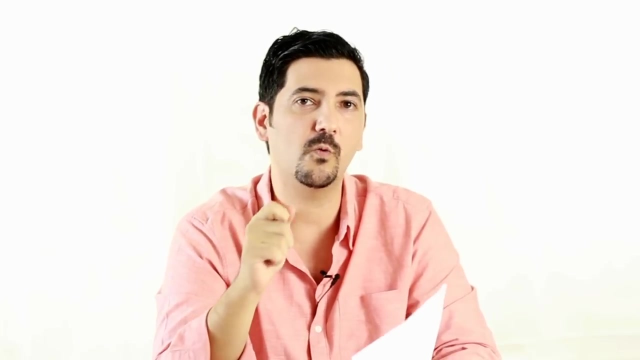 The second process for Initiation Process Group is Stakeholder Identification. At this stage, you will again keep it very simple. You will not categorize all the stakeholders based on their influence and power. You will do that later. Now, as I mentioned before, we just want to know whether we should proceed or not. 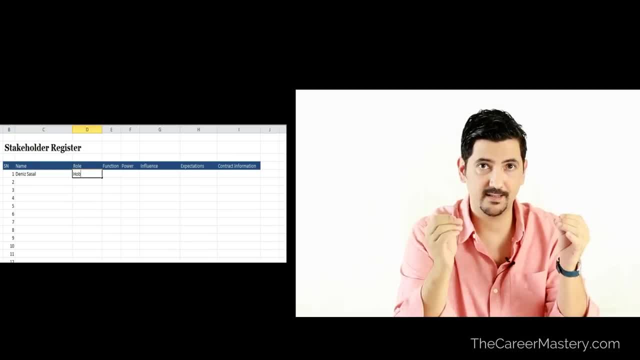 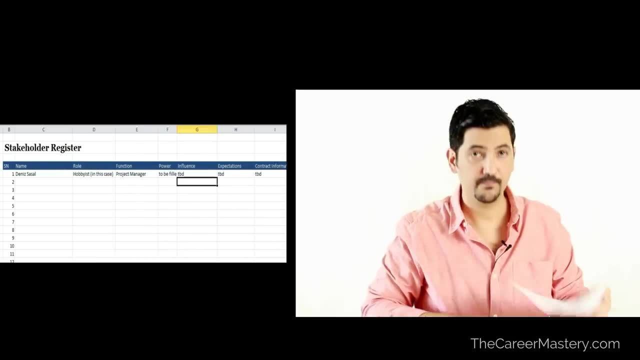 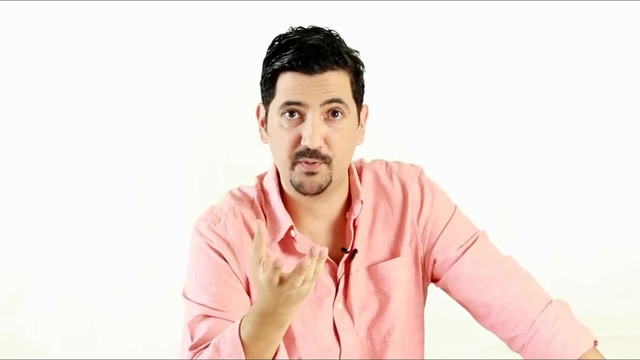 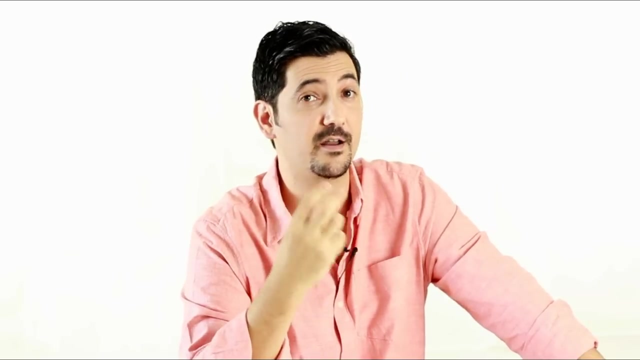 It's a checkpoint. So all you do is create an Excel list and list down all the project stakeholders. So in my case, my stakeholders will be my wife- she'll be my sponsor- then my neighbors, because I'll do a lot of hammering and drilling so I'll make a lot of noise. 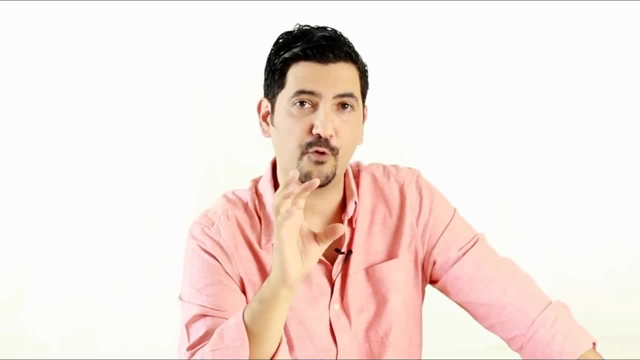 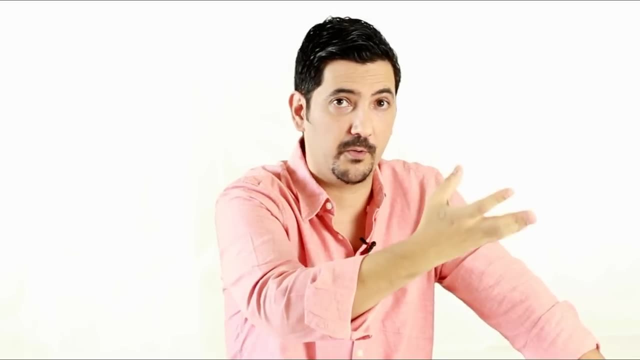 Therefore, I need to include them as my stakeholders as well For most projects. 1. Which stakeholder is your project sponsor? 2. Who is your sponsor? 3. Who gives you the go or no go? 4. 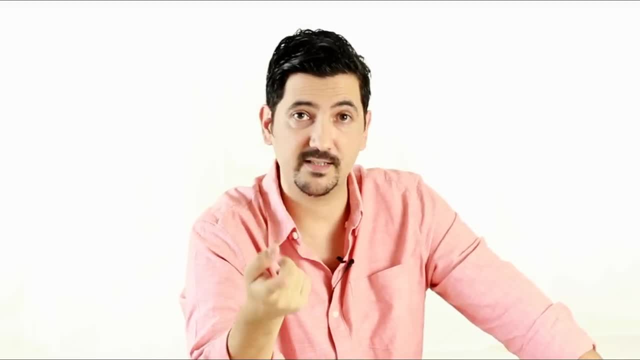 Who is the project manager? 5. Are you the project manager? 6. Who are going to be part of your project team? 7. Who are going to be project management team? 8. Project management team is different than project team. 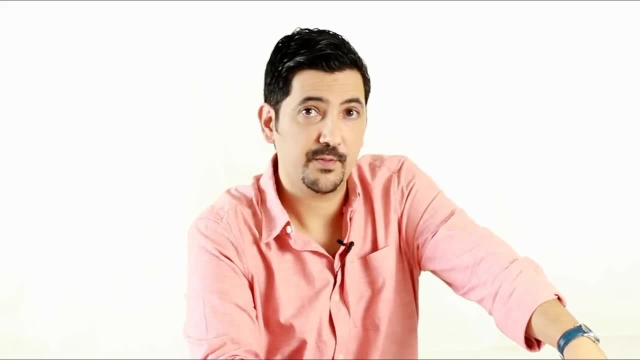 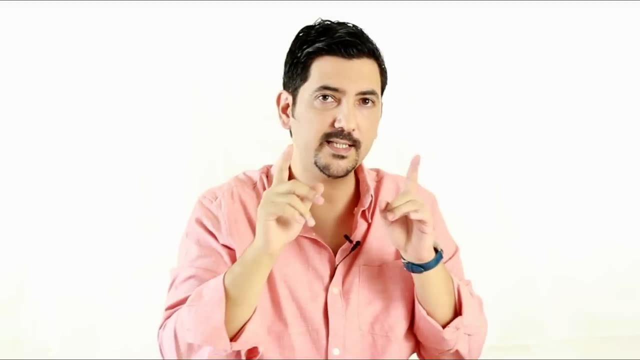 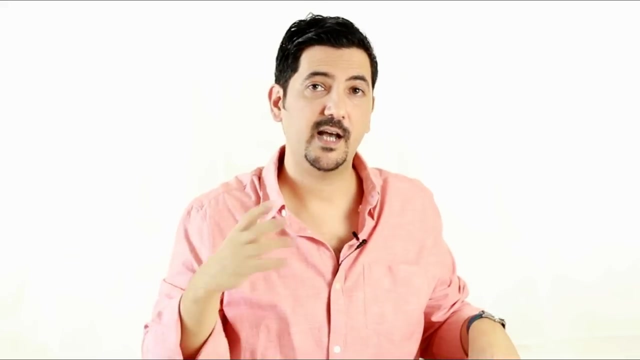 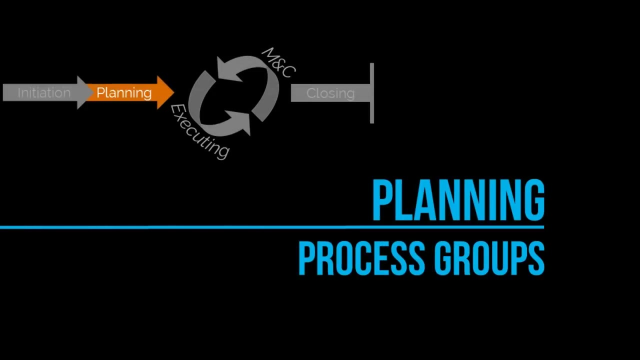 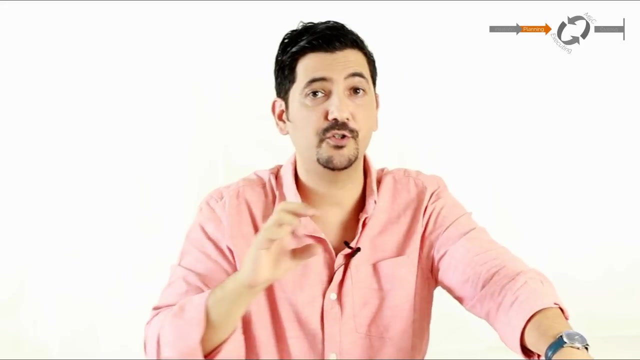 9. Now we have the project charter and the project stakeholder register. it's now time to move on to planning. 10. Planning is a lot more detailed and comprehensive than initiation. We are going to need to talk about a lot of details and knowledge areas. 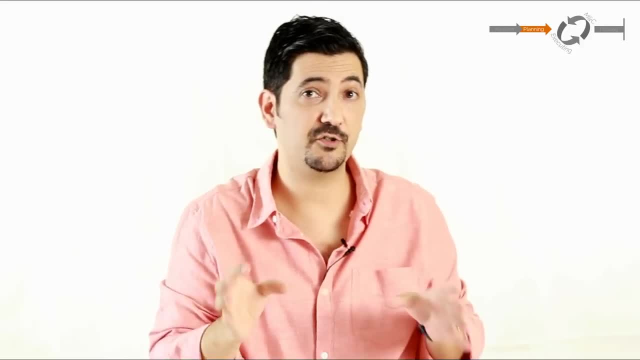 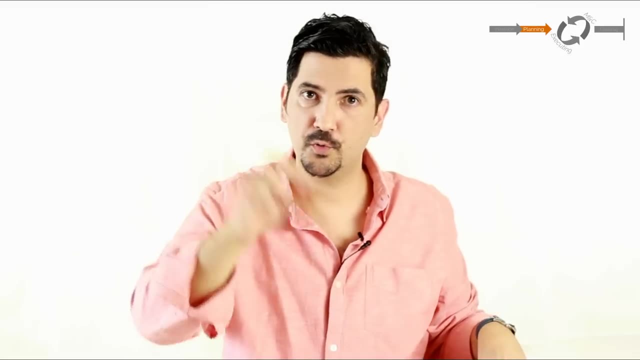 So I am going to introduce you to certain knowledge areas. I suggest you take a break now, Pause the video, Go get a cup of coffee, Refresh yourself and come back when you are ready. Or you can just bookmark this video and watch it whenever you are on top of your focus. 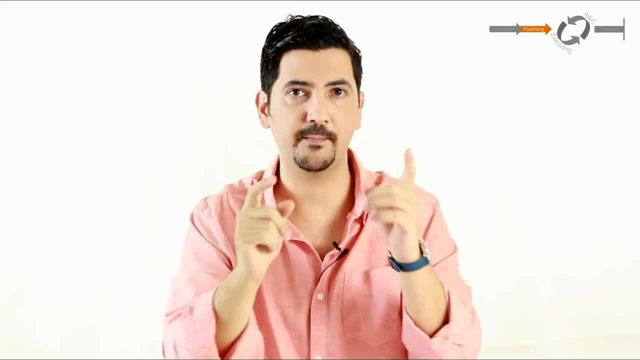 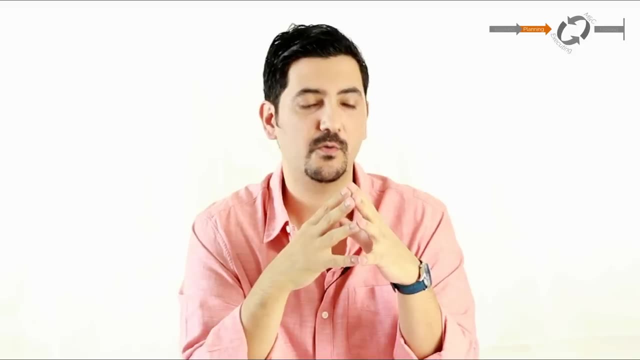 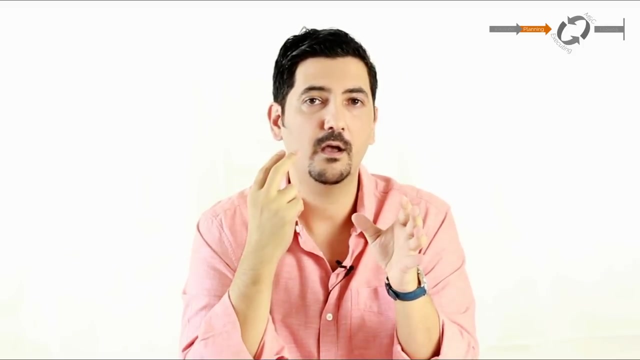 Okay, Let's start So with planning. we are looking to find answers to 3 main questions. The first question is: What are we going to do? How are we going to do it? How to know when the project is done. 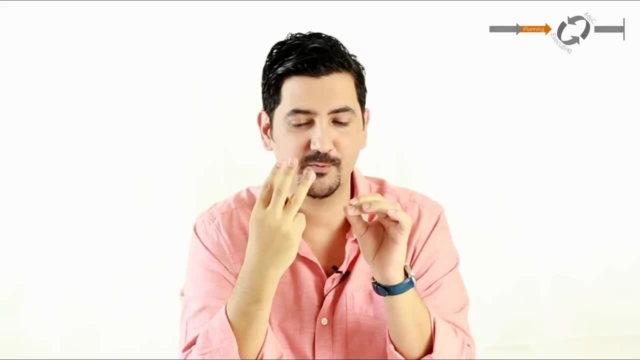 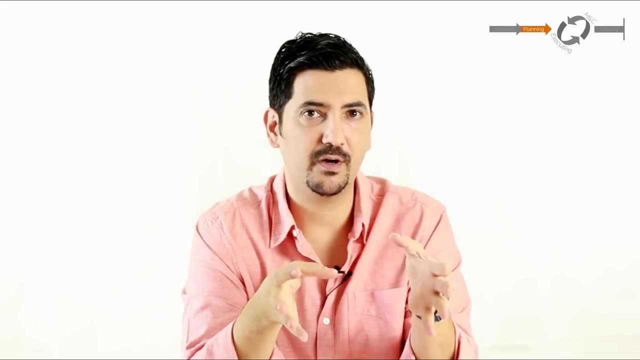 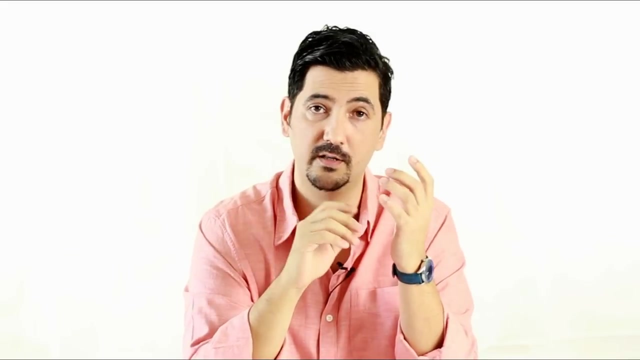 This particular one is very important Because in real life, most projects are never done. At the end of the planning process, you'll end up with a comprehensive project plan, And this project plan will include a few items. It'll include the requirements. 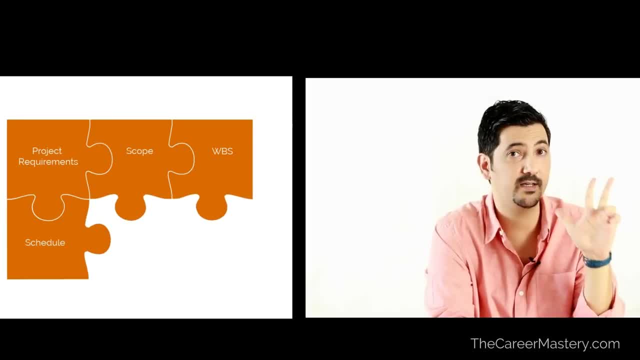 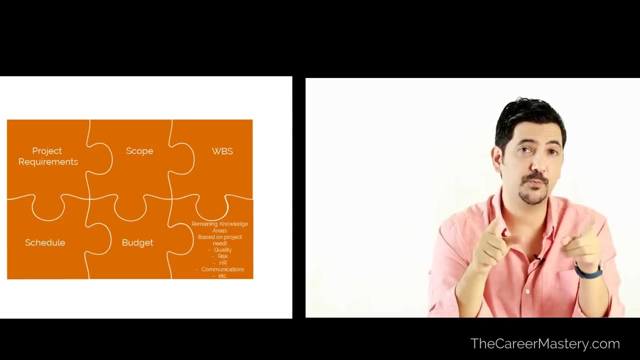 It'll include scope, Work breakdown, structure, or as we call it, WBS Schedule, Schedule, Schedule Schedule, And along with it you'll have a MTA. Then we'll have cost… Budget… network And quality… So Let me put a disclaimer here. 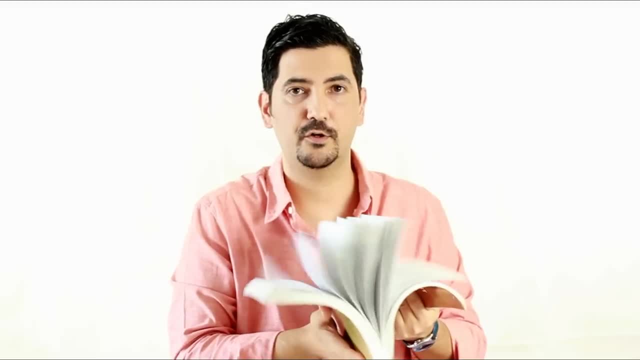 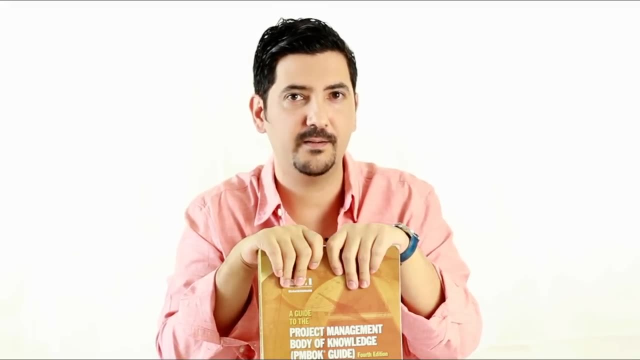 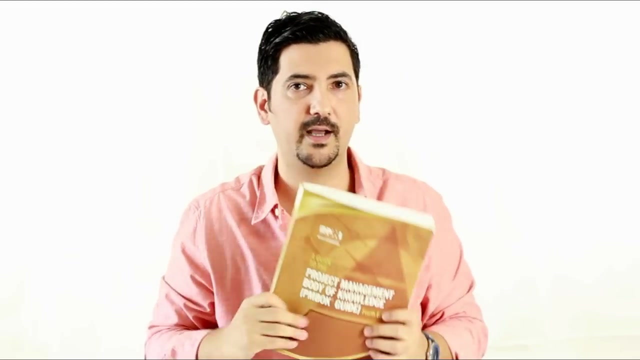 The PMBOK guide is 500 pages of glory. It has obviously a lot more knowledge area, But I'm simplifying things and for you here. So if you plan on taking the PMP test, just make sure you properly read this whole thing. 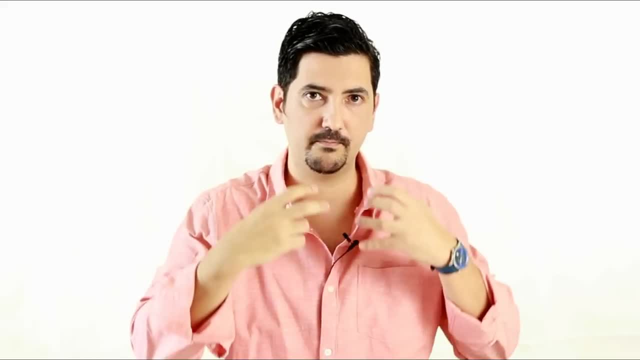 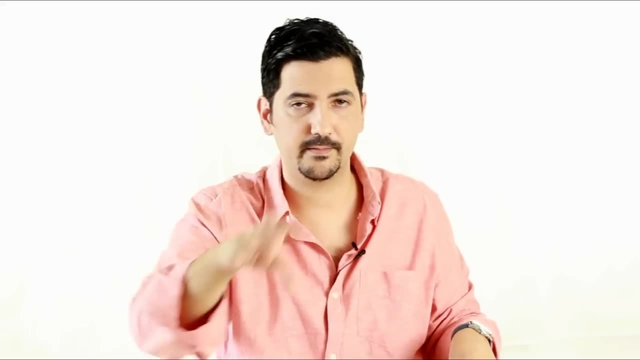 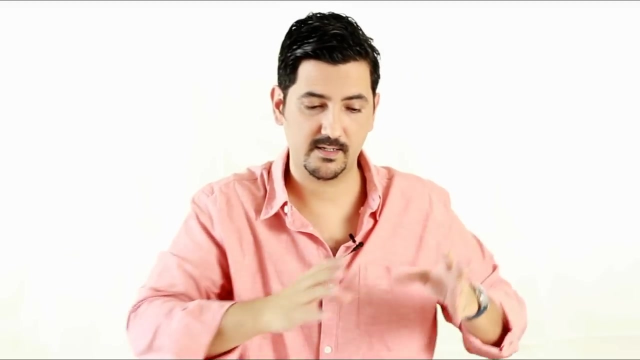 okay, All I am trying to do is simplifying things and make you understand the fundamentals, so when you read this, you'll be able to understand it very clearly. But just keep this in mind: I am leaving a few things out, Because this video isn't only for PMP takers, but for anyone who just wants to learn the 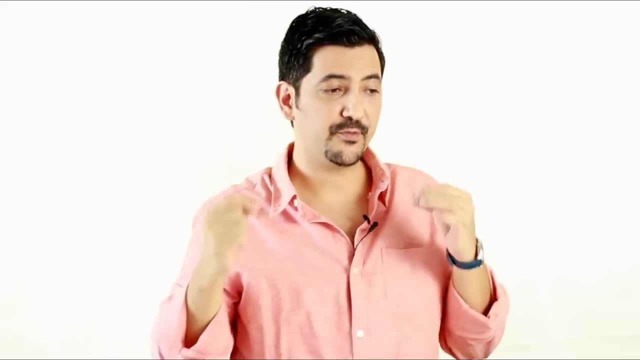 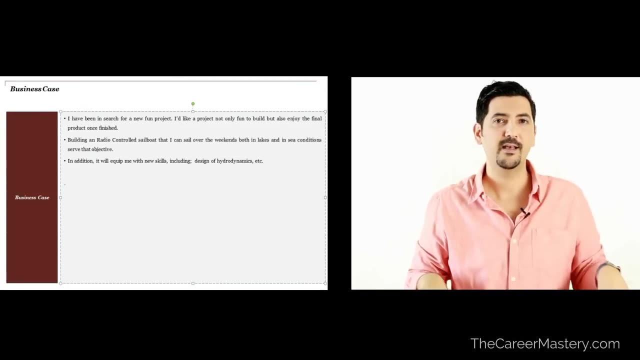 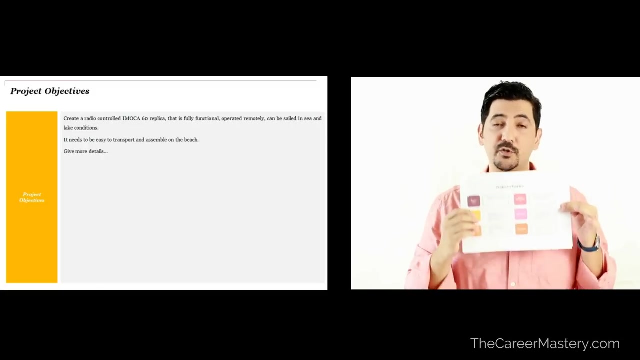 fundamentals of project management. Good, so let's get going. The first process we have is collecting requirements, Understanding what stakeholders want. What do they really want? I mean, we wrote this in the project charter, right? So what we are going to do is we'll just take this project charter and give it more details. 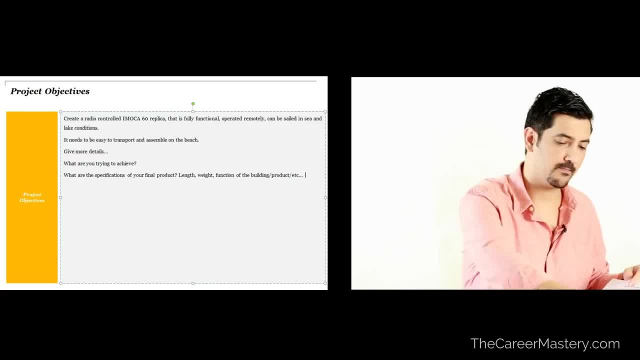 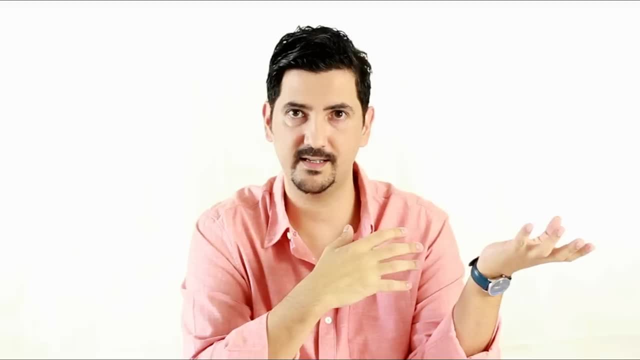 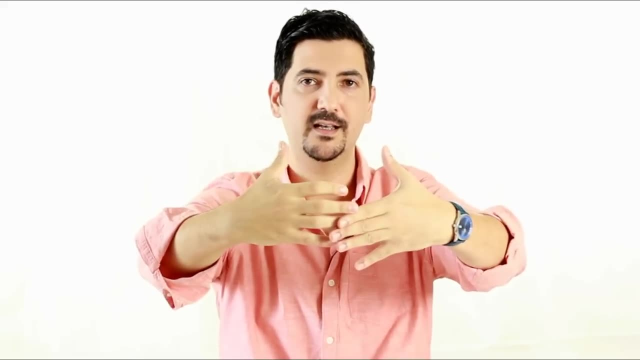 and specifications Right, And then it will become this. See, this isn't a very easy task in real life. I mean, collecting requirements supposedly is the easiest part, but the difficult part is maintaining your sanity, Because the moment you start gathering requirements, then everybody is going to want to know what. 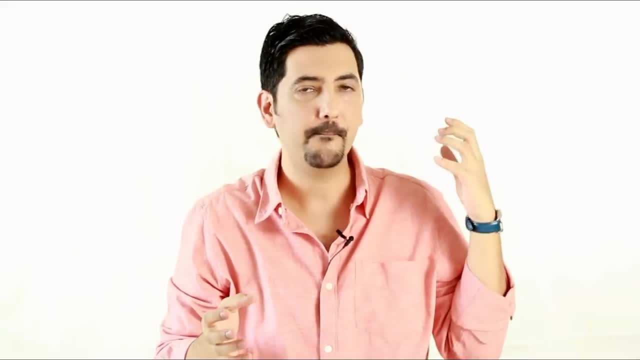 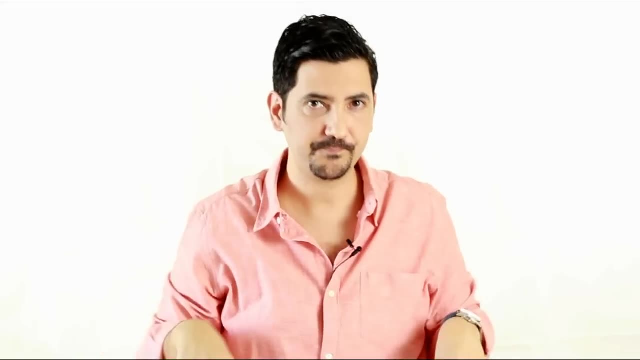 they want to have the best of everything, without consideration for budget, quality or schedule, And they'll have contradicting requirements within themselves. There'll be clashes And, especially at this stage, you don't even know the budget or the quality or scheduling. 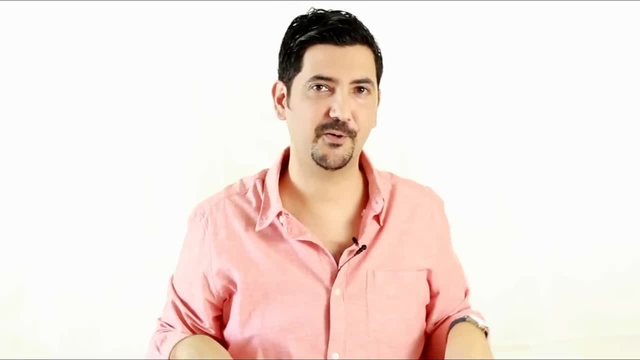 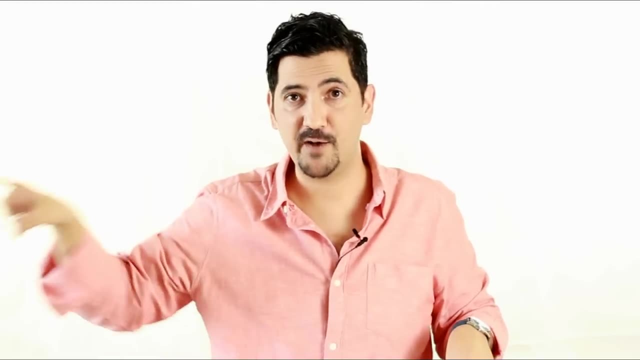 I mean, you have a rough idea but you don't know the details. So you kind of gather the requirements based on your assumptions. And that's no easy task. If my wife comes up to me and says, hey, let's buy you a new car. 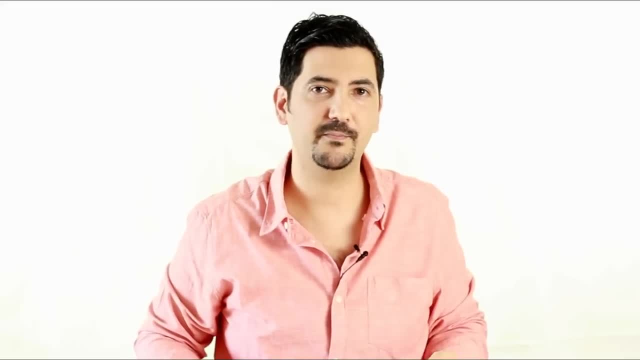 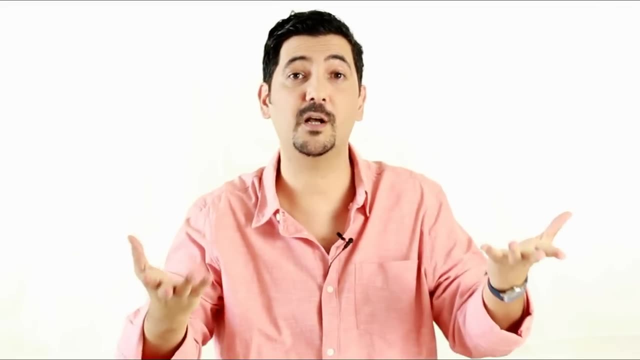 It's time She asks: what car do you want? I'm going to say I want Porsche 911 GT3.. I won't consider the family budget or the maintenance expenses. I'll just say what I want. That's how it's in project management as well. 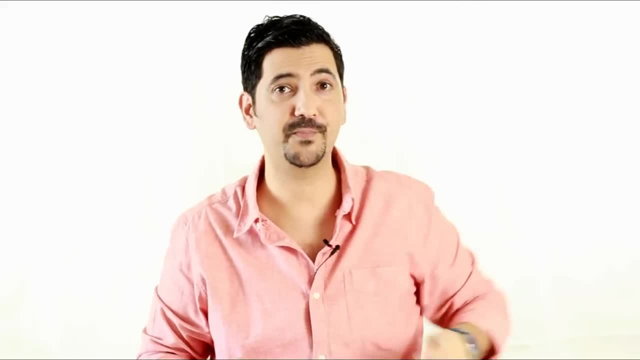 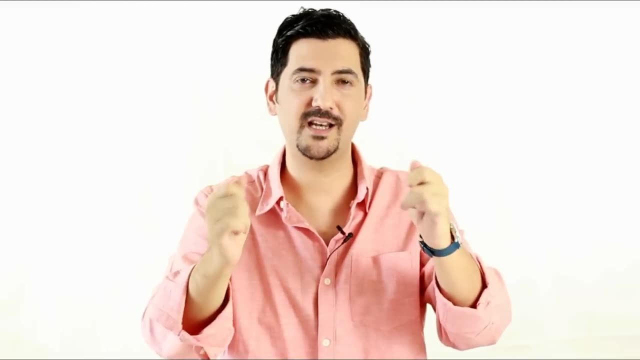 When you ask what your stakeholders want, they'll shoot for the moon. They'll want the best. So as a project manager, you have to keep things on the leash and explain people that there are always trade-offs in life. Just a small tip. 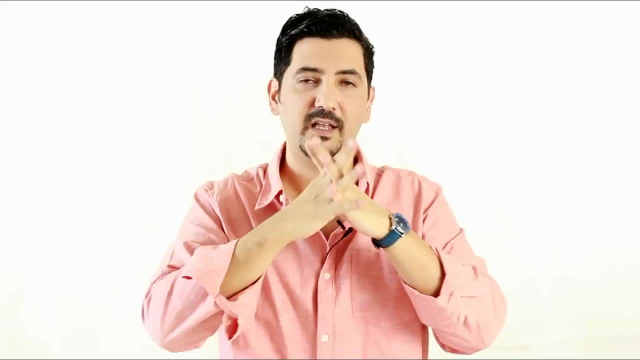 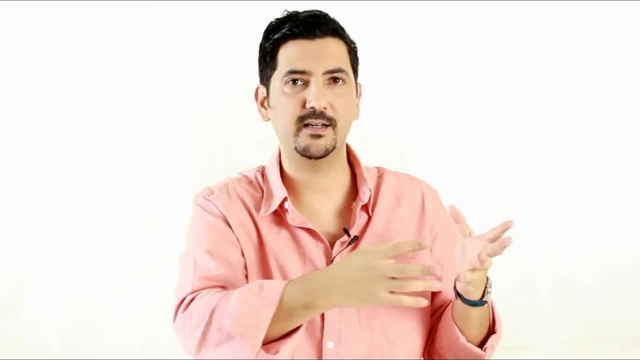 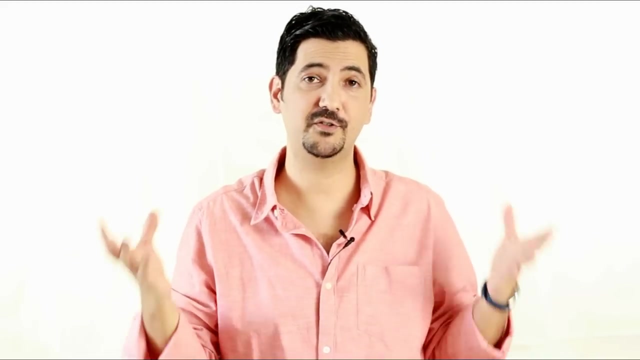 When you are collecting requirements. there are so many methods available to you. You can do one-on-one interviews, you can apply Delphi technique, you can do nominal group technique or other methods, all those fancy sounding names. But if you ask me, and if you can just stick to the good old meeting, 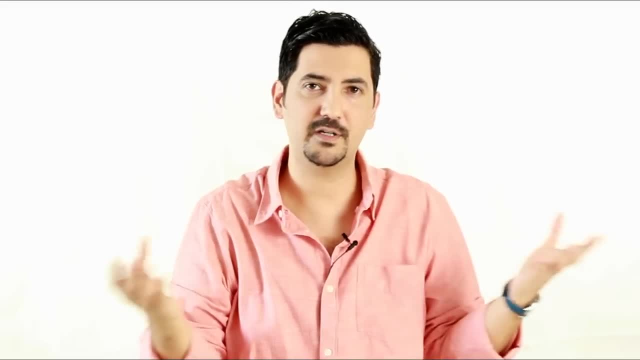 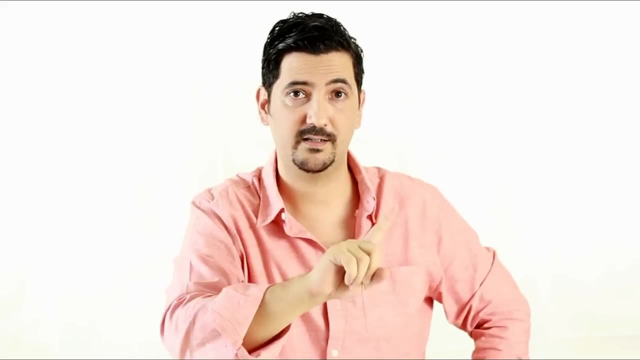 Just get everyone in a room or in a teleconference and gather the requirements collectively. If you do interviews one by one, then you'll have a lot of contradicting requirements that you have to deal with. Get everyone together, let them argue, let them fight. 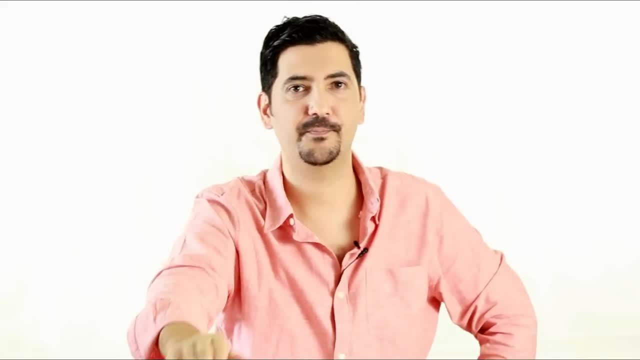 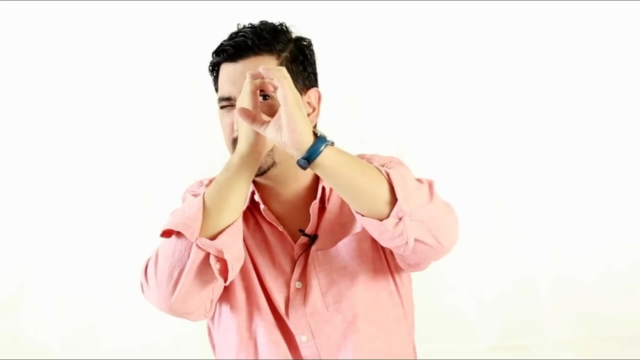 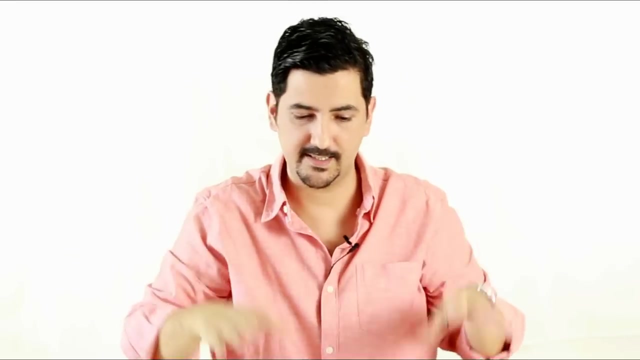 But at the end you'll have your requirements set in stone. Next process is defining the scope. Like this: It's the scope. What does the scope do? Scope makes you see certain things clearer, but then exclude other things. right. That's exactly what it is in project management as well. 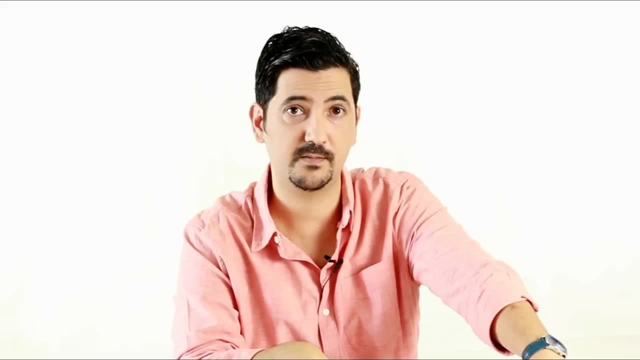 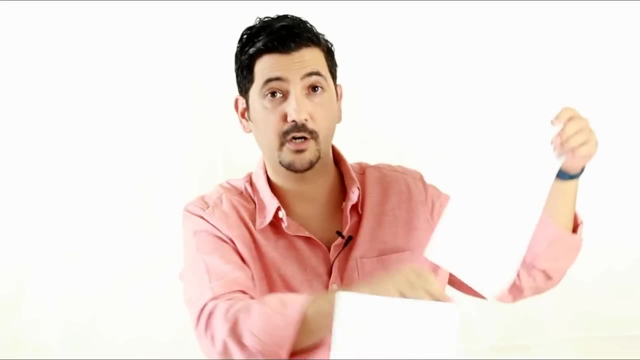 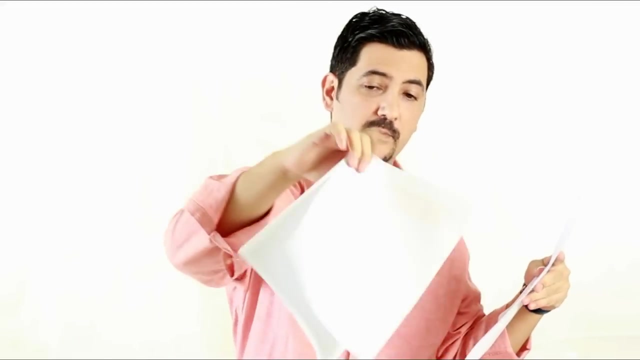 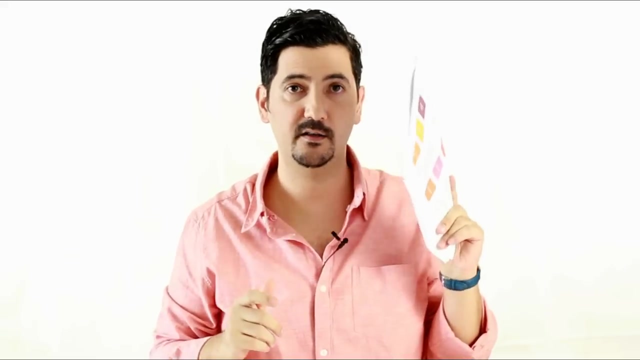 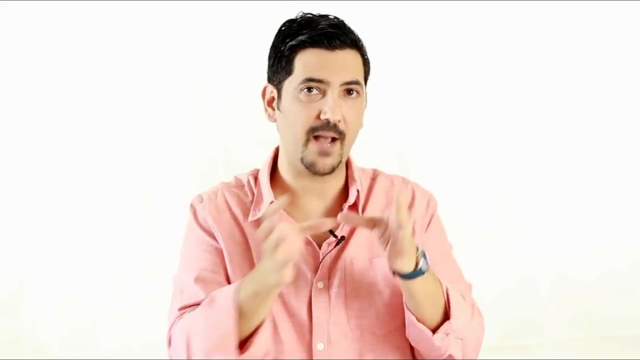 So to do our scope, we need a few documents. We need the project charter and then we need the project requirements document and then any risk, assumptions and constraints, whatever you have. that will all help you define the scope. Now, defining the scope is one of the most important processes, because what happens in 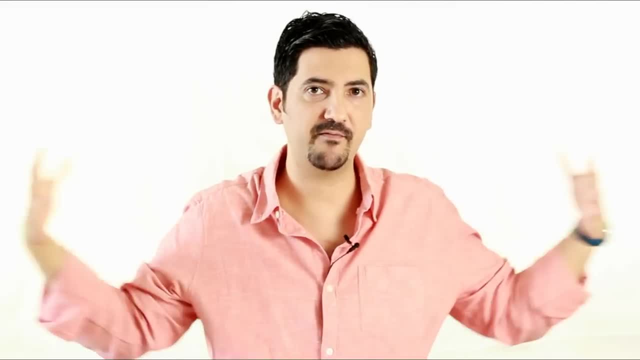 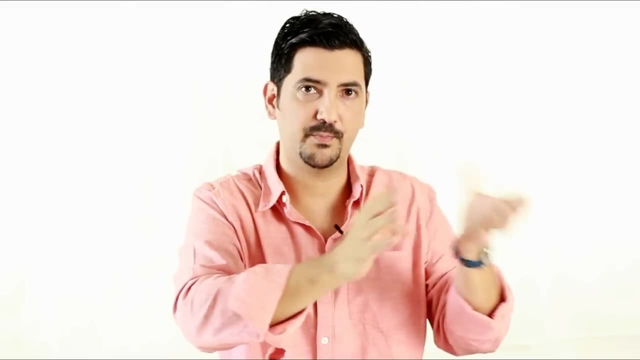 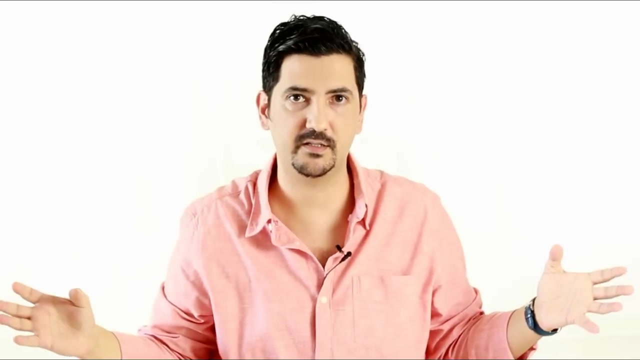 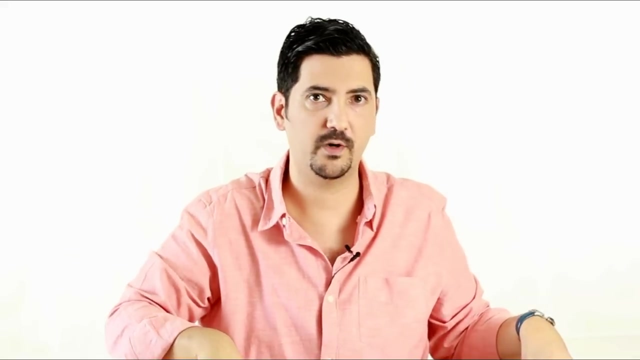 reality is Weak project managers include everything in the project requirements document Or make it very vague also in the project scope. So as a result, your project plan just becomes an impossible plan to execute Because your scope goes into your project plan. So if you do a weak job with setting your scope or if you are really vague, then you 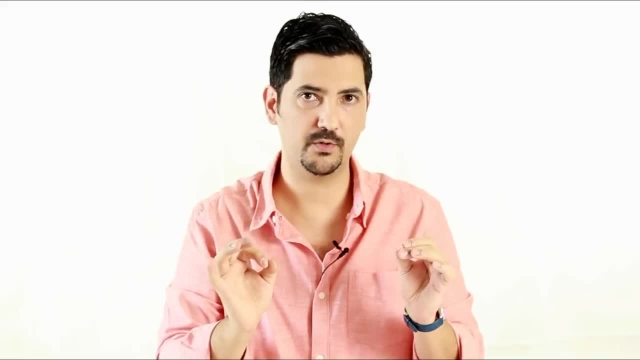 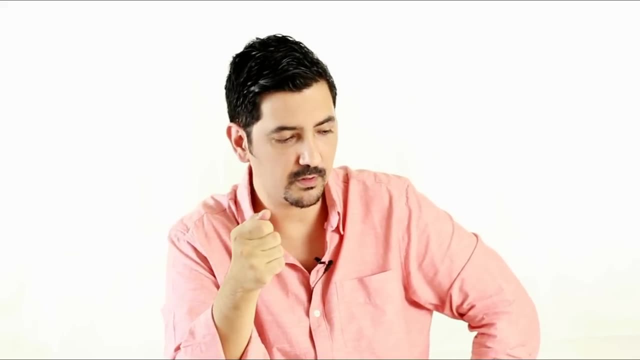 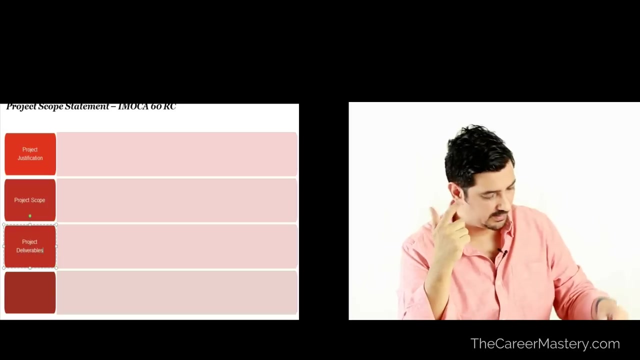 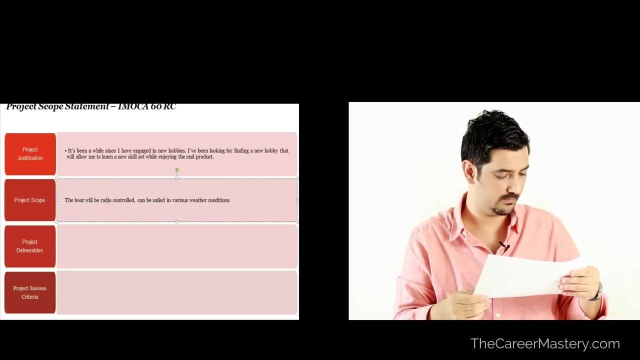 are not going to be able to execute it. Try not to go overboard. Make things very clear. So your project scope statement should or may include your project scope and then your deliverables, your project justification, your business case and success criteria. 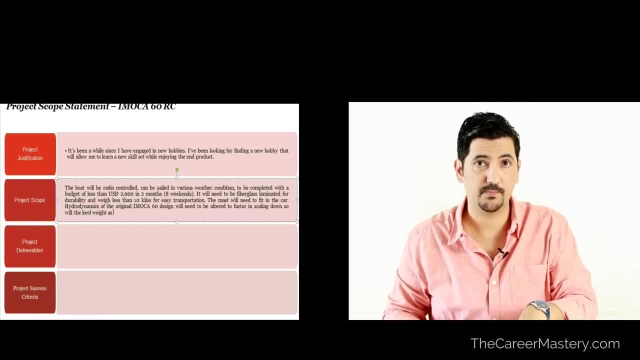 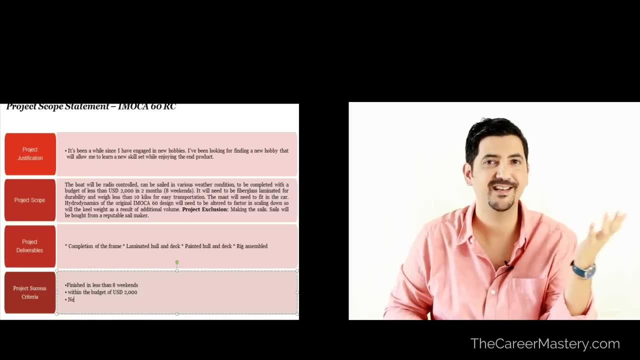 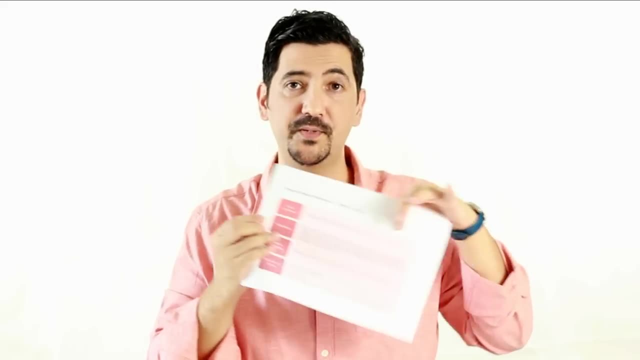 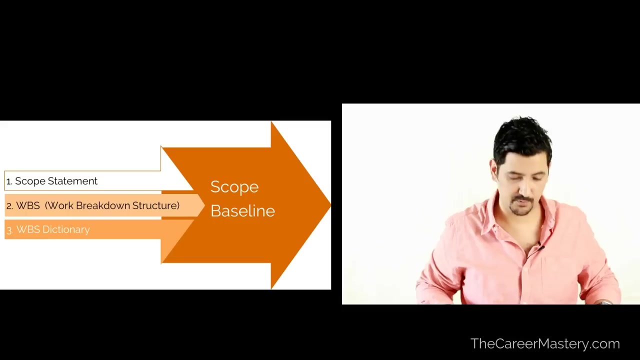 Right. So after the project scope, let me introduce you to a concept called Scope Baseline. Scope Baseline is composed of three things. So you have your scope statement, then we need work breakdown structure. I'll refer to it as WS from now on. 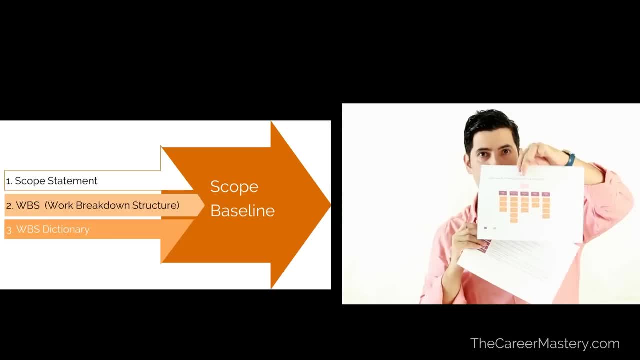 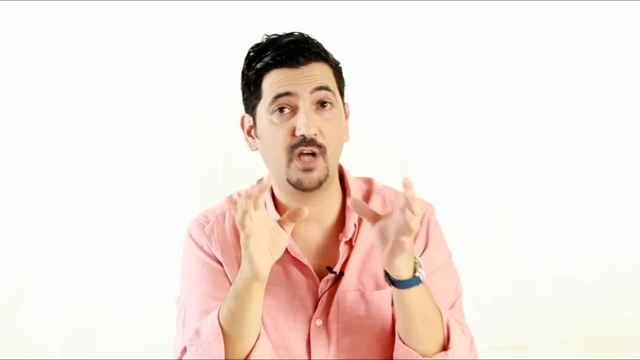 Okay, this is your WS. We're going to do that now, And after that we're going to need WBS dictionary, and again, we're going to talk about that soon. So let's move on with WBS. Now I want to stop you for a second and make an announcement here. 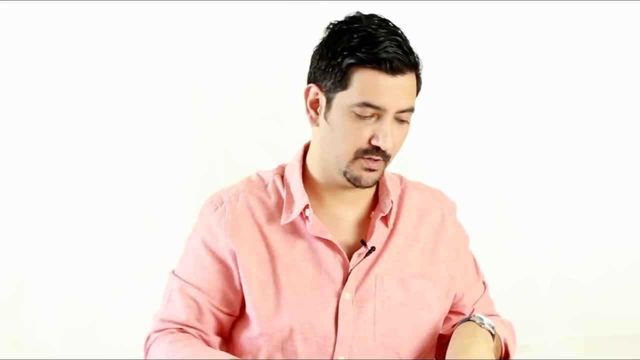 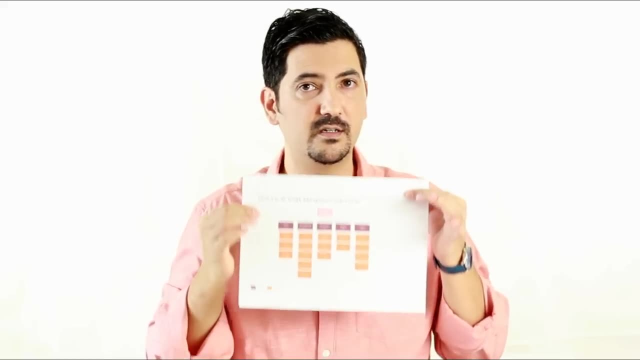 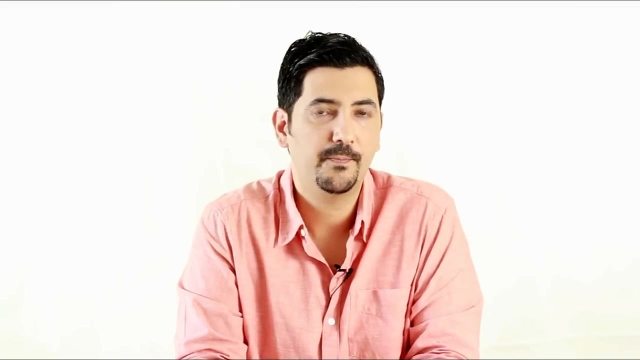 You can't afford to misunderstand WBS. It is very important. Whatever project management methodology or framework you use, this is essential. Okay, So if you want to again, feel free to take another break, go get some fresh air and come. 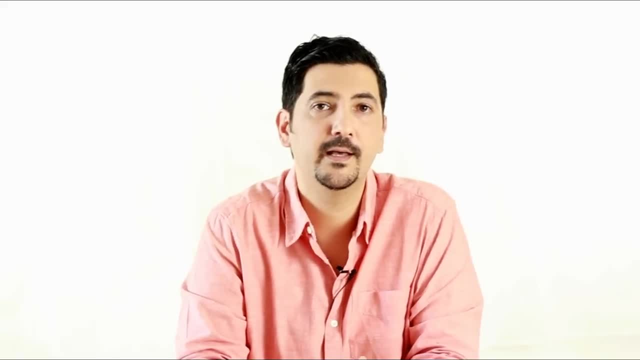 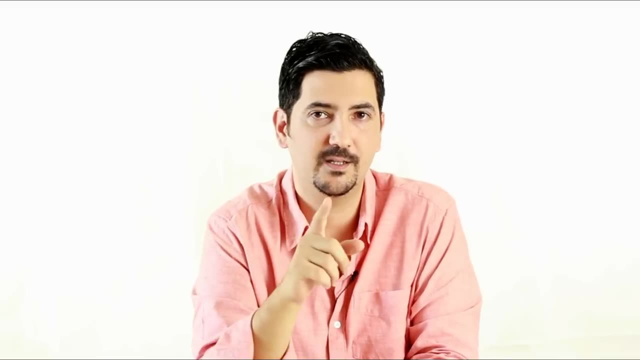 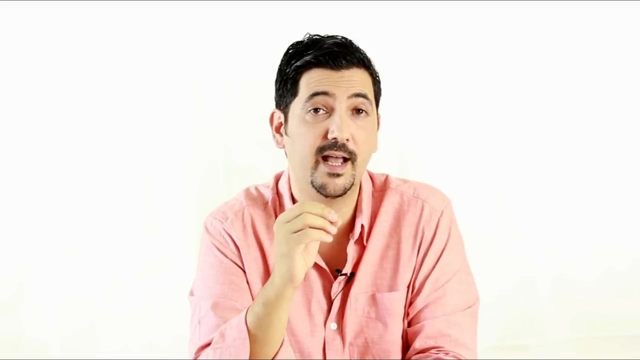 back when you're ready. Good, Before I start creating a WBS for the boat project, let me tell you what it is. The WBS breaks the project down into smaller and more manageable pieces. It's a top-down project. It's a top-down project. 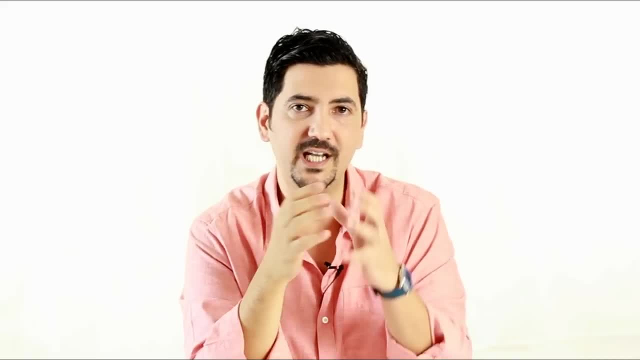 It is a very simple project. It's pretty simple. You can use WBS as a template to create your own WBS project. It's a very simple project that you can use to create a WBS project. It's a very simple project. 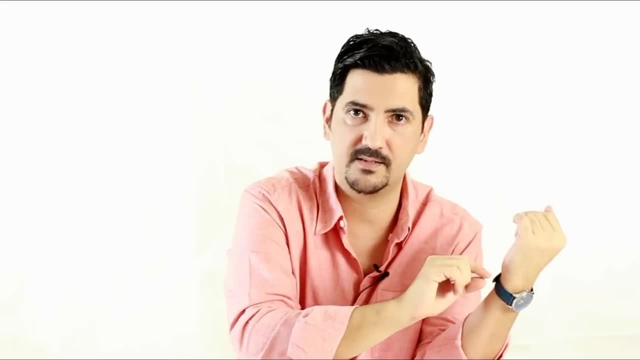 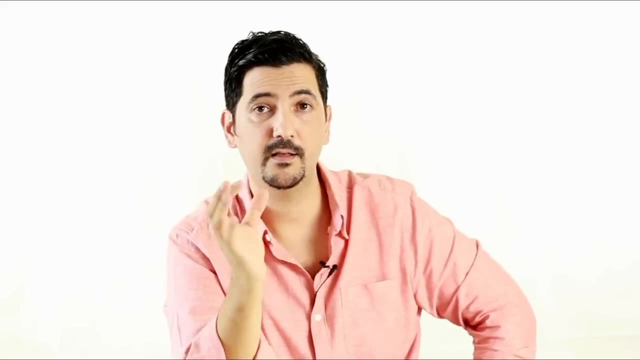 You don't need any effort, Right? You basically just decompose your deliverables And then we call them work packages. Now I want to highlight one more important thing here: If you're strictly following PMI's framework, then work packages have to be things. 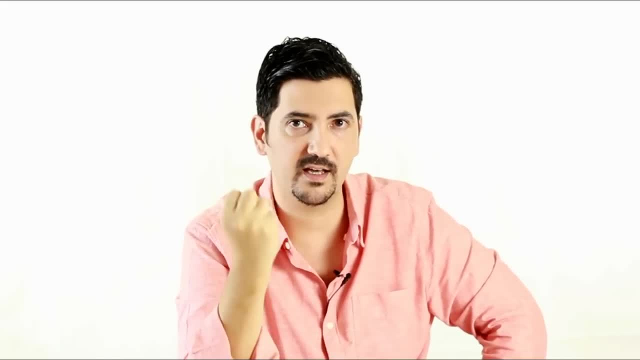 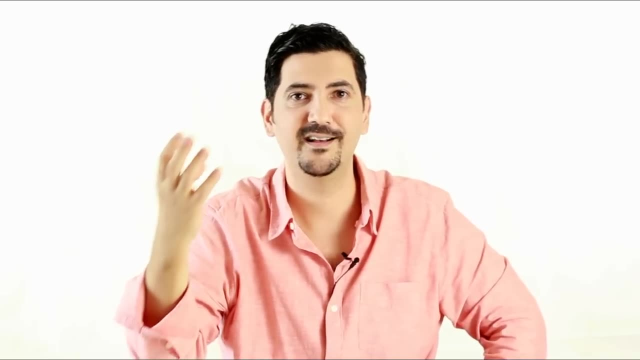 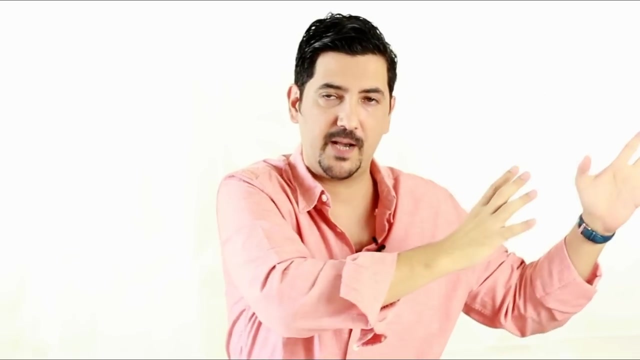 They can't be actions, They need to be deliverables, Things. They can be documents, or building or things. My vocabulary is failing me here. So in practice, though, the things is for PMI but for everyone else, you can do a hybrid. 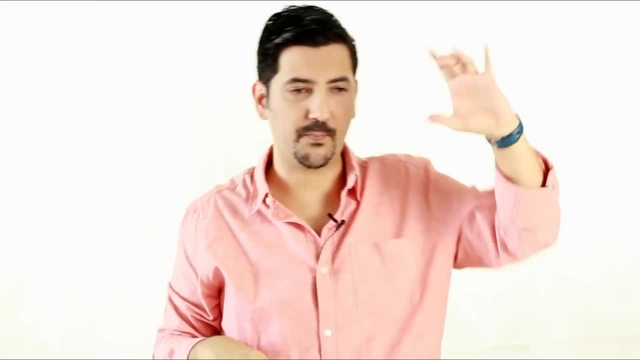 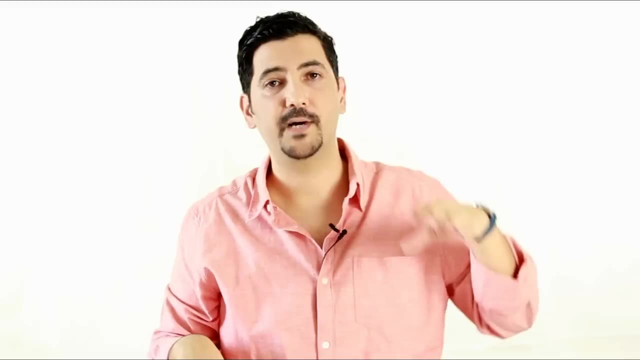 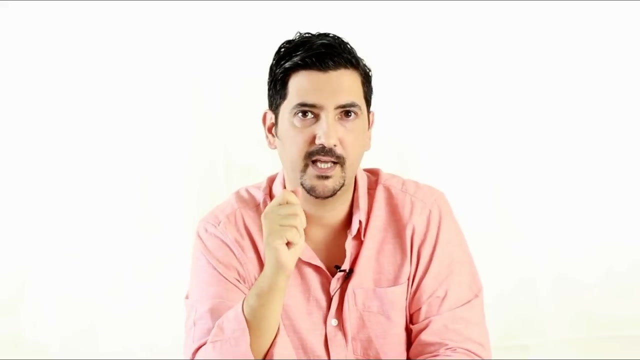 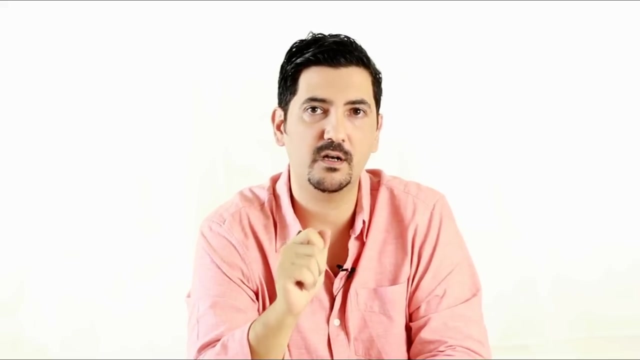 model. It can be work packages and then activities and anything, So whatever suits your need, Ok, so how deep you go, I mean how many layers you want to go? Here is the question. Can you answer this question? Can you confidently estimate the cost and time requirements of that work package? 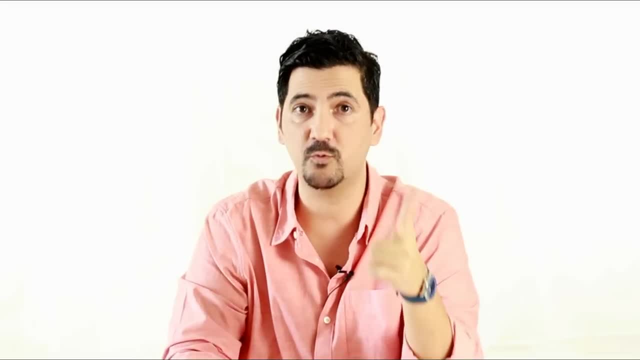 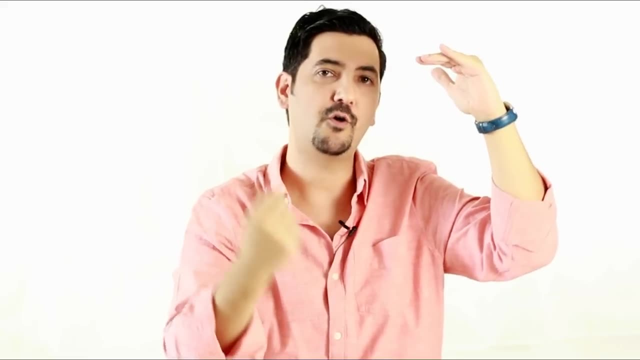 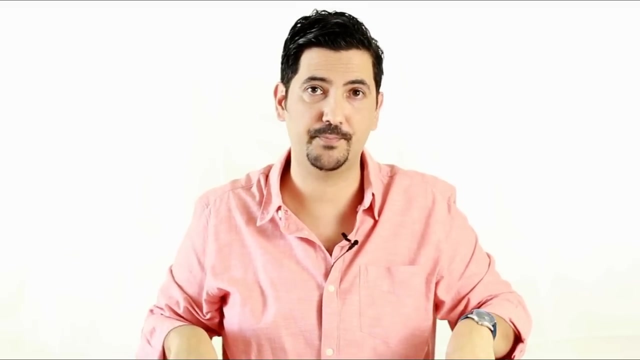 Can you say it'll take 1 week or 1000 dollars? Can you answer that question? If you can't, then you need to break it down further to activity level until you can make some cost and time assumptions. For example, when I look at this boat, I can't say how long it will take me to finish it. 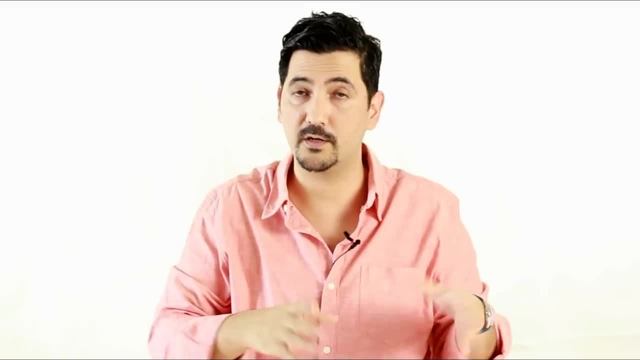 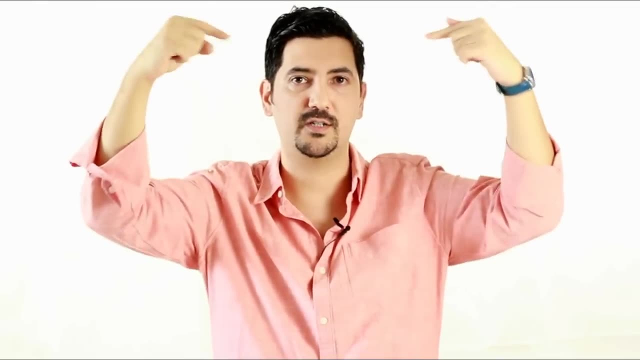 But I can estimate how long it will take to laminate it, or do the woodwork, or do the frames. So go as deep as you need to go, and then you are going to roll up and estimate the cost and time. But that's for later. 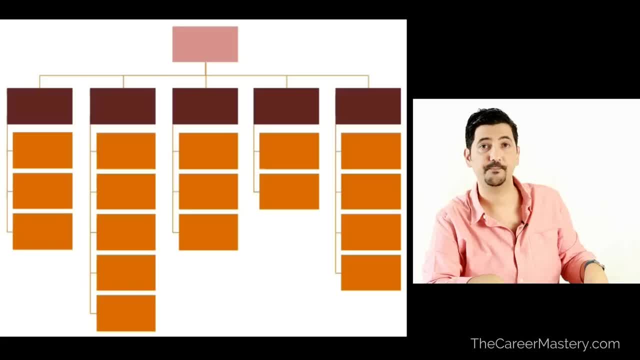 So let's do it, Let's do the WBS. So you start with the project name as level 1. And then you segment your project into various work components. So in my case, my segments are: I have design, I have manufacturing, I have electronics. 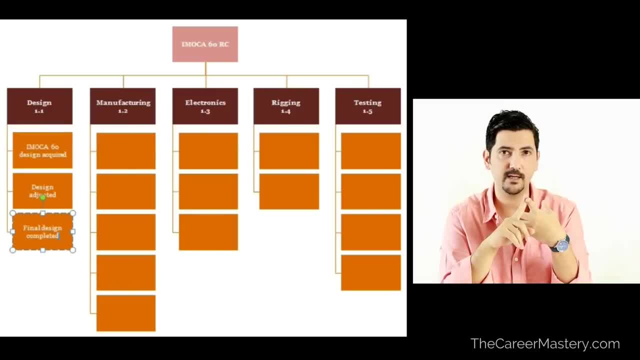 and I have work. Then I have the rigging. rigging is the mast, sails and shrouds and the whole thing, And then I have testing. So then we need to put labels on them: 1.1,, 1.2,, 1.3.. 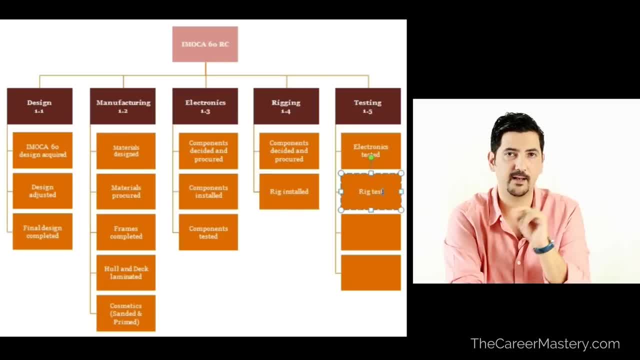 Now this is still too high level, right When I look at the graph at that stage, can I estimate the cost and schedule? No, Probably not. This means I am going to break it down further Now. for this project, a project this small, I don't need sub-segments. 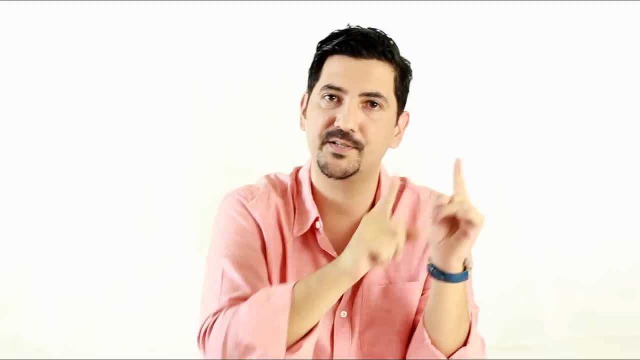 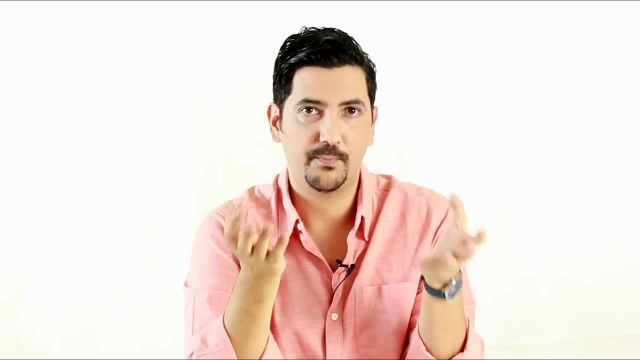 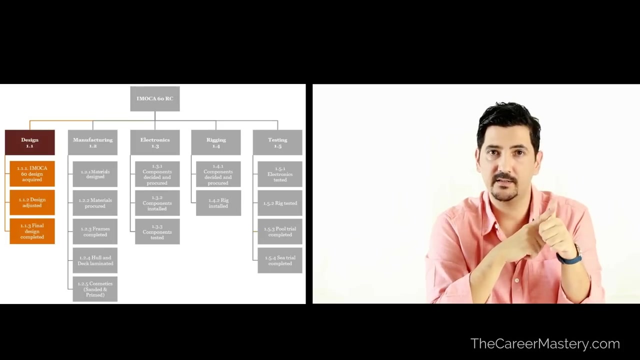 But keep in mind that in your project you may need to put in sub-segments to break it down even more clearly. Now let me start attaching my work packages. These are the important bits My work packages are. So I need to find an actual IMOCA 60 design. 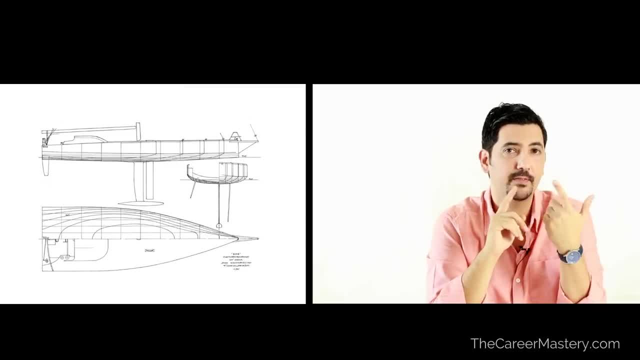 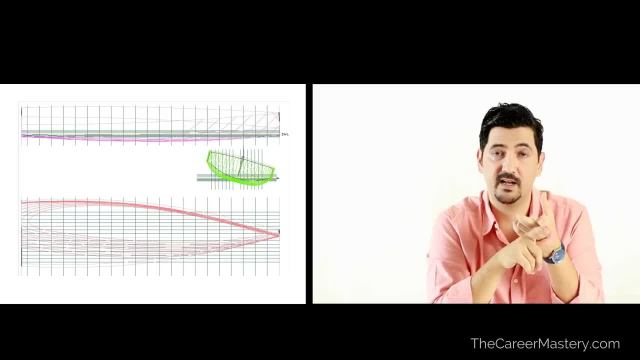 partiron: 0.. Kelowna responses: 0.. Continue to line it up till same value as 0.. And then at this point, What else? After that, I need to adjust the design for scaling down, Because you can't just take a design for 20 meter boat and then manufacture a 1.5. 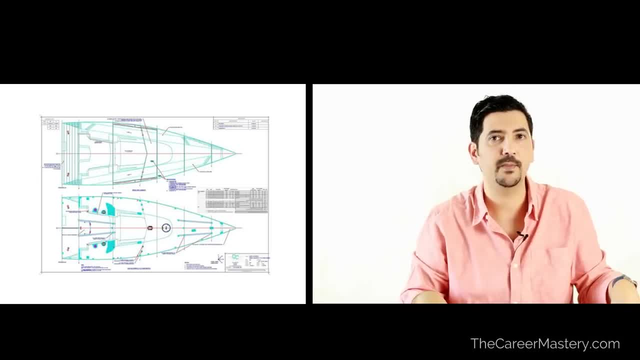 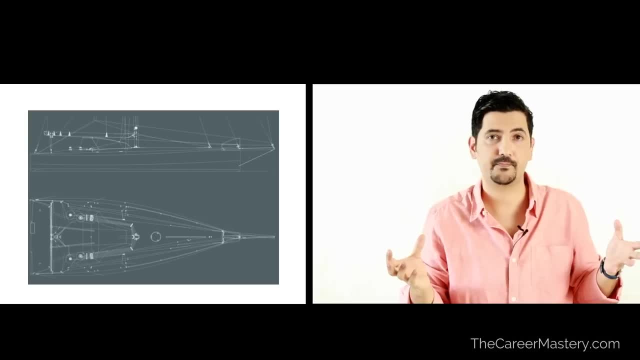 meter version of it, So it won't sail well, It won't float well. That means I increase the volume. After that I need to finalize a design. You see, thanks was complete And this actually why I actually design it or modify the design I have. 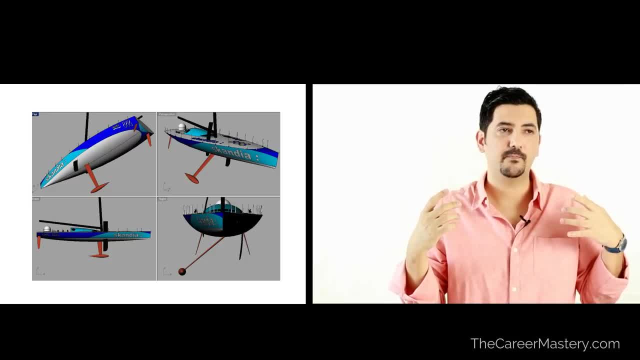 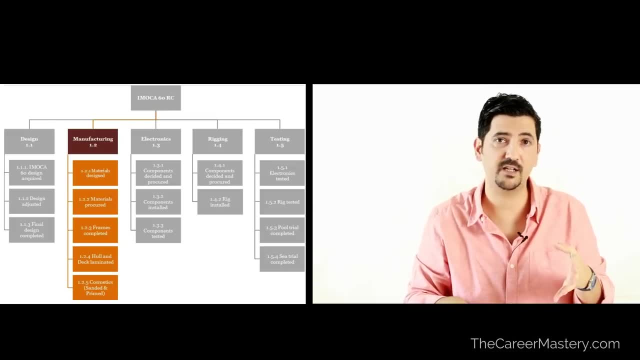 And this is multiplier or fluorescent solution. You see what I mean. I can always use View to adjust a book module where I make it ready for manufacturing. So for manufacturing, my work packages are. I need to decide on the materials and then 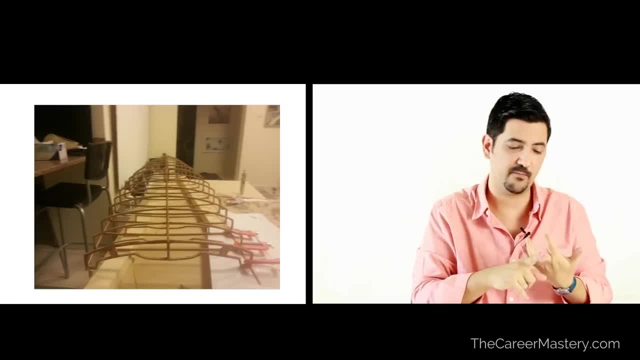 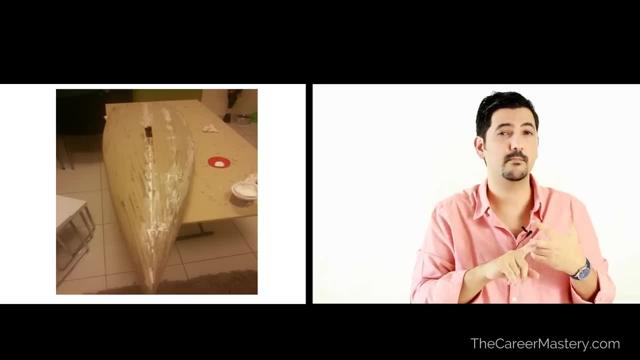 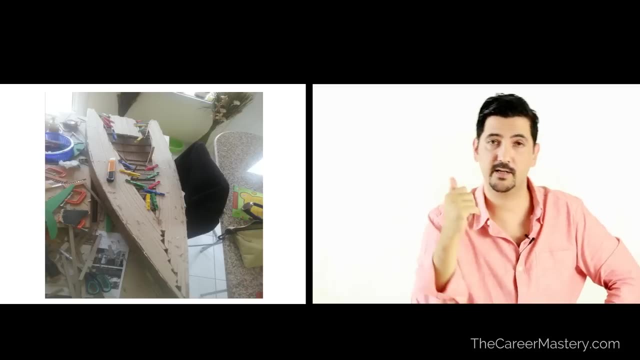 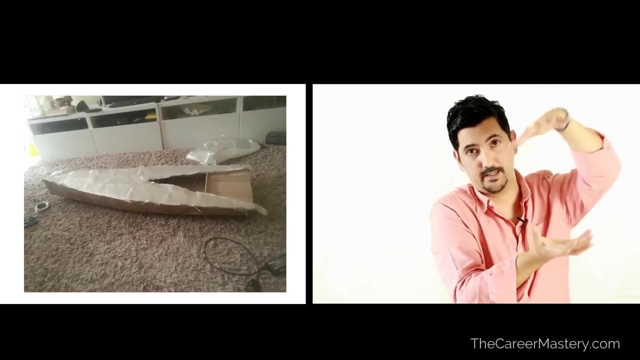 I need to procure them, then I need the frames. I need frame for the deck and the hull. then I need to laminate it. I need to again laminate the hull and the deck And then I need to assemble them together. you know, the hull part and the deck. 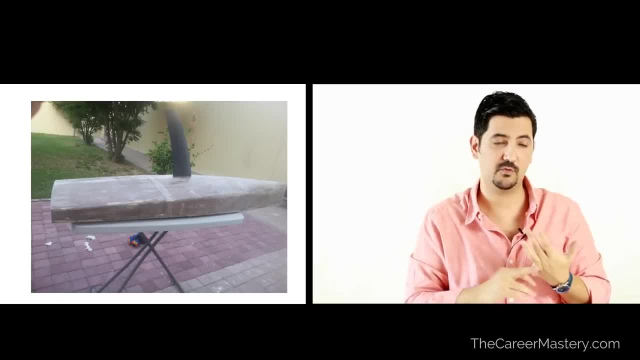 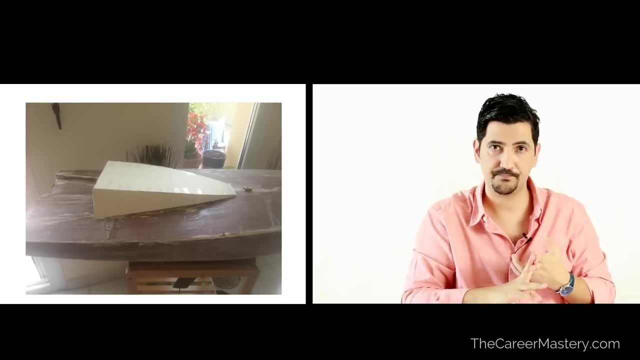 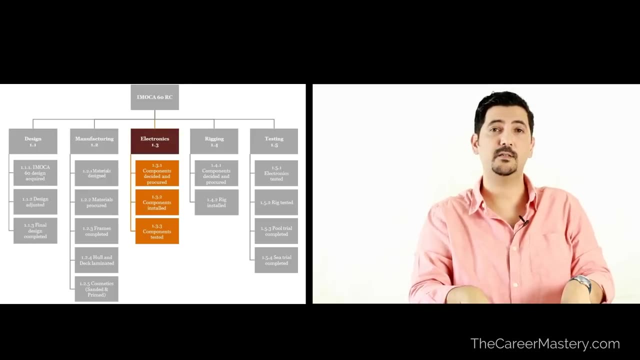 Then later on the cosmetics. So for cosmetics I need to do a lot of sanding, you know, And after sanding I will do the painting and yeah, yeah, I think that's pretty much it And that's pretty electronics. 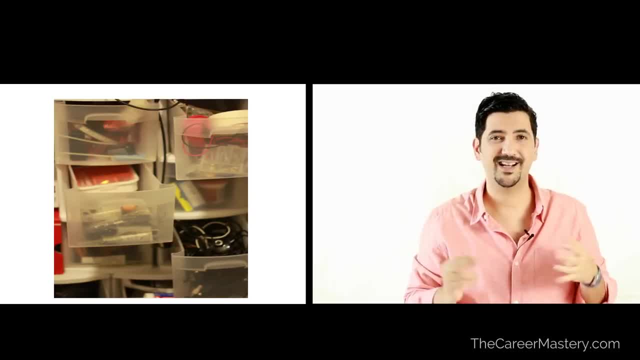 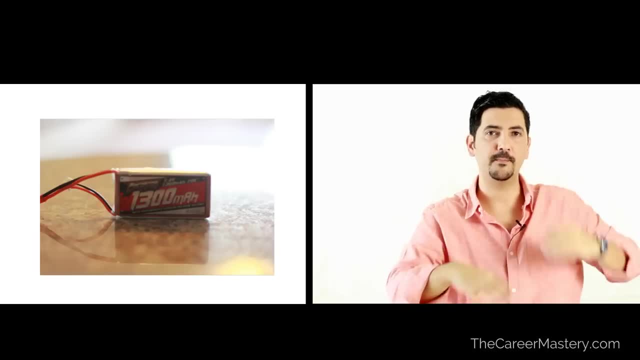 First packages. again, I need to decide on the components and procure them. I'd like to merge them under one work package So I can easily estimate the cost and time investment at this level. I don't need to break it down further. And then the second work package is: assembly. 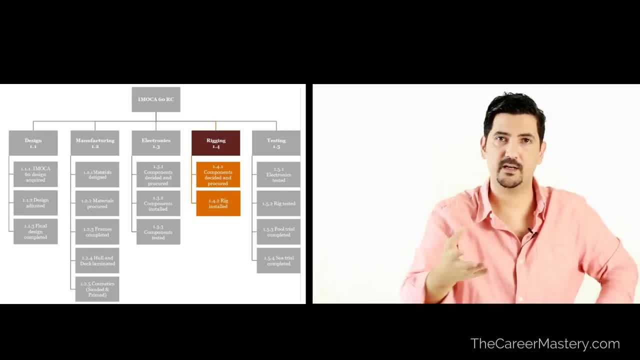 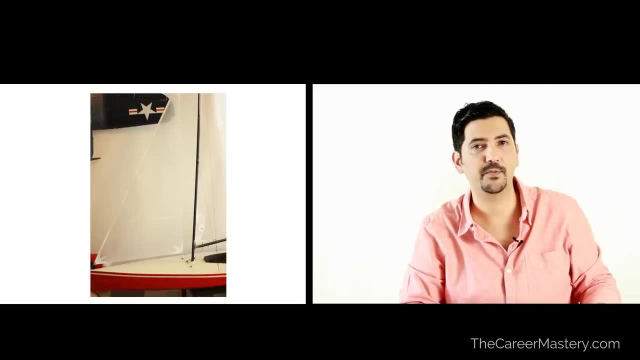 Then move on to rigging. The rigging is again, as I said, the mast, the boom, the sails, the lines, the shrouds, everything you know. So for that again, I need to decide on the items and then I need to procure them. 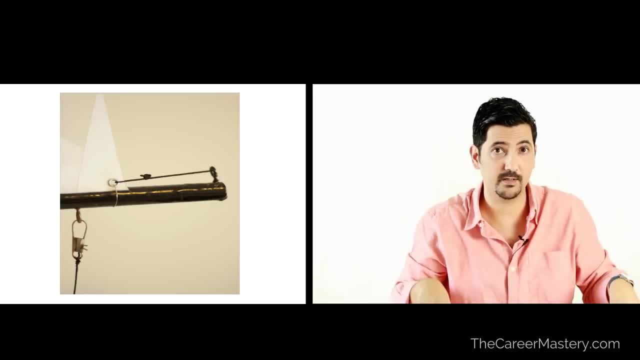 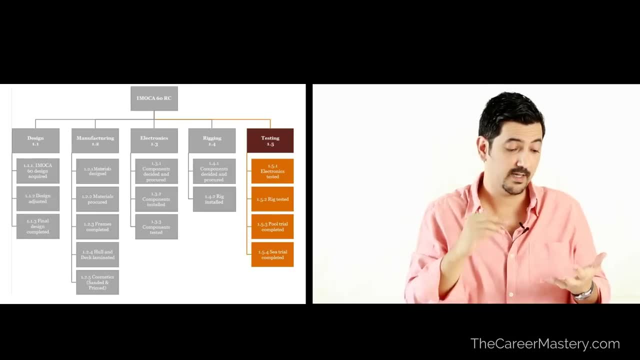 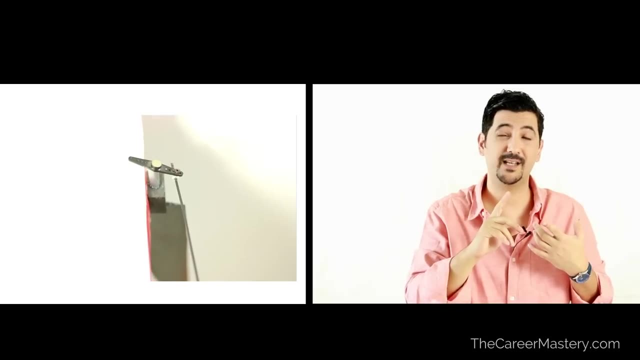 And then I need to install them, assemble them, yeah, And finally, the last one is testing. So I need to do the testing for the electronics, the rigging and the hull, And then I need to do a pool trial and finally, sea trial. 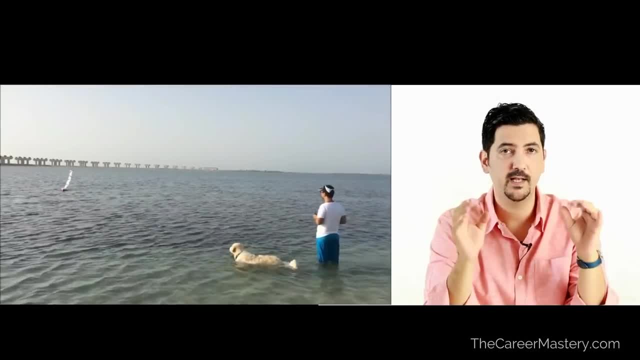 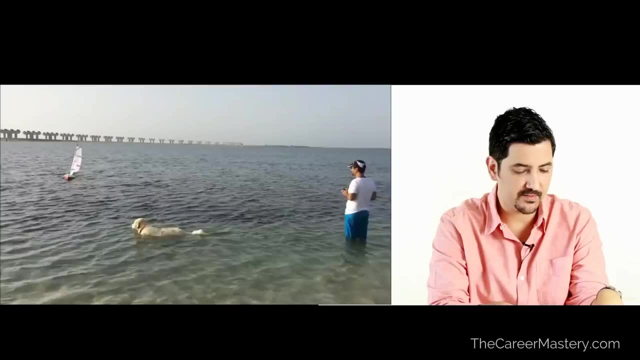 Okay, now we finished creating our WBS. Now I want to talk about the importance of this document once more. See, every time I create a WBS, I need to do a pool trial. I need to do a pool trial. Everything happens after WBS. In the planning process, for example, the cost schedule risks. everything is calculated by using this chart. We do not calculate the cost or the schedule for a project as a whole. We do that at work package level using the WBS. 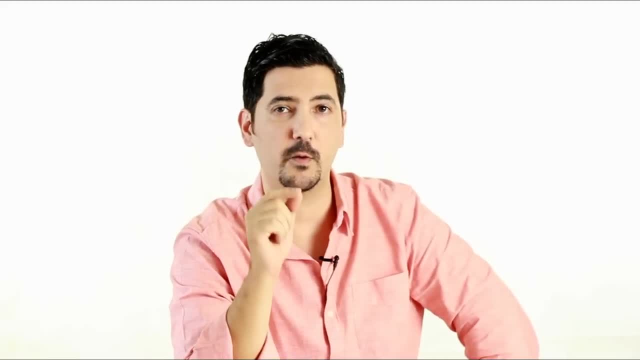 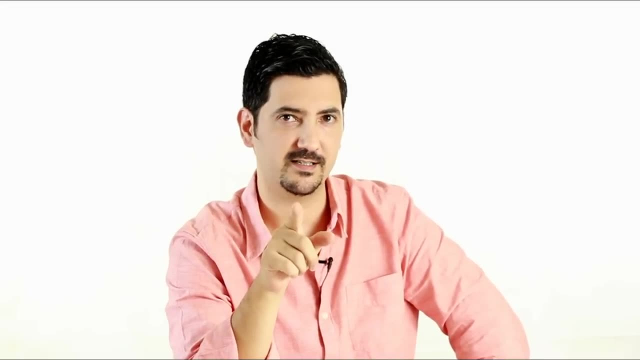 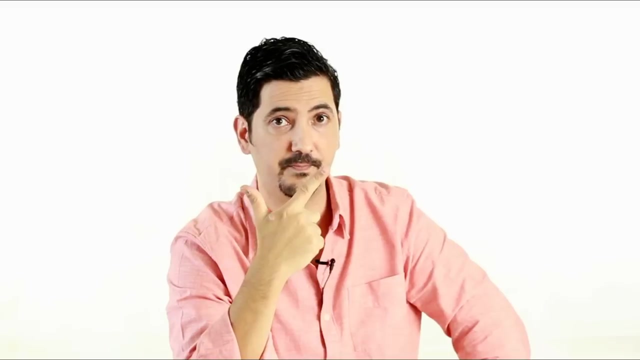 Now, before we move on to the other processes, I want to remind you of something, Something, Something that I mentioned earlier. Do you remember the scope baseline? Do you remember what it was consisted of? Let me just remind you once more: It's the project scope, WBS and WBS dictionary. 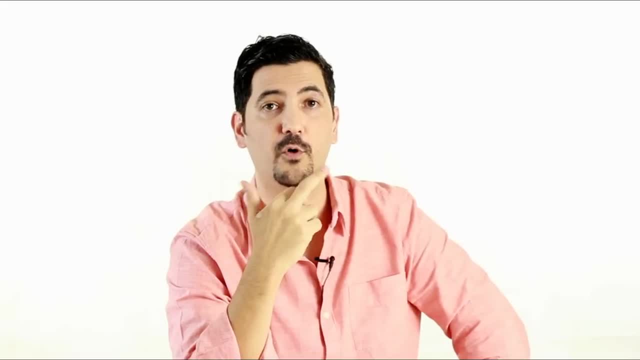 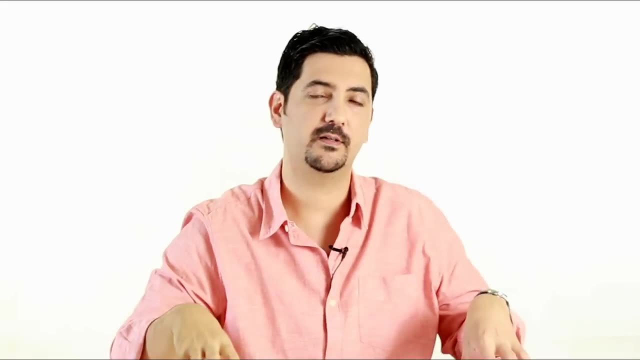 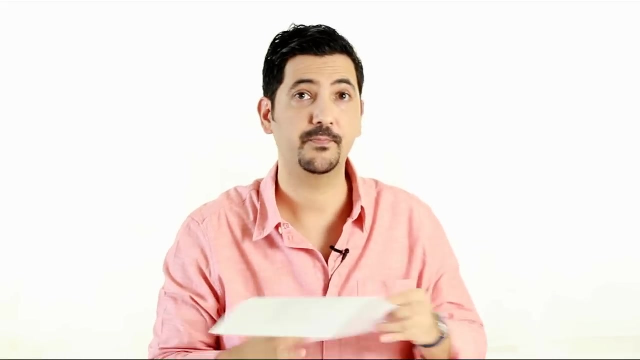 So now we covered the first two. Now it's time for the third one, WBS dictionary. And once we have it, then the project scope baseline is completed. Okay, So what is this dictionary thingy? Let me just find it as well. 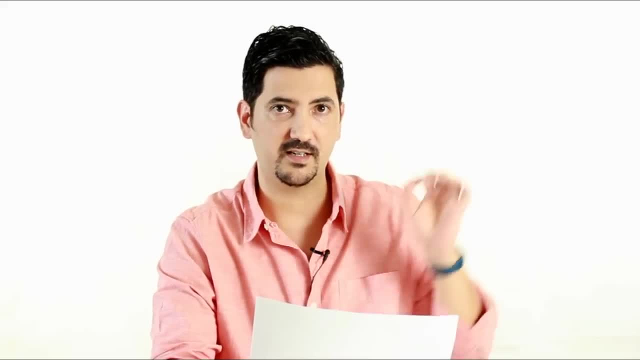 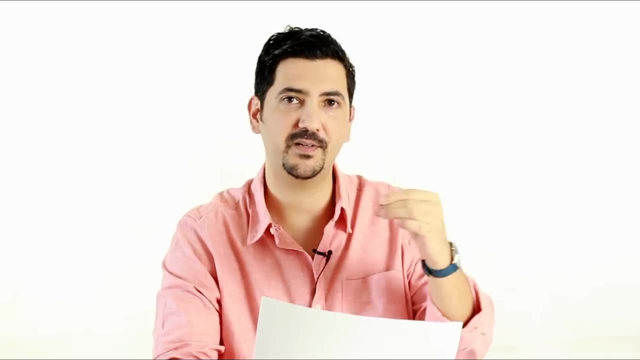 So imagine this: If we don't define these work packages in WBS properly, then we are prone to a scope creep. Now, what is scope creep? Scope creep is basically scope extending its boundaries. Remember the Porsche 911 GT3 that I wanted from my wife? 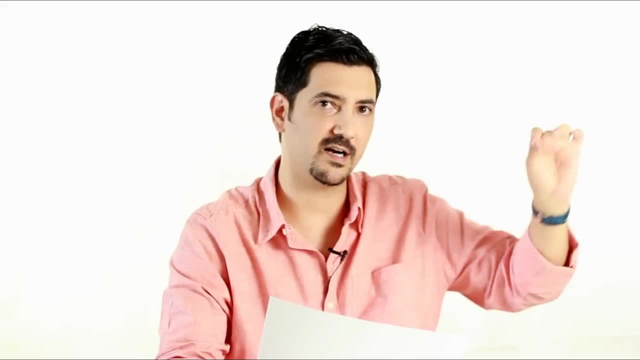 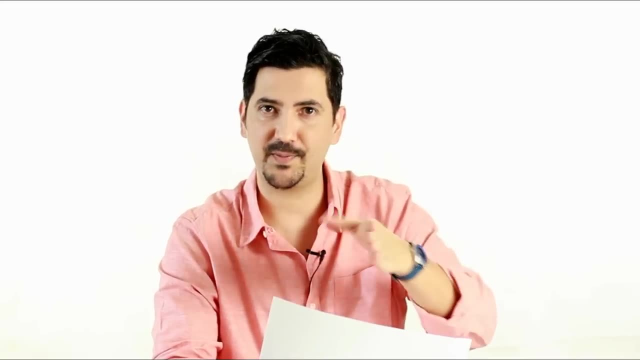 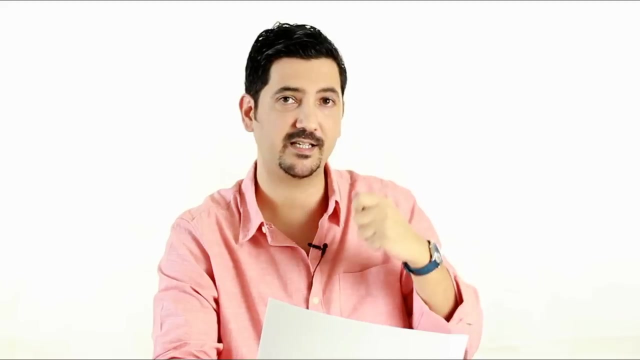 So that Porsche 911 GT3 becomes GT3 RS, basically a higher model. So if you don't control and keep the leash, Then it keeps on getting expanded and expanded. Your stakeholders are going to want to stretch its limits And to prevent it. what you do is you create a dictionary for every single WBS item. 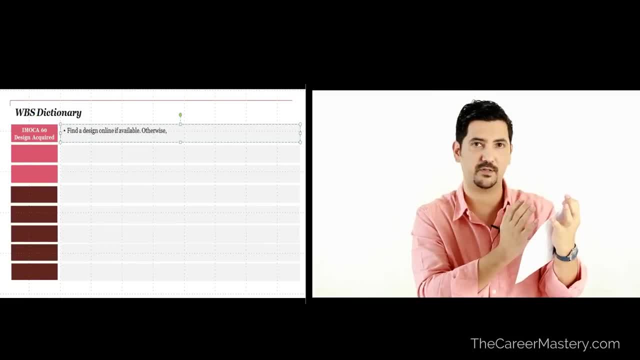 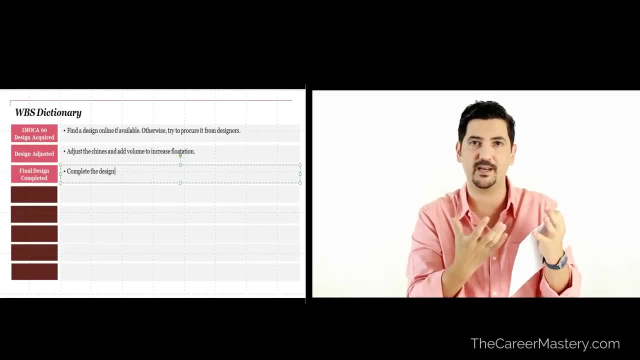 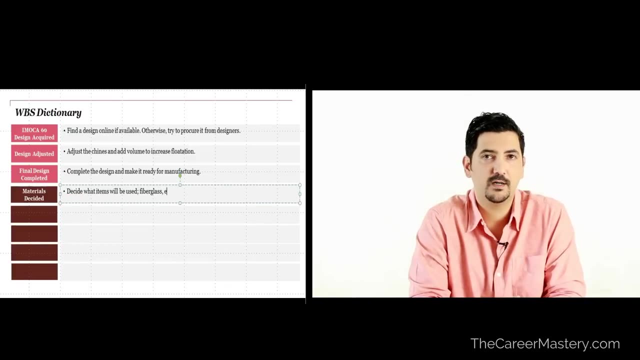 What does that mean? What are the boundaries of it? What do you mean by work package, whole framed, So you put boundaries around it. You explain it By that way. nobody can stretch it. Okay, For those of you who are preparing for a PMP test or a CAPM test, you'll know that there 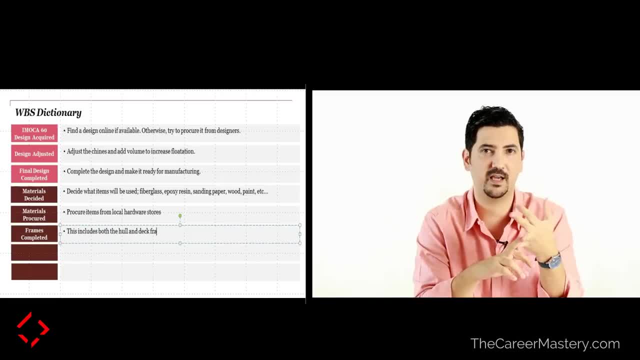 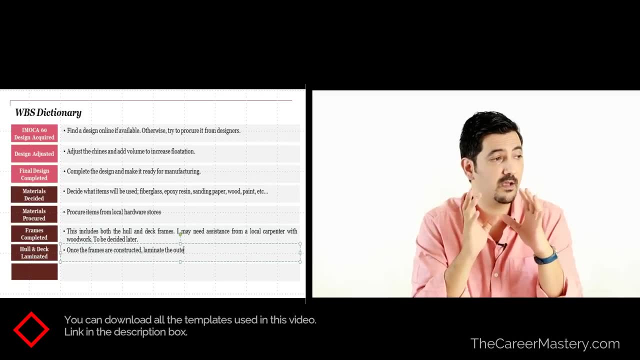 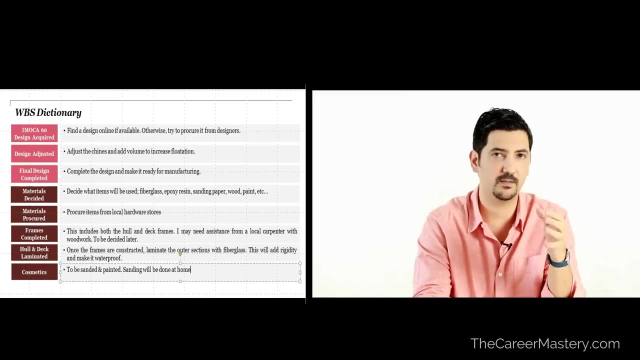 are a few other knowledge areas like human resources and communications and risk management, procurement and a couple others, So I'm not going to cover them here for a few reasons. One: I don't think they need explanation. Most of them are fairly easy to understand once you read the PMBOK. 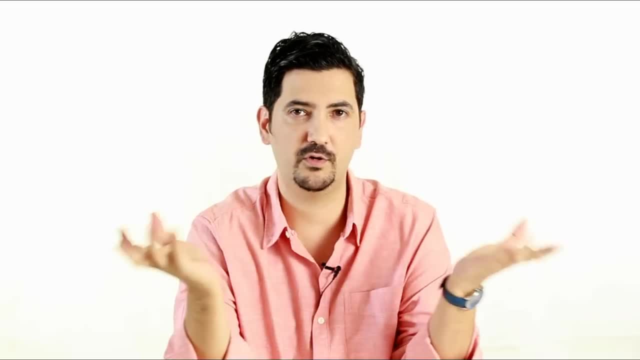 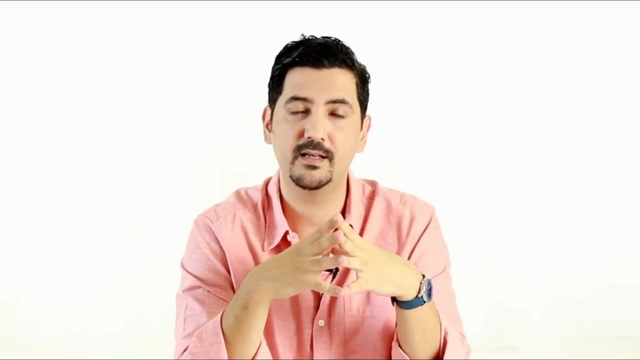 They're very intuitive. You don't need me to teach you about procurement or human resources. The only exception, in my opinion, is risk management. See, that's not very easy, But I won't talk about risk management here because I will probably have a dedicated video. 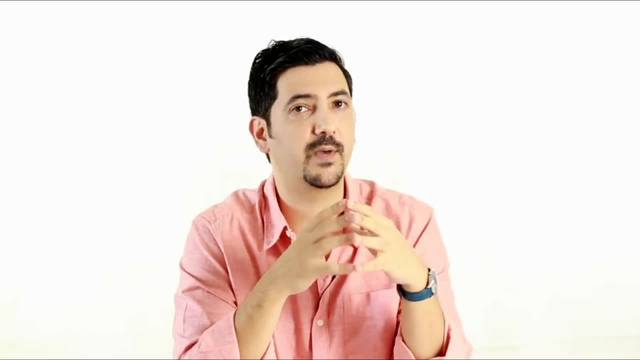 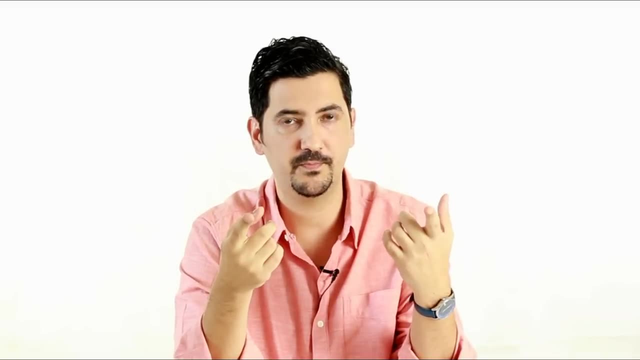 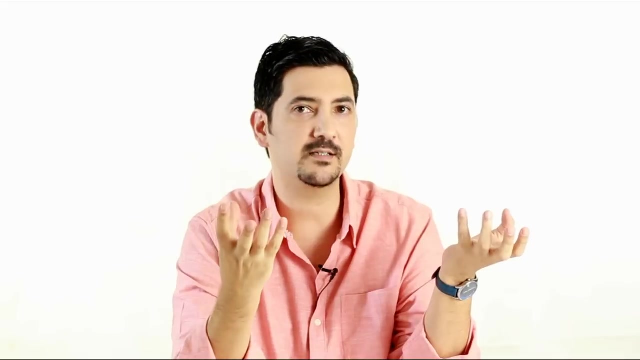 on that later, Maybe next month, And I don't want to spend an hour running risk management simulations here. Plus, for most of you- like 99% of you running small projects- you don't factor in risk management anyways. You are aware of the risks but you don't go out of your way to spend a week on preparing 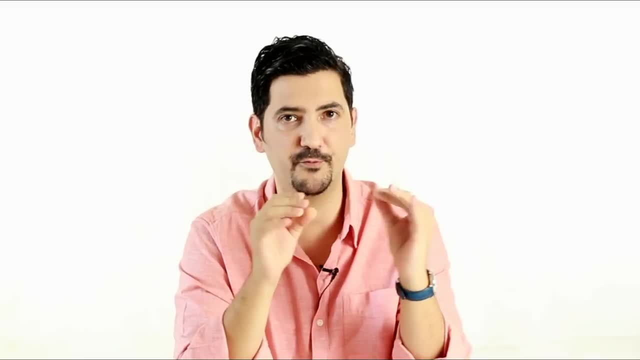 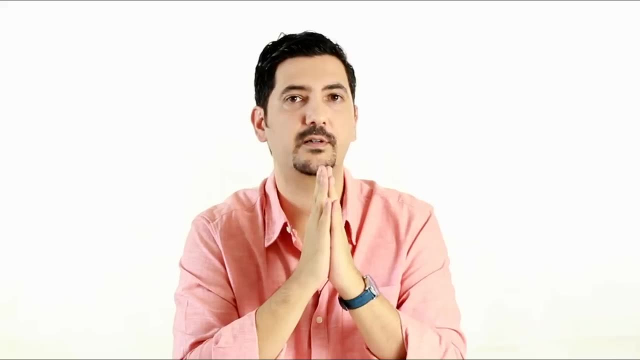 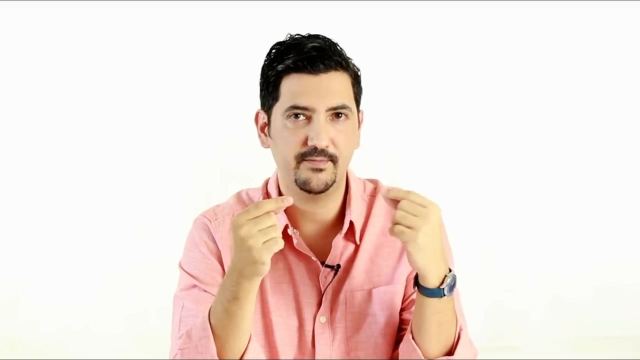 risk registers, So instead I'll focus on, in my opinion, more essential ones here. So let's continue with time management, the schedule, And what we do is we start giving estimates for how long a particular work package will take. 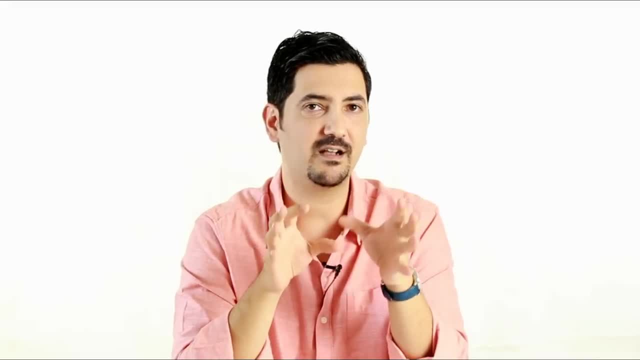 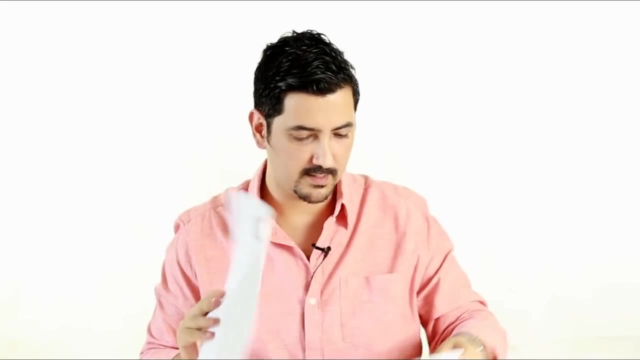 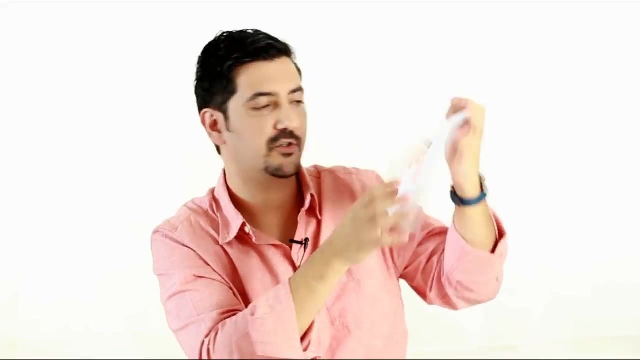 Here's an important point for you: If you can't confidently estimate how long a particular work package will take to complete, then you need to do what You need to break it down further. So let's pick one: Materials decided as part of manufacturing. 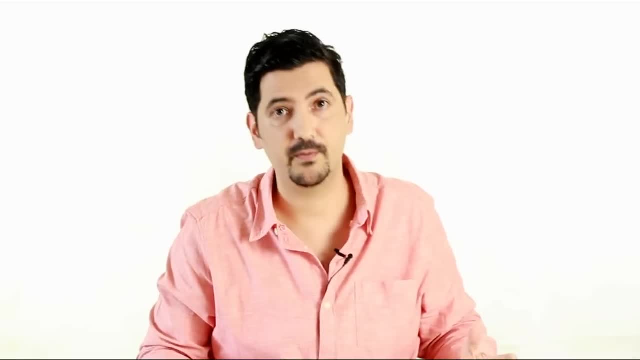 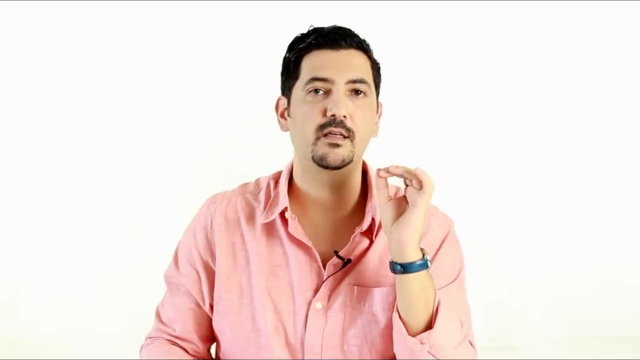 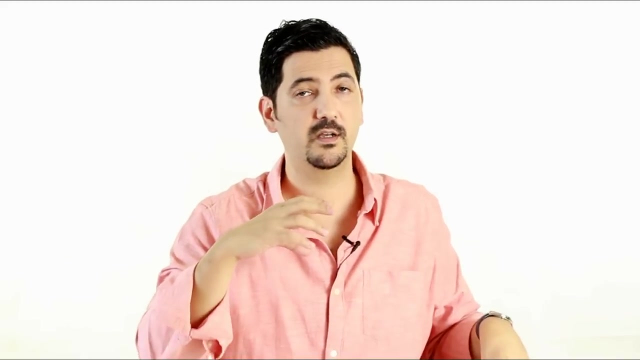 Do I know how long it takes? Yeah, I know it, So I don't need to break it down further. And once you're done estimating these, The other fun point Parts starts, And that's putting them in a sequence. Now for PMP takers, you need to resort to PMBOK guide for boring details of finish to. 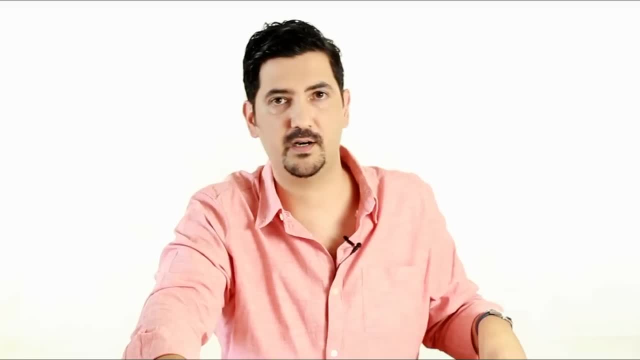 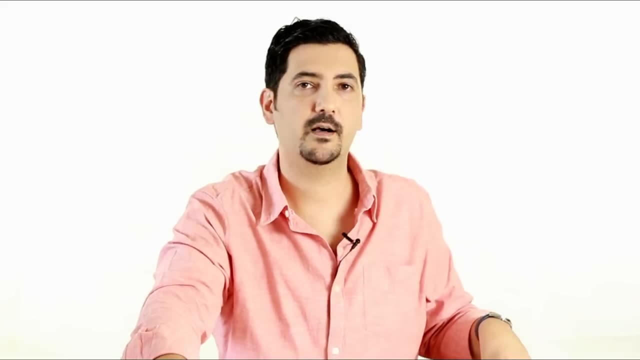 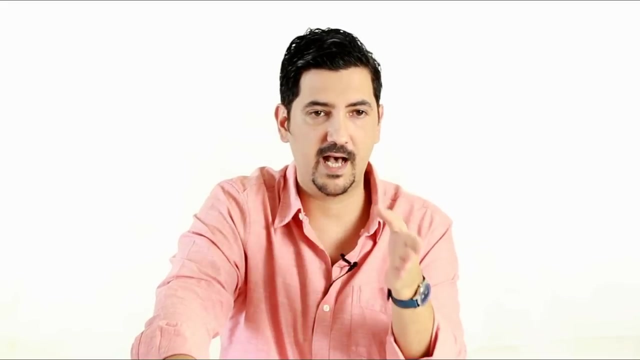 start, start to finish, and calculations of critical path For all of you. for the rest of you, you don't need to, because I am going to show you a lot easier way. So in practice we do all of those with the help of MS projects. 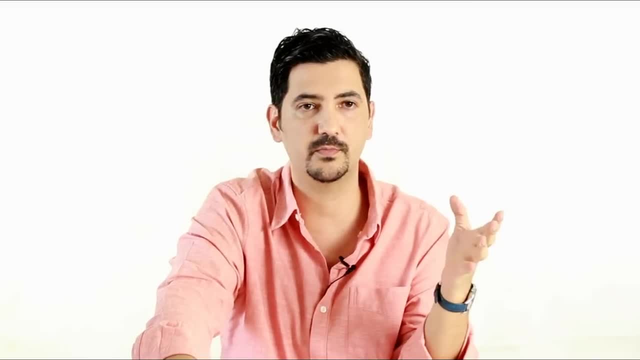 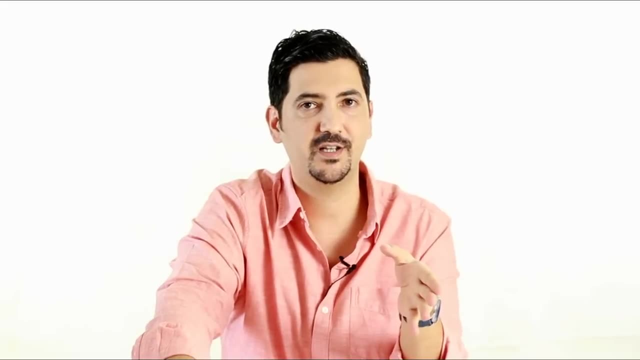 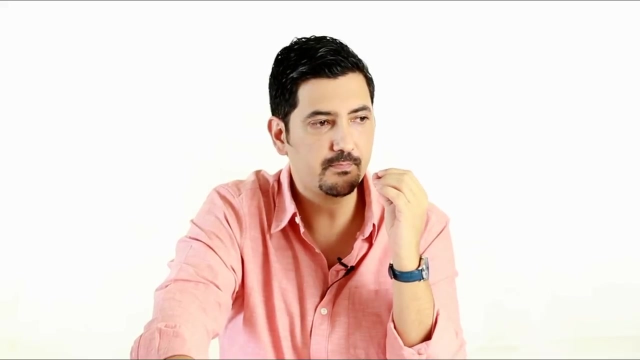 MS projects is very easy And it's an awesome, awesome program. But you don't even need MS projects for most of your projects. All you need at this stage is a Gantt chart, So Gantt chart is very easy to use. 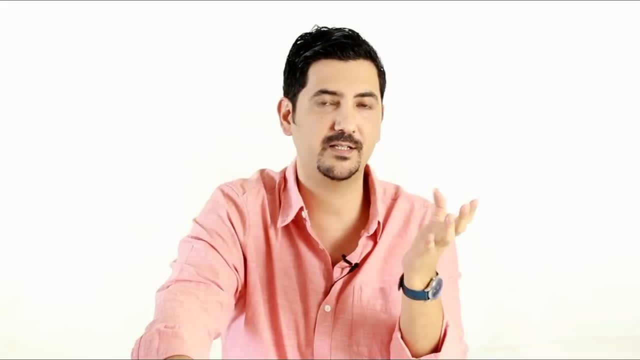 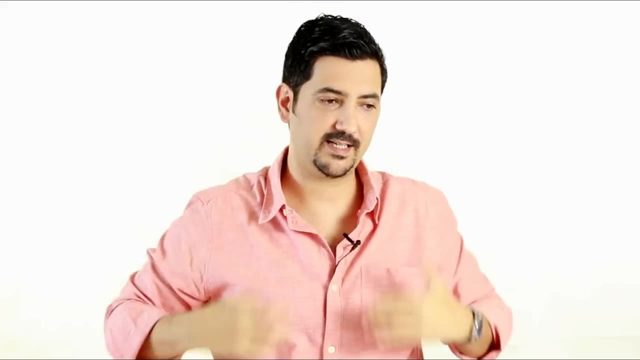 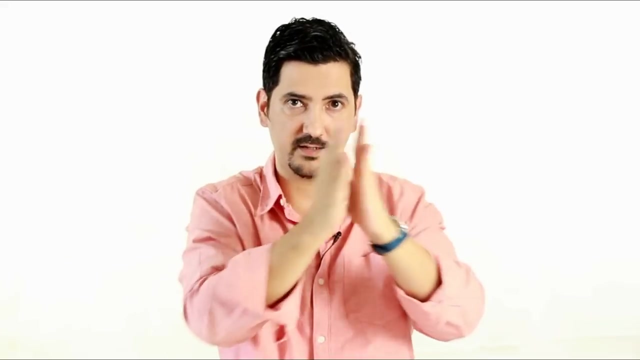 It makes things so simple And it's very easy to list your activities or work packages in a suitable time scale. Each work package or activity is represented by a Gantt chart. It is represented by a bar that shows us the start date, the duration, the length of it. 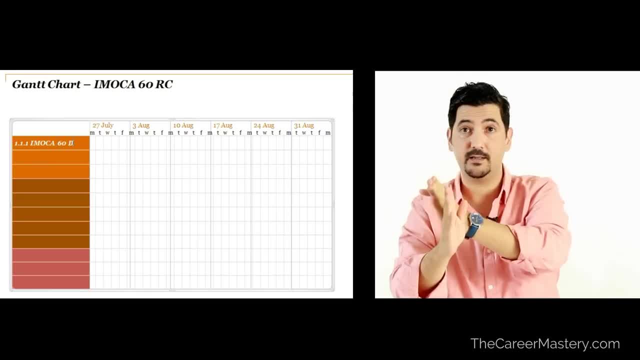 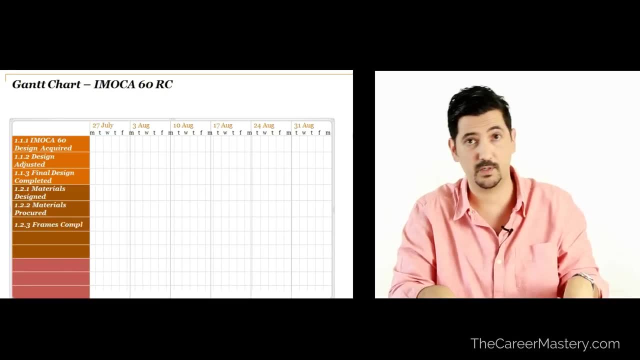 is the duration and the end date of the activity. So it's very simple. You can use MS projects, you can use MS Excel, or even manually on a powerpoint if you want to. So it really depends on how complex your project is, right. 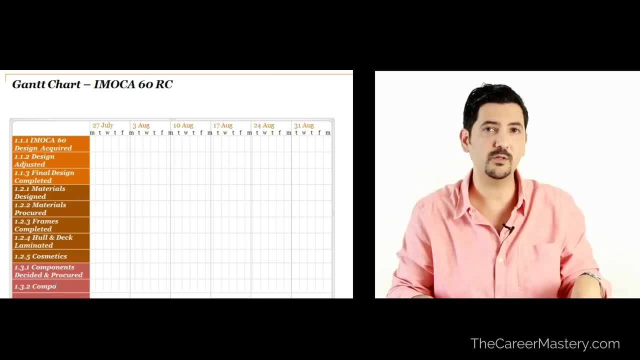 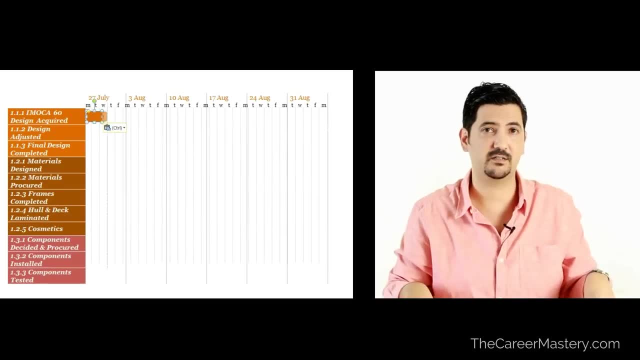 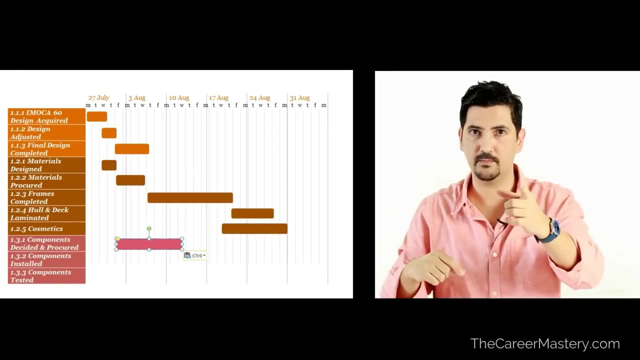 So for me, and probably for you too, all you need is just a powerpoint. You don't even need Excel, You don't need to run calculations or anything, Just manually do it on powerpoint. And that's how I'm going to do, demonstrating how I did it for you. 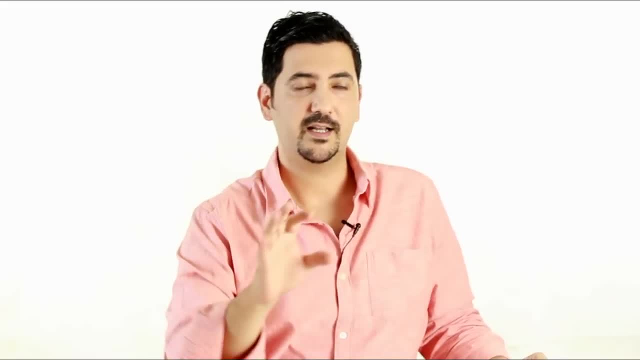 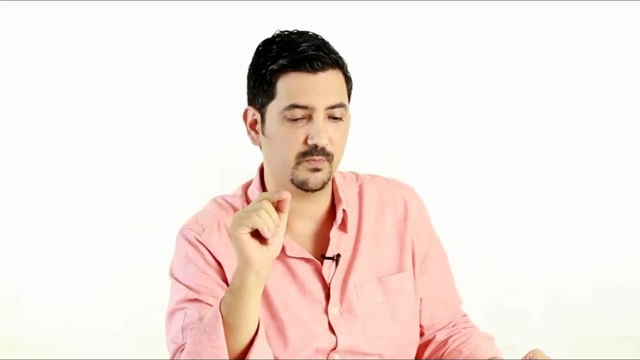 If I could speak. So, if you're still with me by this point, please consider subscribing to my channel because, as I said, if you don't, YouTube will not show my future videos to you. In fact, you can even hit that bell icon so you'll be immediately notified of my future. 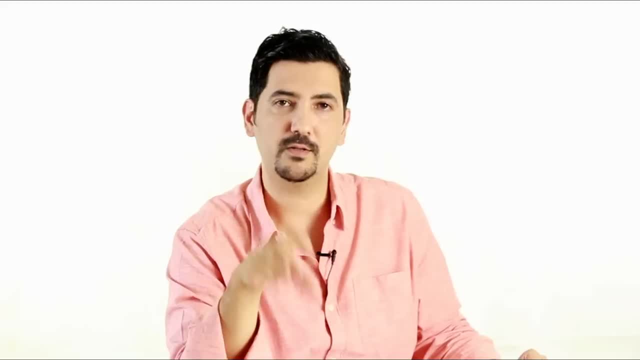 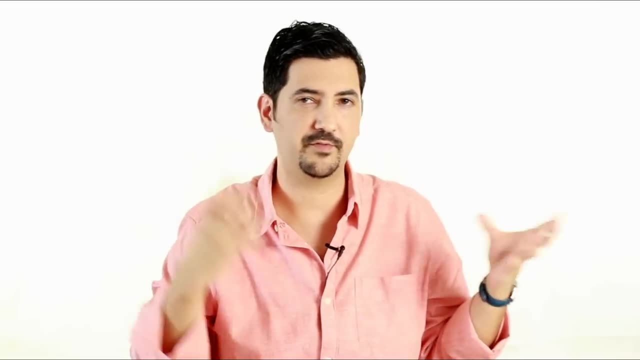 releases. Oh, You can also download all the templates I used in this mini course from the link down in the description. You may need to register, though I'm not sure. I haven't figured out how to do it yet, So sorry, I digress. 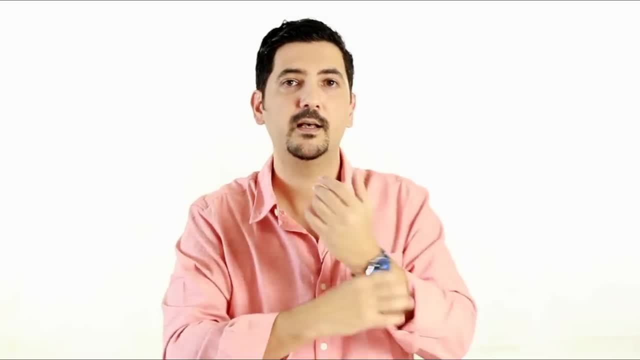 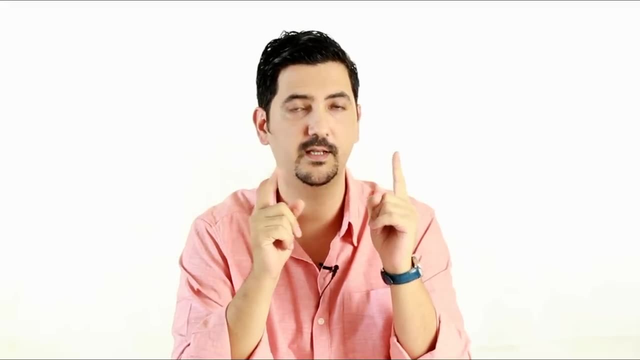 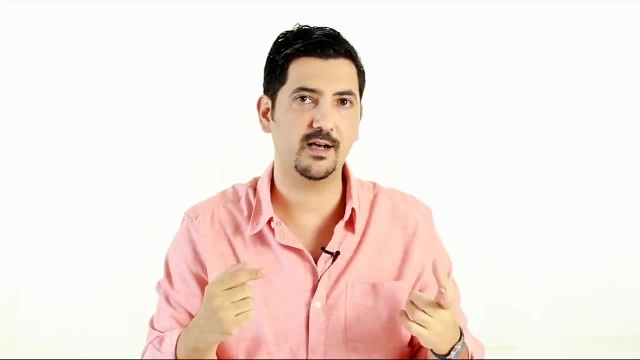 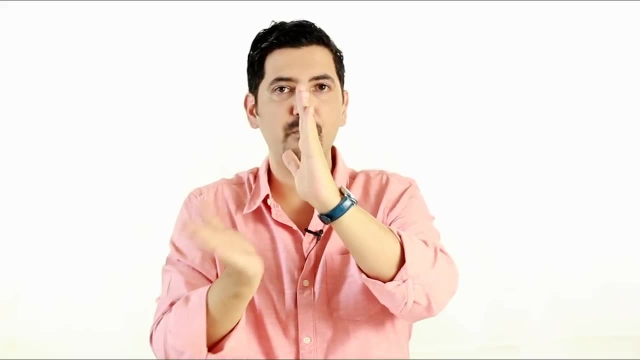 Fast tracking another project means teleporting or downloading it. Fast tracking another project means müs those activities in a specific way, in parallel. So you see more bars along the same vertical axis. Last thing you hear a lot is called project crashing. Crashing in simple terms is shortening the duration of the activities by adding more. 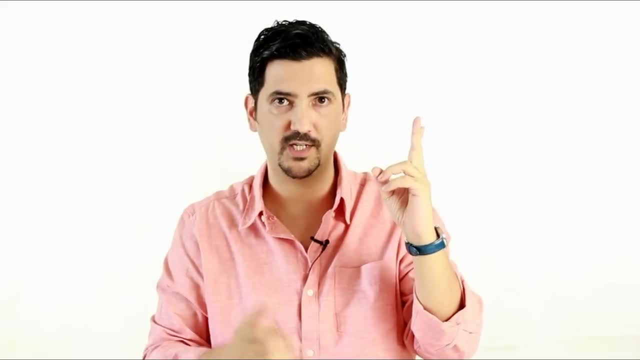 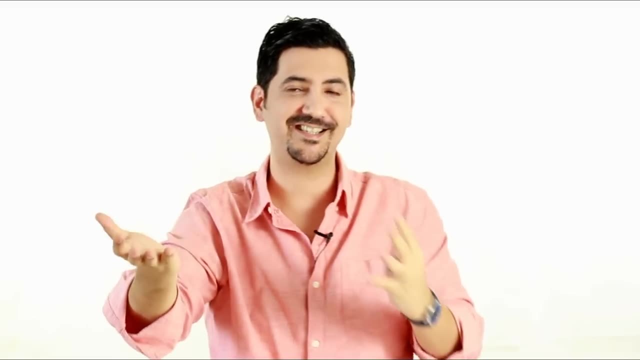 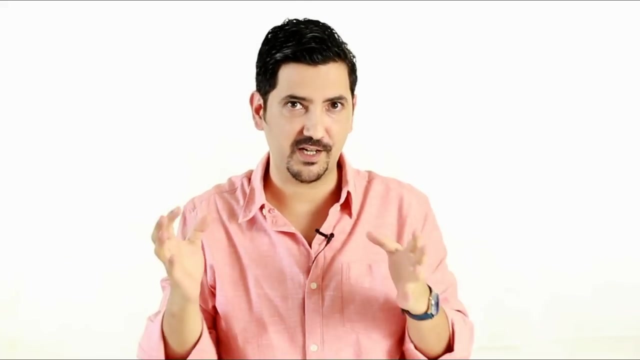 resources. For example, if 2 workers finish the project in thirty days, then how long does it take for 4 workers to finish it? 15 days, if you said 60, you need a break. So this is called Project Crashing, but it comes at a cost, right? 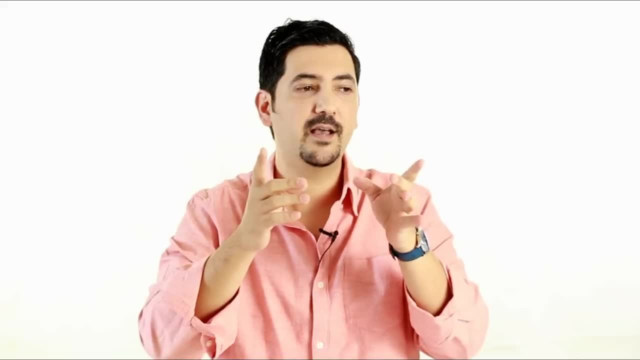 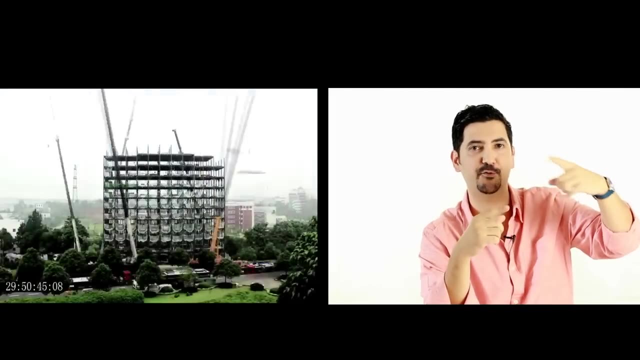 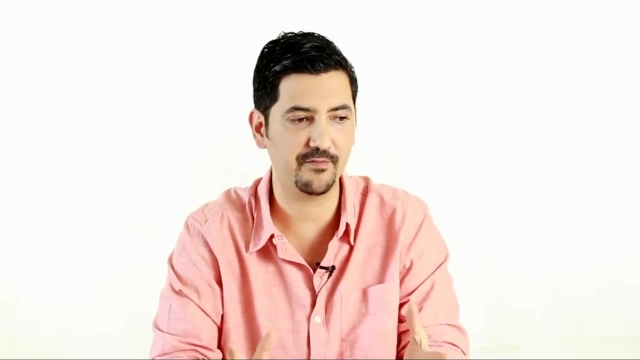 Cost of additional resources, additional money. So have you seen those huge towers being built in China in 30 days? You can see their footage. they are amazing. This is what they do: They just crash every single work package because they don't have a labor shortage. 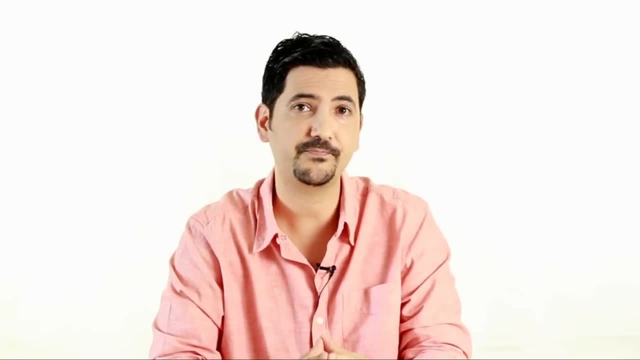 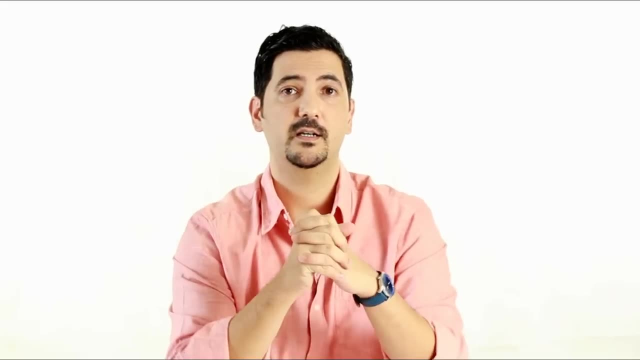 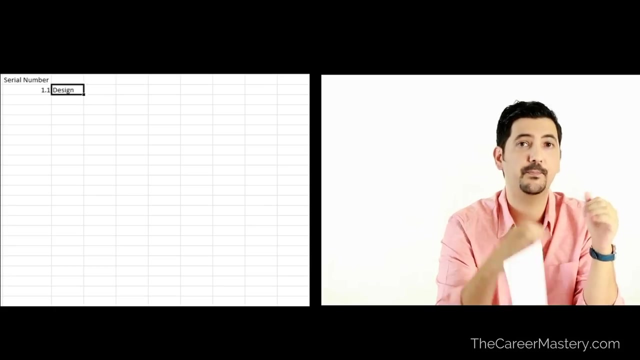 and probably no money shortage either. So that's how they do it. Now let's move on with the costs: Cost Management. Now for this piece, we'll take out our beloved WBS again, But instead of putting durations now, we'll give our cost assumptions. 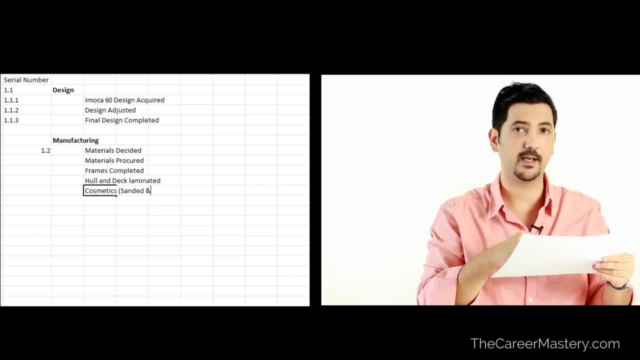 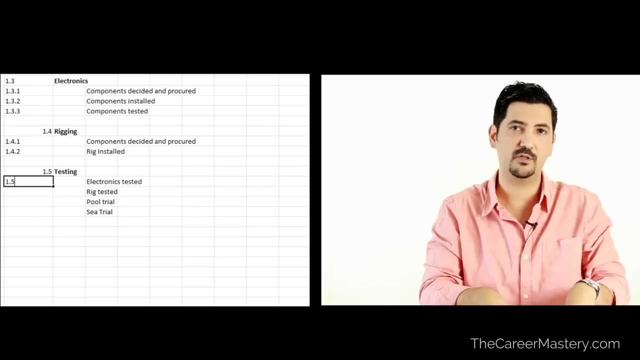 Fairly simple, right? So we'll do a bottom-up estimating and then start giving our cost assumptions for each work package- Again, very similar to what we did for Schedule Management. But once you have all the costs added up, you may need to use Excel to give the easy. 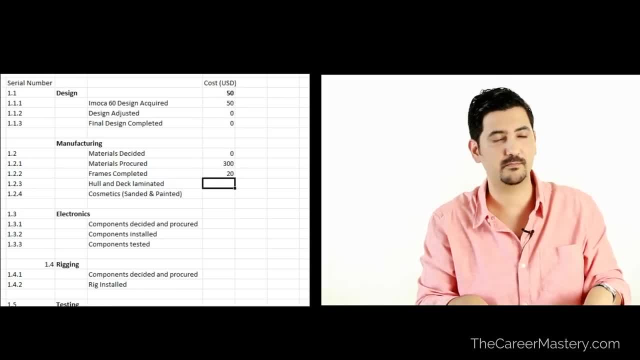 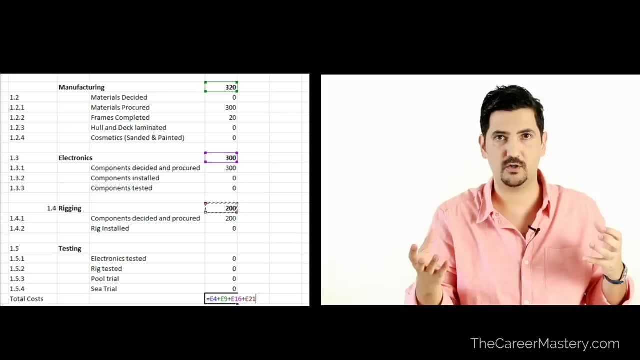 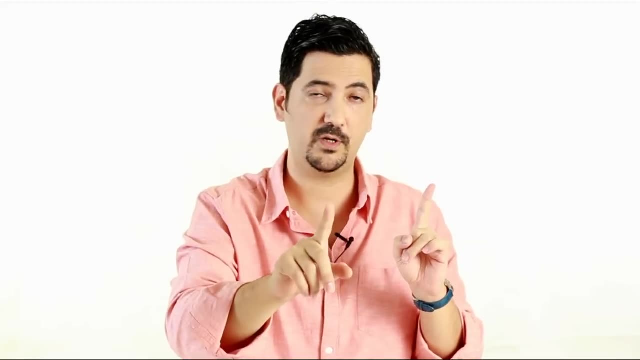 calculations. Powerpoint won't do fine here. So once you have all the costs added up- the direct costs, indirect costs, variable and fixed costs if you want to- then you can create a budget For those PMP takers. keep in mind that there are a few more steps for you. 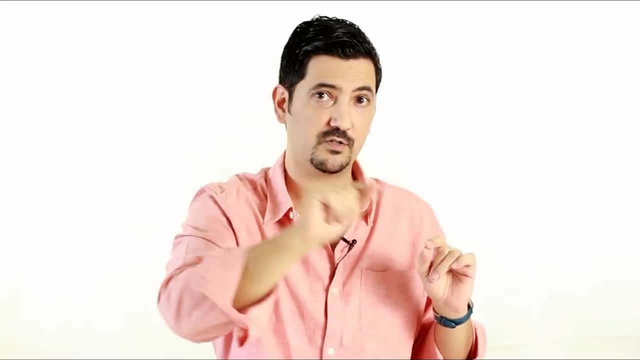 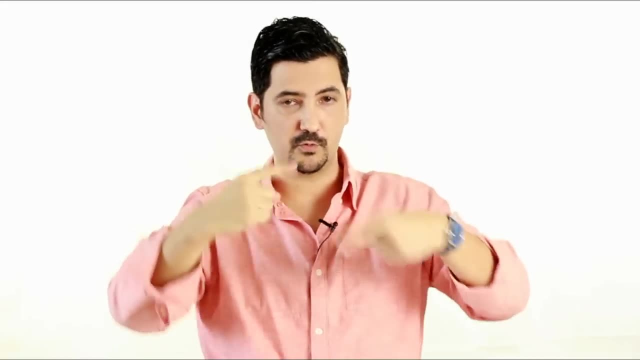 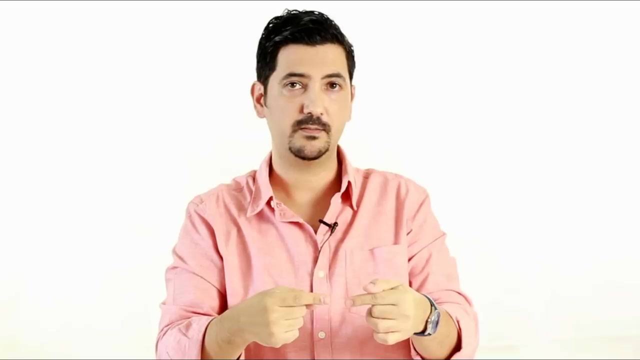 For example, You need your risk register And risk contingency activities to be included in your budget. Not just that, you also need your management reserves. So the way it works is you roll up, Get your cost estimates for activities, then work packages. then you'll have a rough. 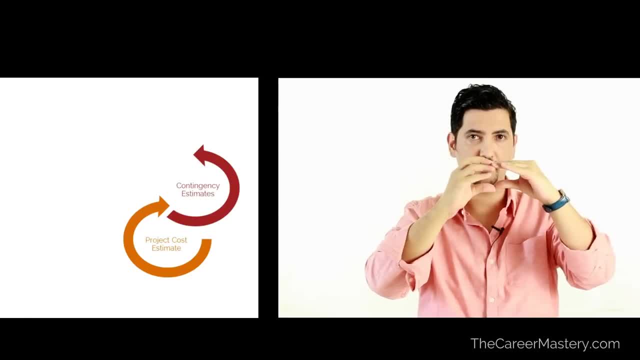 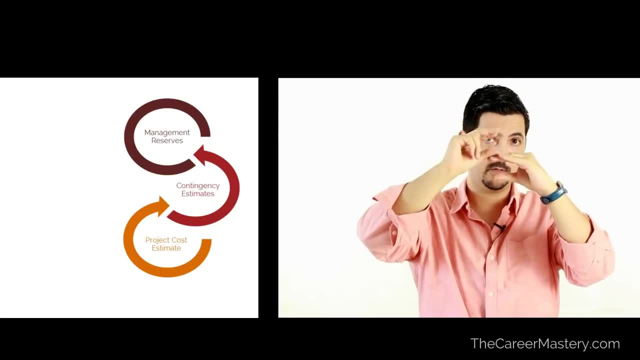 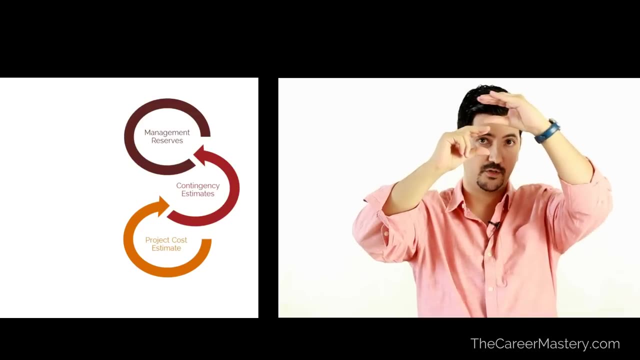 idea of the project cost estimate And once you have it, you include the contingency estimates which comes from your risk studies. You include that, and that gives you your cost baseline. Then you include the management reserves and voila, you have your cost budget. 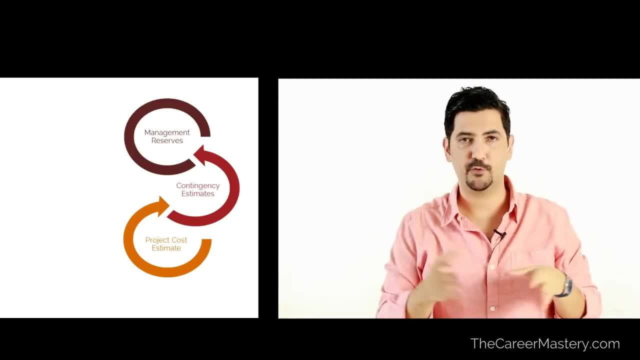 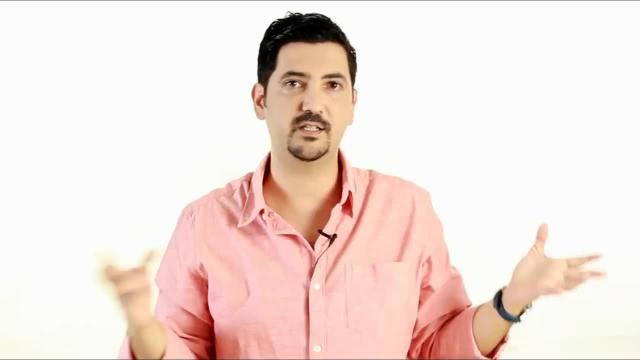 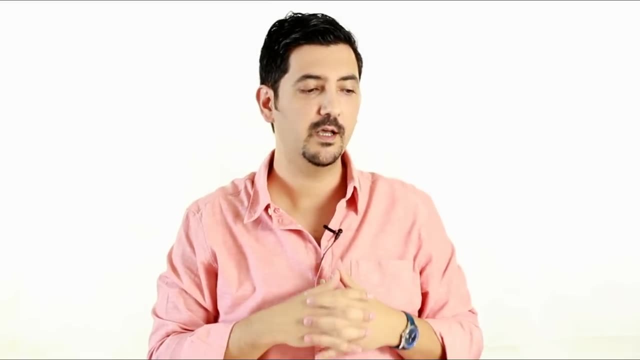 That's pretty much it And, as I said, for 99% of us we don't really do that in practice. We roll up the cost of each work package and then put a 20% contingency reserve and we are done, So no need to complicate anything that we don't have to. 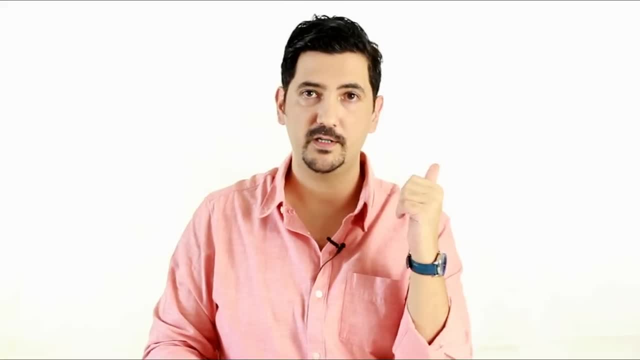 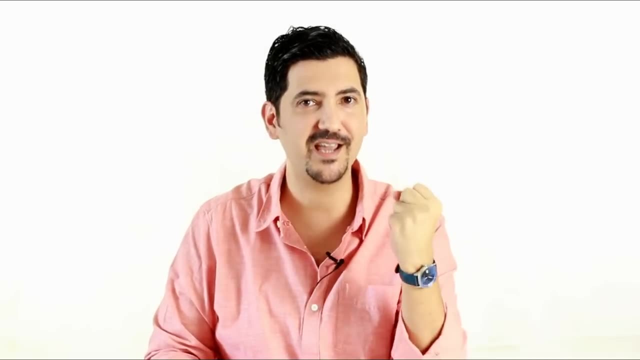 You know we are done with planning. Alright, so far, we are done with the initiation, we are done with planning and now it's the fun part, The execution. You know, It's the doing part, It's where we execute things. 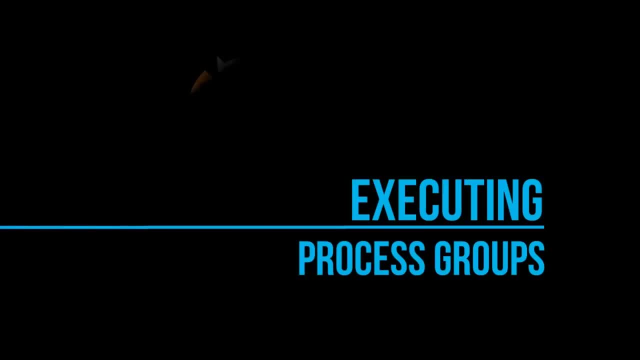 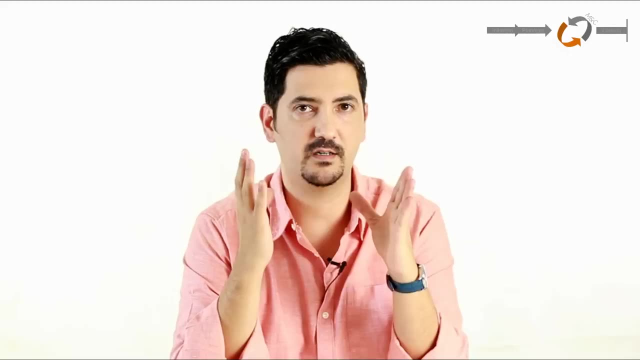 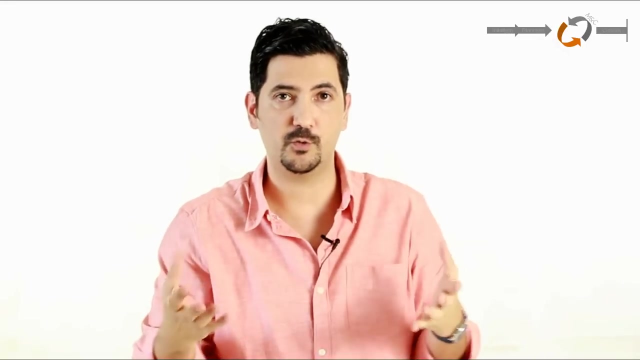 It's the fun part. Now let's do it. The purpose of the executing process is to complete the work we defined in project management plan. You know: meet the objectives. This is where we do the work. Your focus now is as a project manager. I am assuming you take the project manager. 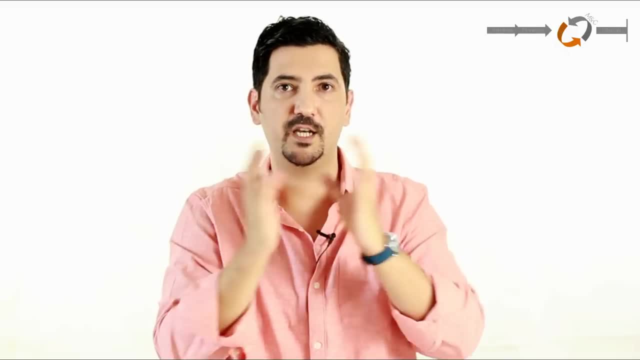 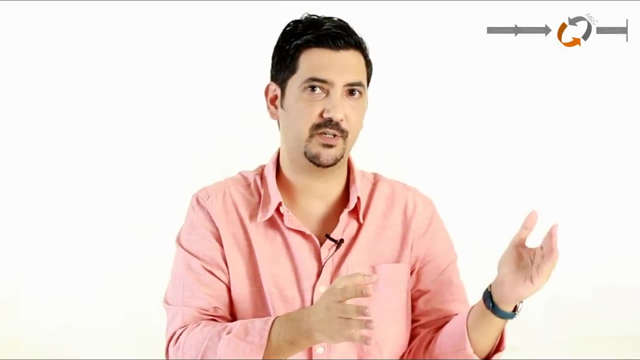 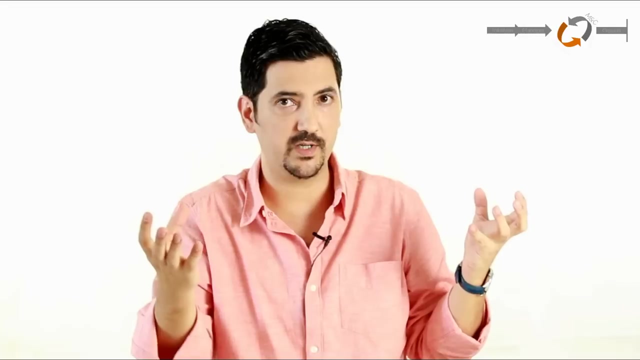 role is to manage your team, follow processes, conflict resolution. Your job is essentially guiding the team to stick to the plan you created with your team. So if you have done a good job with planning, then your execution is going to be so easy. 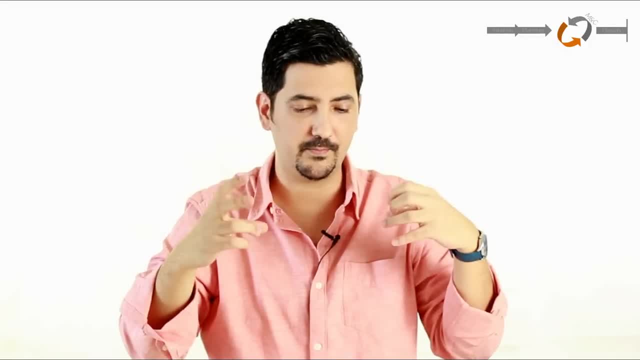 Although it takes the longest, but it's just like playing with Legos: You just put them in their places. But if you have a good plan, then your execution is going to be so easy. If you haven't done a good job with the planning, then your execution is going to. 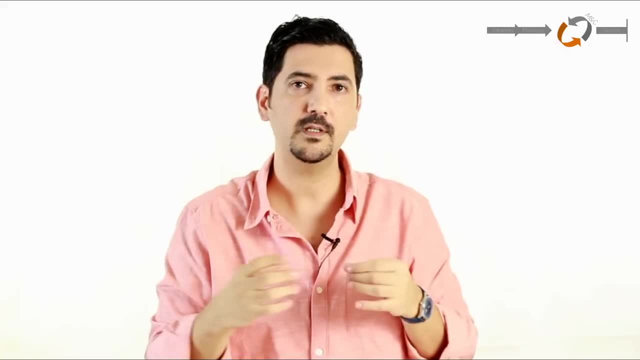 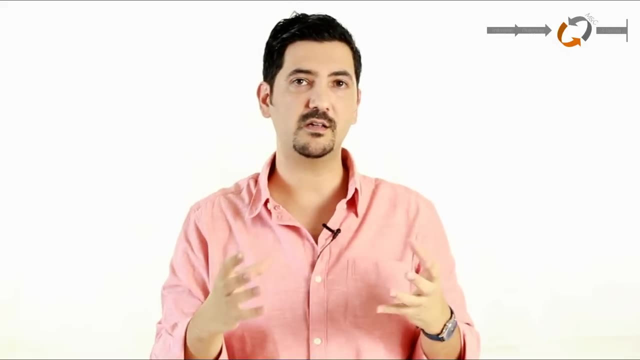 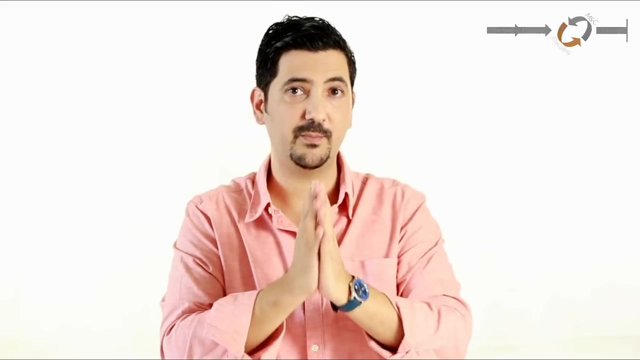 be a nightmare. So in execution, if you are not the one doing all the execution work, you need to constantly manage the expectations of stakeholders. You need to protect your scope. I talked about the importance of this before, Because you'll quickly realize that the stakeholders will want you to gold plate. 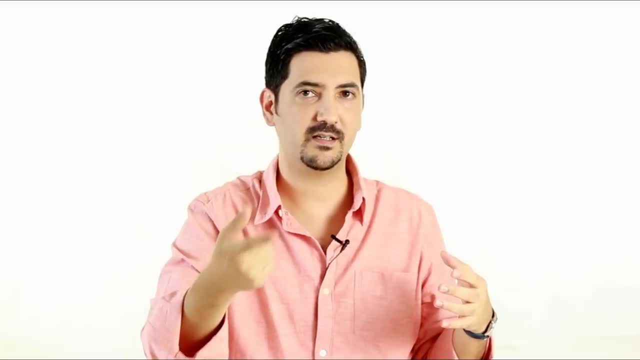 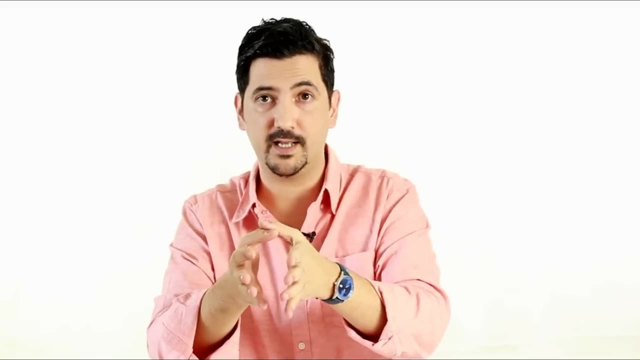 Do you know what that is? The gold plating? It's in simple terms, It's making changes to a project that are outside of your scope. Instead of getting the grade B quality material, as you agreed, your stakeholders now want you to get grade A quality. 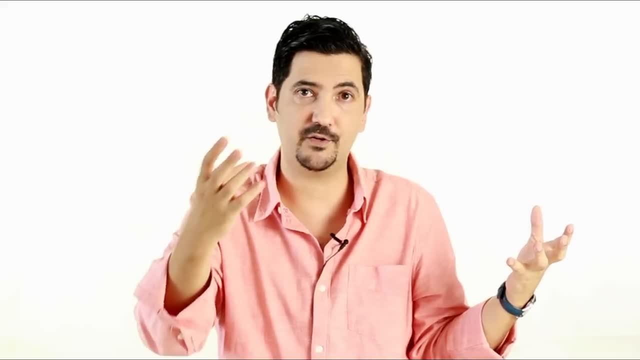 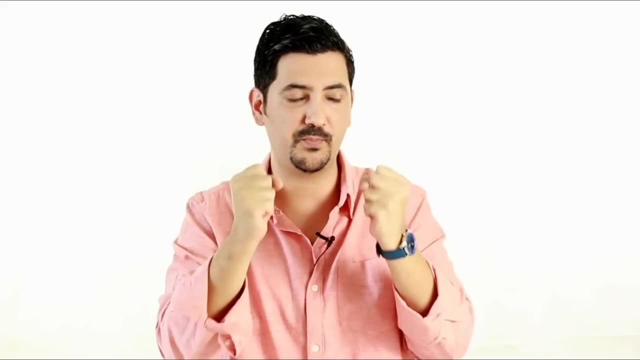 Now this is a problem because you didn't factor that in your budget or time estimates. So, as a project manager, you need to prevent scope creep, Protect your scope. Your scope is like your national flag. You protect it against all unnecessary change requests. 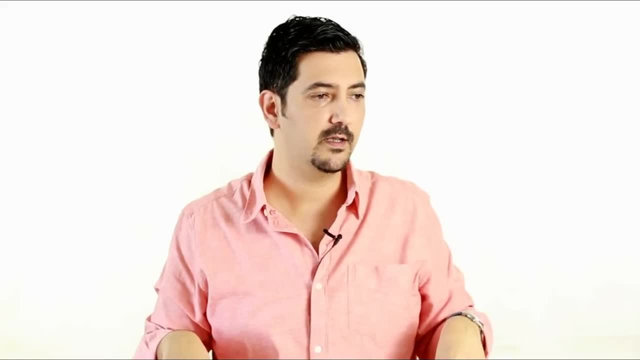 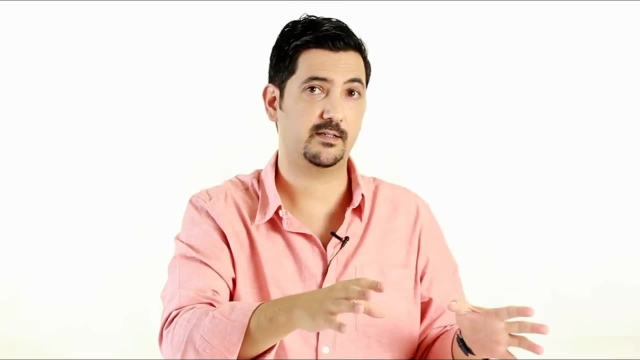 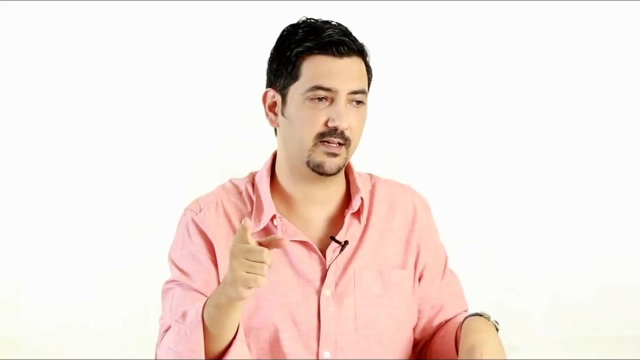 You resist. If they are really really legitimate ones, you can evaluate it and put it in consideration if it's really valid with a change request. But don't just take it as is, Don't say OK, no problem For those PMP takers or CAPM takers. pay attention to change requests and how it's done. 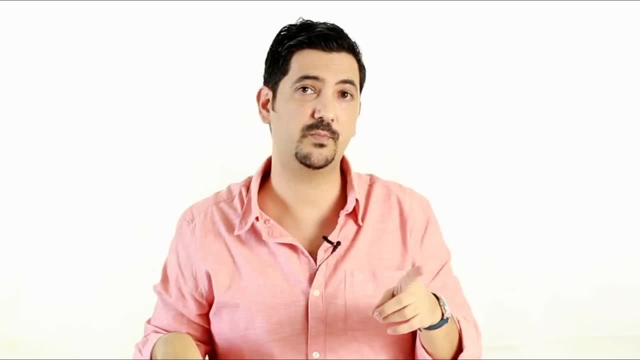 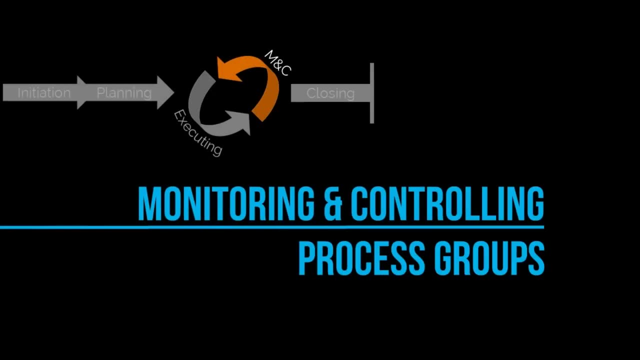 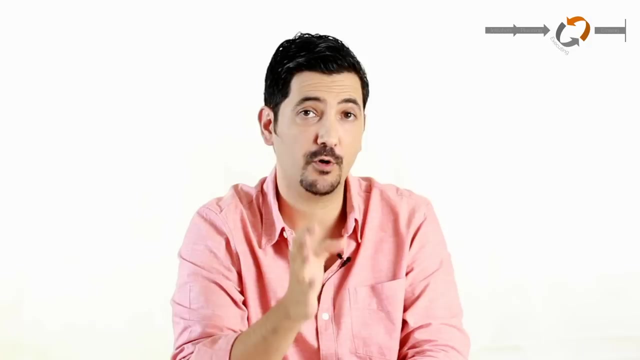 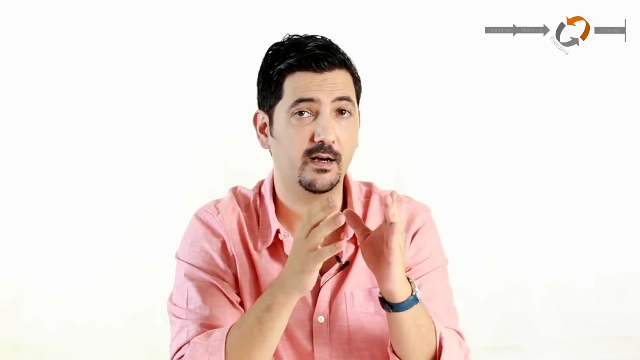 Now, this was the execution. The next process group is called monitoring and controlling process group. Monitoring and controlling means measuring the performance of your project against the plan, Managing your change requests and making sure you are hitting your KPIs if you have included them in the first place. 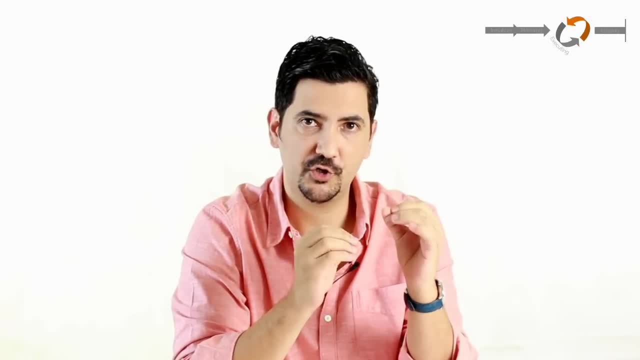 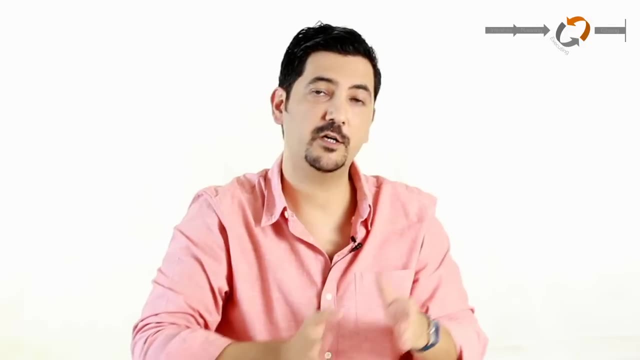 An important aspect here: Monitoring and controlling starts with the execution process group. So they run in parallel. So you monitor and control when you are already in the process group. So you monitor and control when you are already in the process group. So you monitor and control when you are already in the process group. 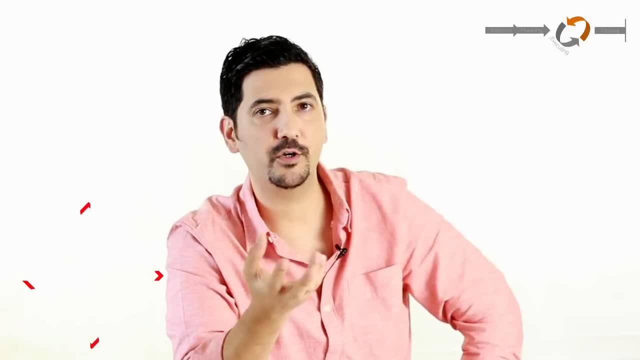 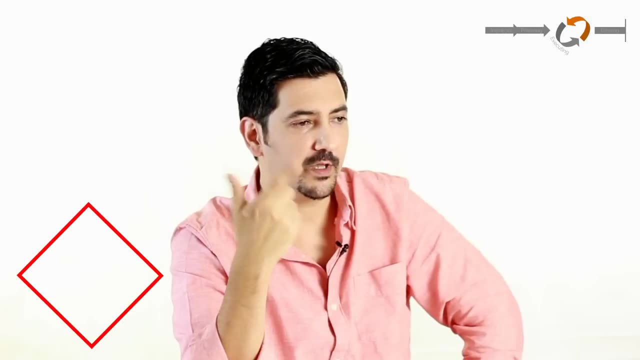 So you monitor and control when you are already executing it. I mean, it makes sense, right? How can you monitor once you finish the execution? So what do you monitor and control then? So you monitor your scope, You make sure no scope creep happens. 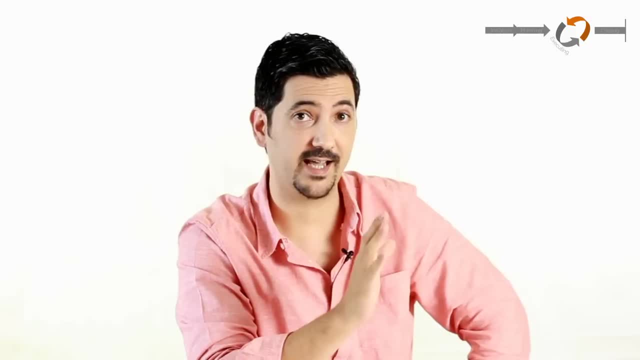 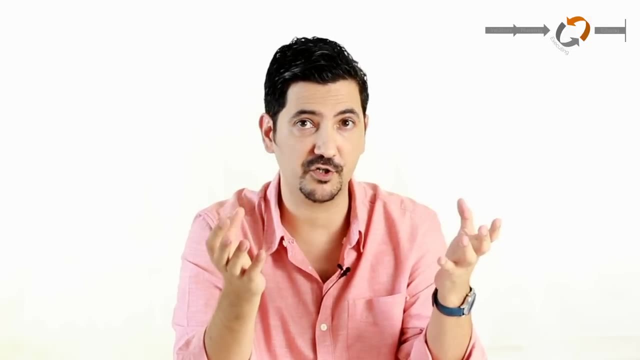 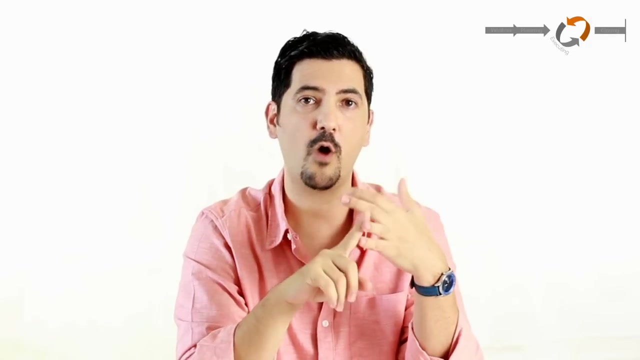 You monitor your schedule And forecast. if you think there will be delays. This is particularly easy to see because you already have your project time plan, your project schedule- Remember we even put it on the Gantt Chart Right. Then you monitor your costs, your quality, your risks and your procurement. 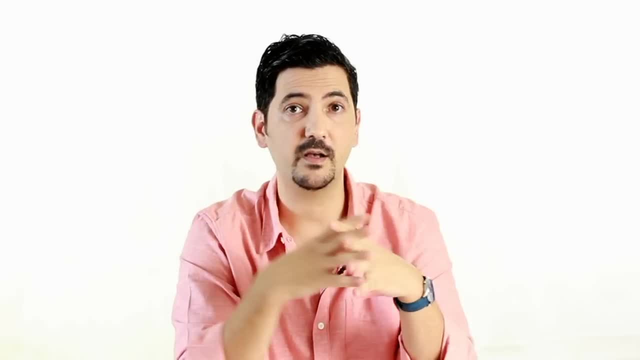 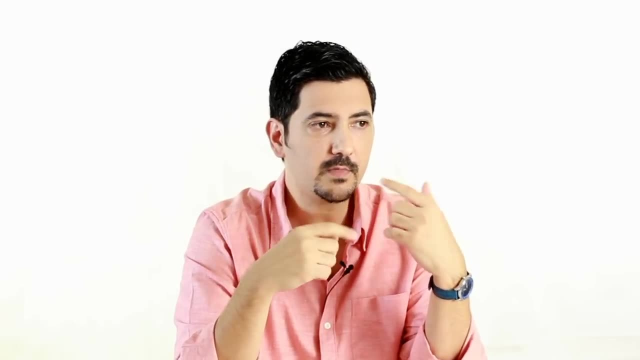 Is procurement happening alright? Are the contractors happy? So this is fairly simple. For example, you finished a particular work package And then you can just always look back and verify if you were within the allowance. If you weren't, then you look for the root causes. 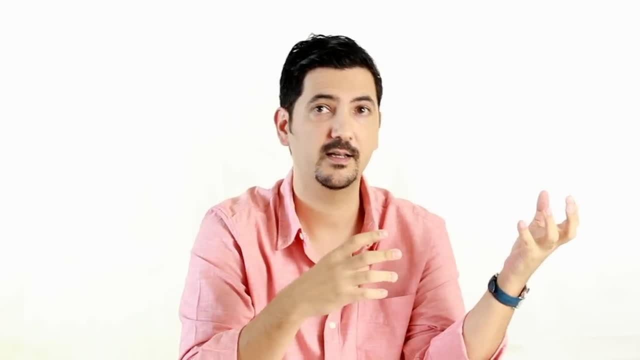 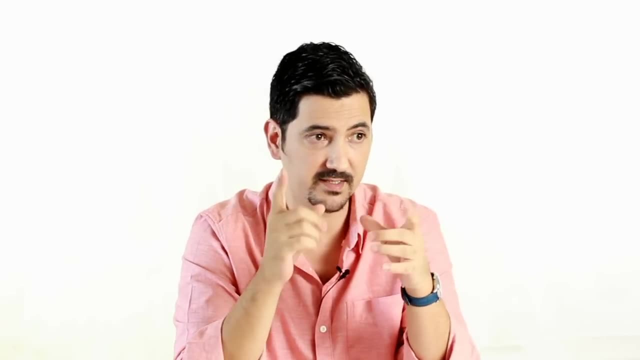 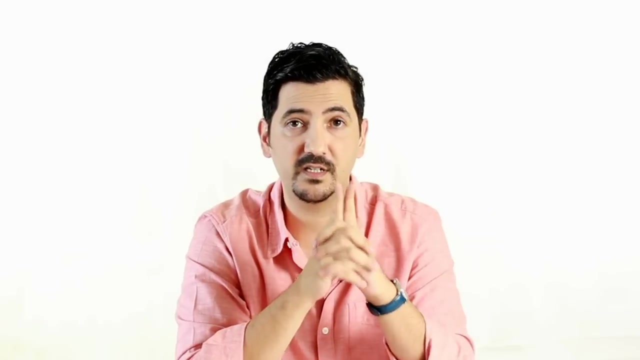 What happened? Why did we exceed the budget or the schedule? And obviously you solve those problems so they won't repeat And you make sure you document everything For PMP takers. please pay extra attention to earned value calculations here. It becomes particularly important in this stage. 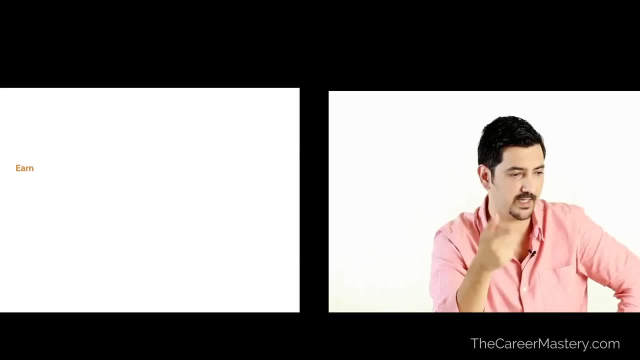 Now I want to quickly touch on earned value. So earned value is the total project budget multiplied by the percentage complete of the project. For example, you have budgeted $1 million And you have finished 20% of it, So your earned value is $200,000. 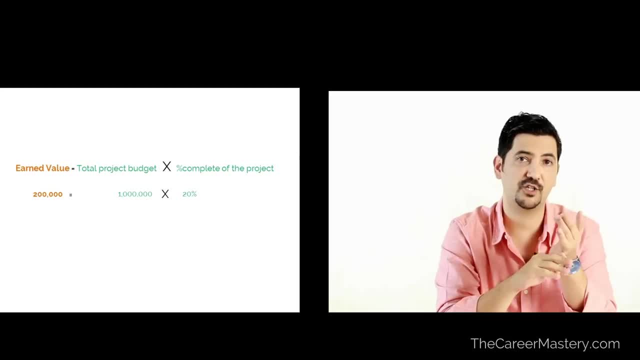 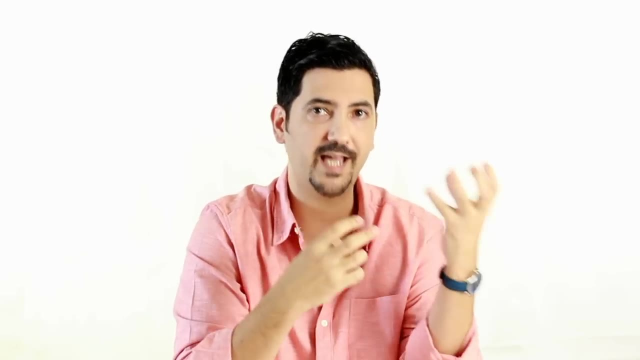 Now this is primarily used for construction and software projects and an important concept by PMI, But in real life it doesn't hold much value other than few industries like the construction and IT, And the reason is The value gained cannot always be assessed alone. 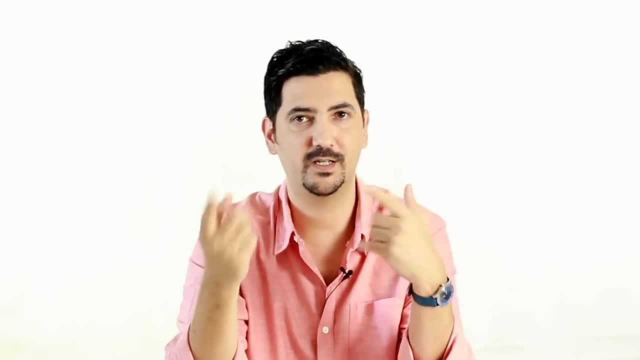 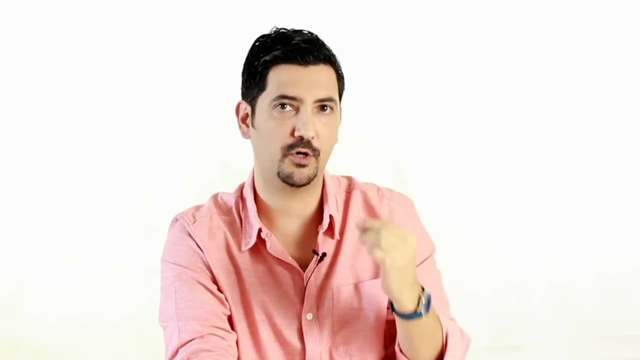 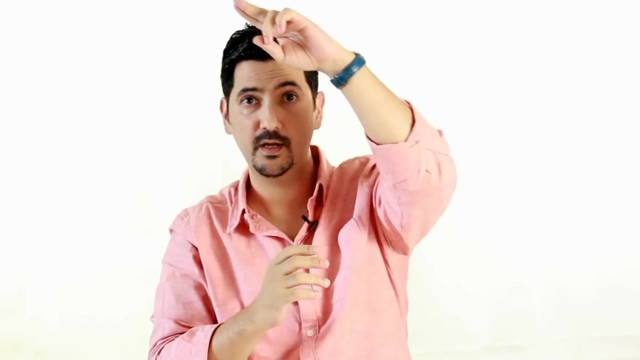 What does this even mean? It means it's not always a linear progression. Most of the time, the actual value of a project goes like this. So it's not linear, It's a power curve. Most projects show exponential growth instead of a linear one. 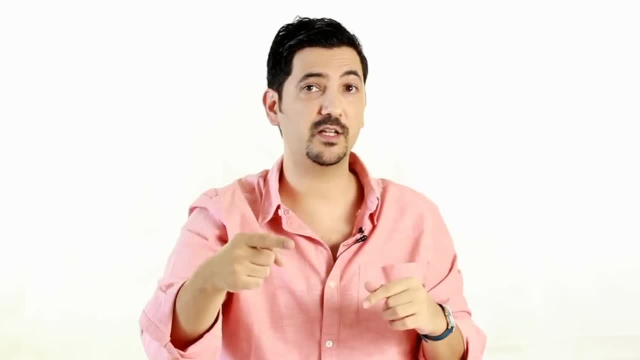 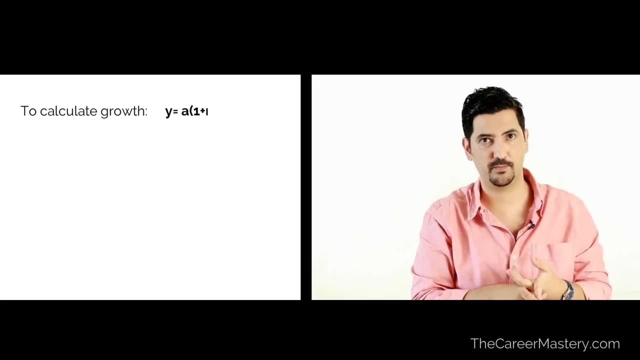 And they get compounded results every month And their calculation is a lot more difficult than a simple y equals to mx plus b. To calculate it you need a growth decay function. So you need a growth decay function. It's a very complex one. 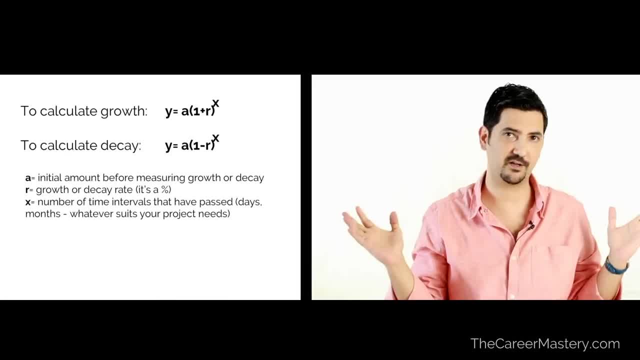 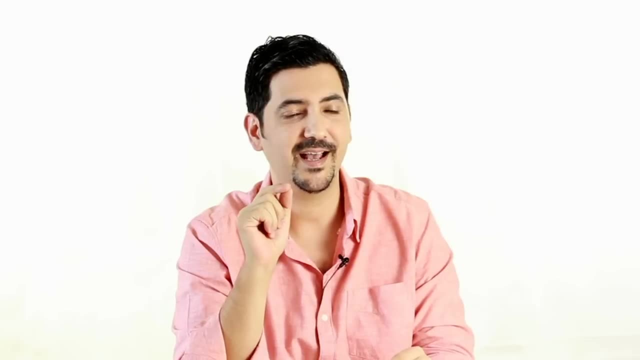 And no project manager is going to run that every week just to calculate the earned value. This one is very similar to how we calculate compound interest. So before I bore you to death, let's move to closing process group. Actually, no, I want to explain this just a bit more. 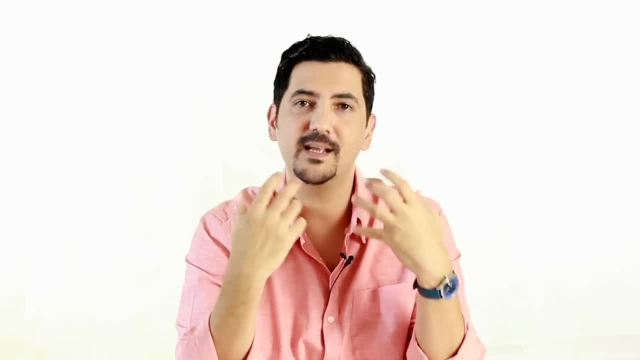 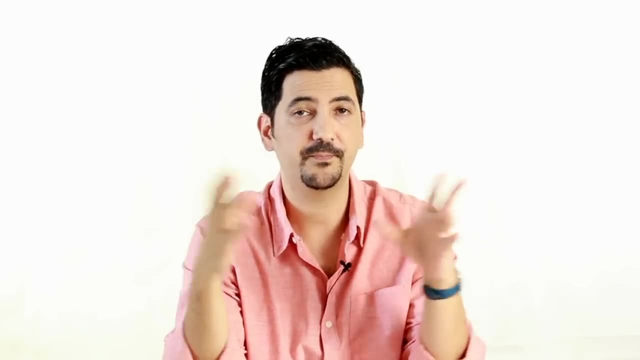 The exponential growth theory, because I believe you'll benefit from it. So let's take my YouTube channel, for example. Let's call this project Project 100,000 subscribers. That's what I'd love to achieve. At the moment, I have about 19,000 subscribers. 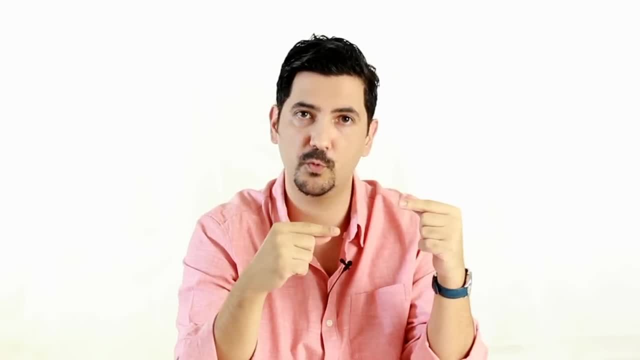 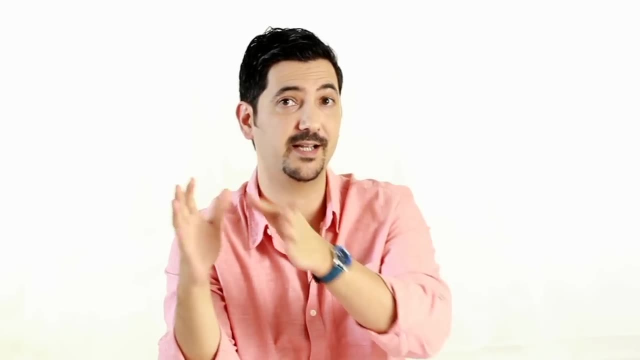 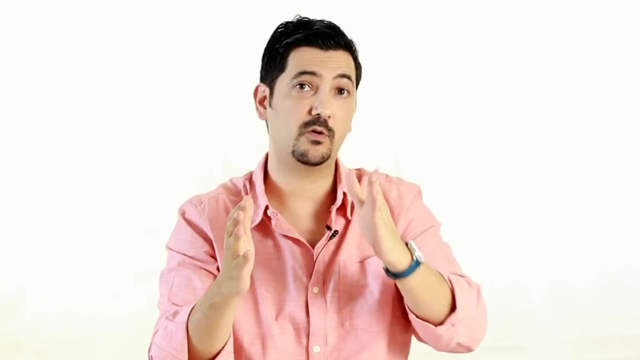 So let's say I get 500 subscribers per week with 20 videos. If I have 40 videos, provided that I maintain the quality, I will not have 1,000 subscribers per week. It'll probably be 2,000 per week or a lot more because it gets compounded. 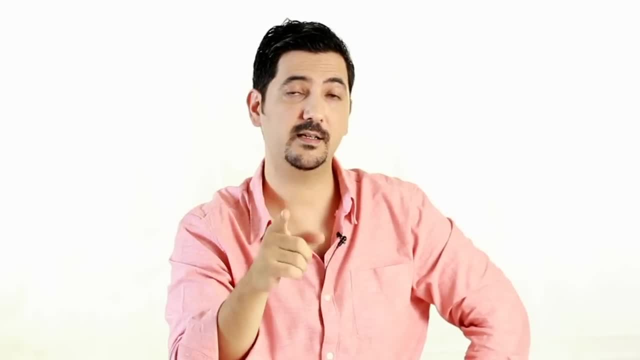 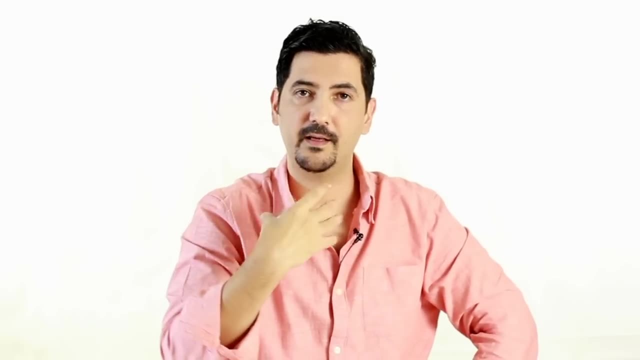 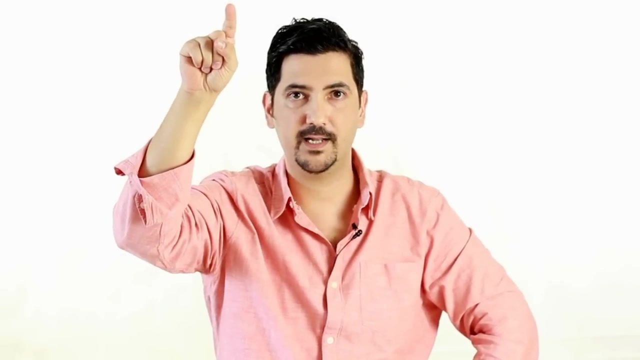 Just like your money in your savings account. See, if you calculate your earned value based on your execution, then you'll get confused. I mean, think of it this way. I'm still putting out about 1 video per week, But it all of a sudden just became exponential. 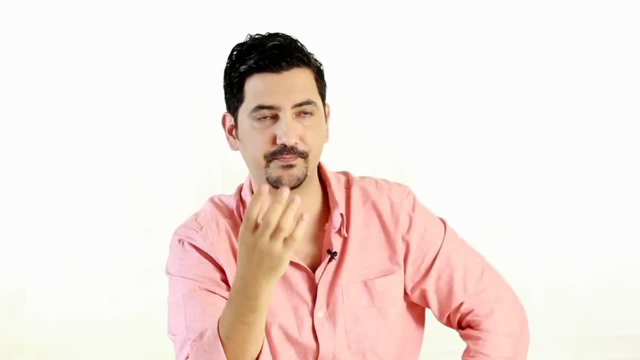 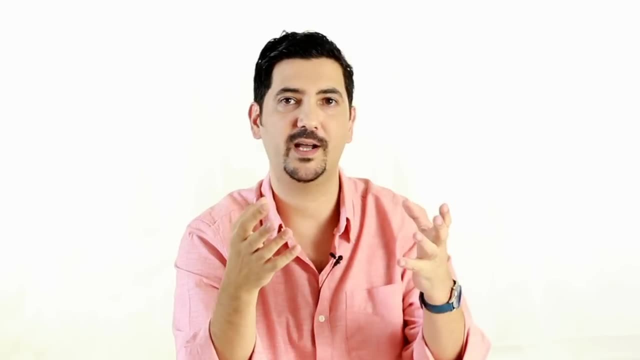 So that's how most projects are in real life. Ok, sorry to have taken your time. I digress a little bit there. So the key takeaway is: Whatever your project is, don't quit just because you don't see the results now. 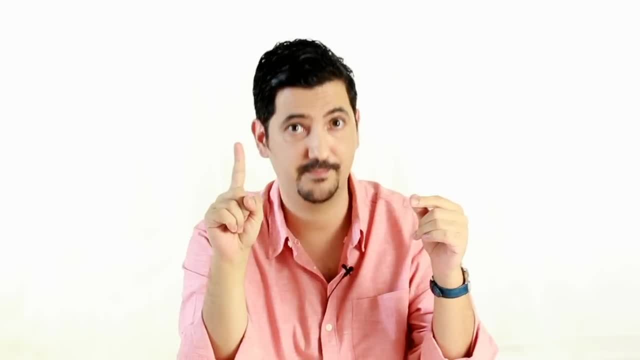 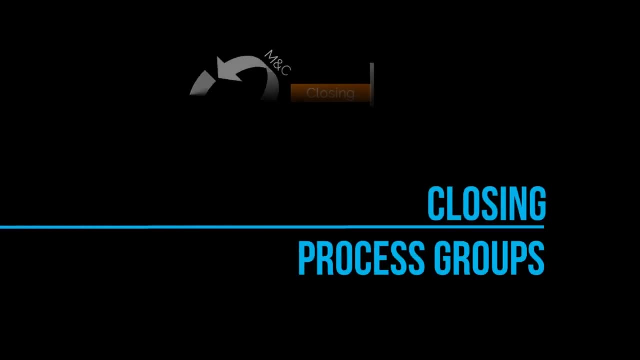 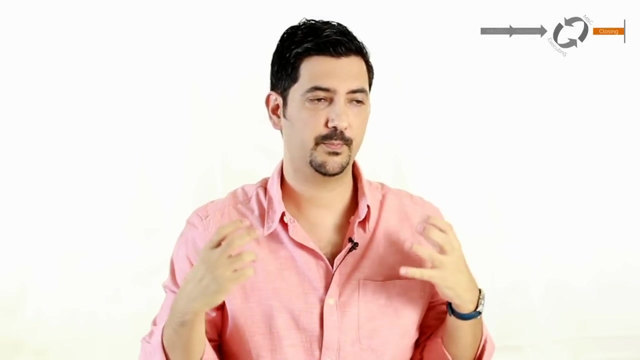 They will come And when they do, they will come like that: Ok, Let's do closing, Let's close this project. Now, we finished the product, the end result: We have the boat, It's completely finished. But is there a reason? 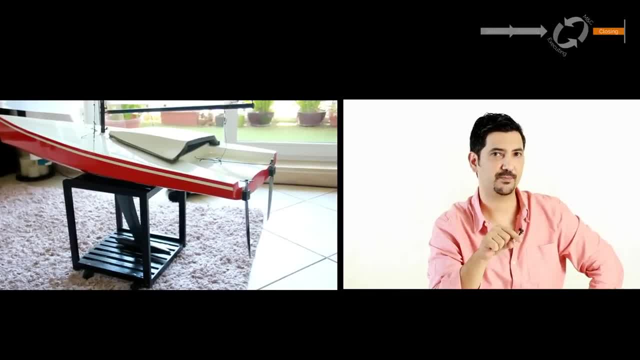 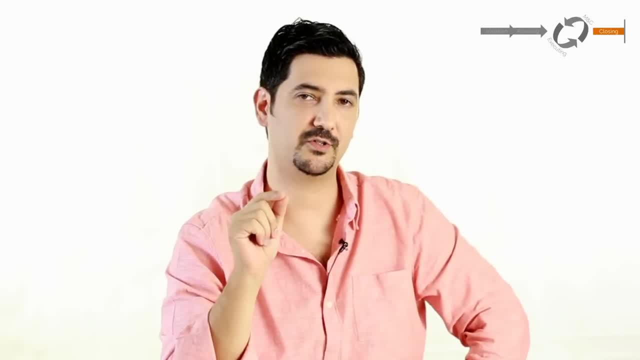 Is the project finished? I mean, the product is finished, But the project? No, It's not. Not yet. There is still some work to be done. Not much, But we still have to do certain things, And mostly boring admin work. 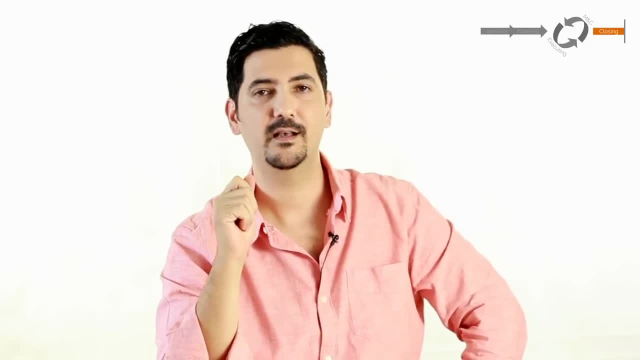 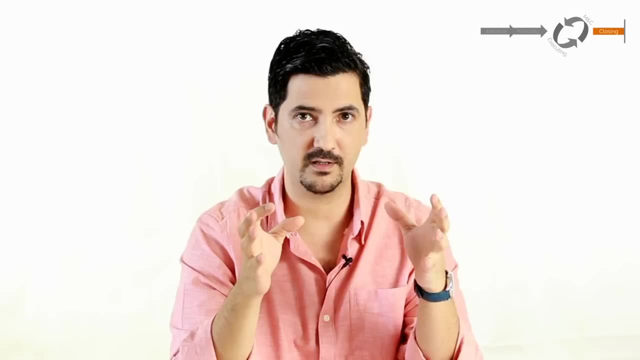 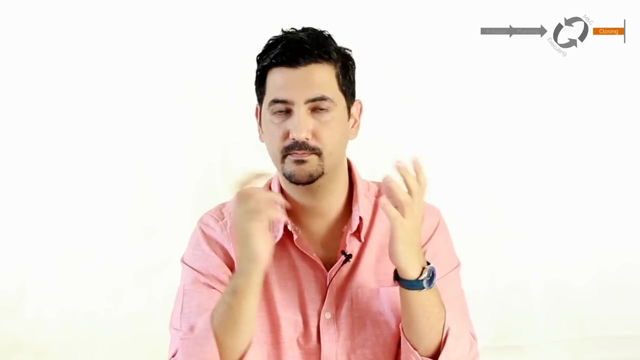 So what do we do now? Well, what you do is well. it's actually really customizable to the needs and complexity of your project. But, in general, what I am going to share with you are good starting points. 1. We handed over the end product to the client. 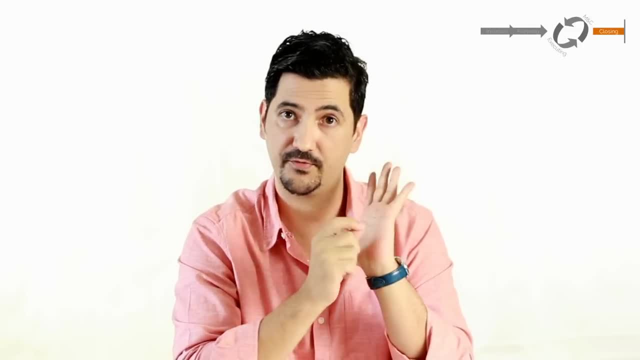 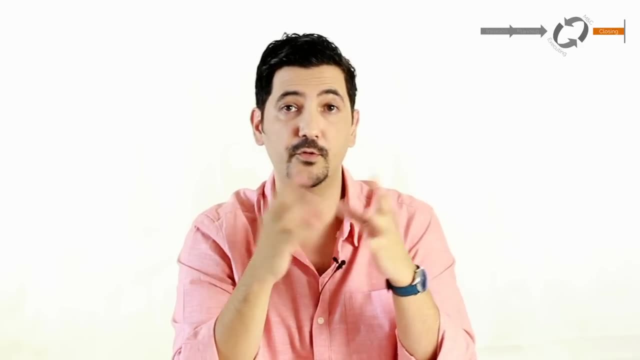 If it's a project you did for a client, you need to basically get a sign-off from the client that says ok, I received the possession of this item, And then they sign it off. 2. And then you finish procurements. 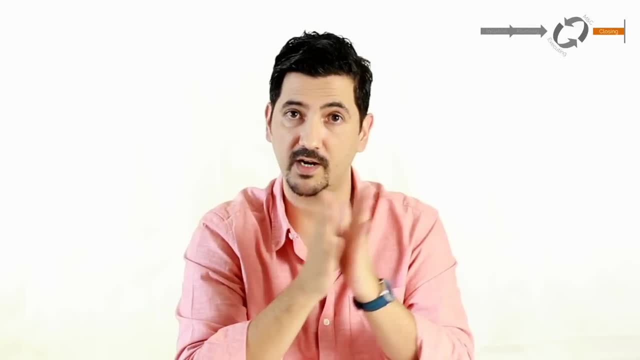 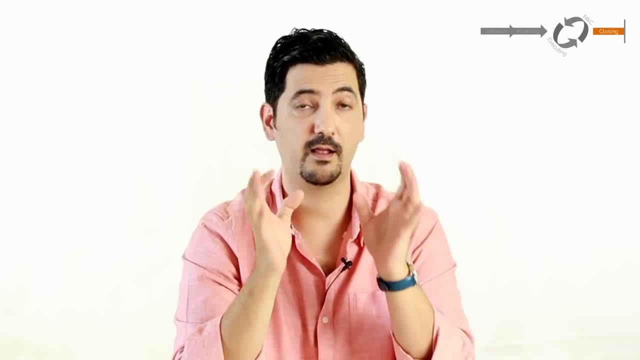 Meaning you need to make the final payments and complete your cost records, And then you need to gather your final lessons learned. This is basically documenting what went wrong and what did we learn from it: 3., 4., 5., 6.. 7., 8., 9., 10., 11., 12., 13., 14., 15., 16., 17., 18., 19., 20., 21., 22. 23.. 24., 25., 26., 27., 28., 29., 30., 31., 32., 33., 33., 33., 34., 34., 35., 36., 36.. 37., 38., 38., 38., 39., 39., 40., 41., 41., 42., 42., 42., 43., 44., 44., 45., 46.. 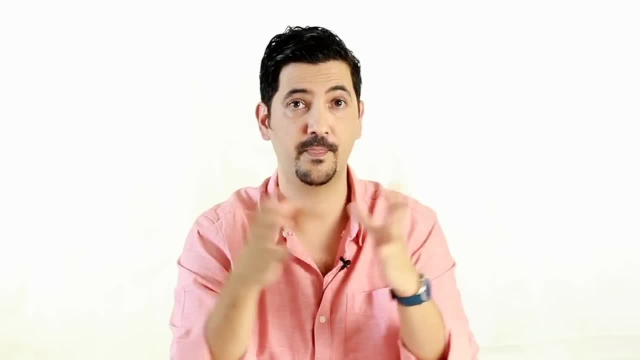 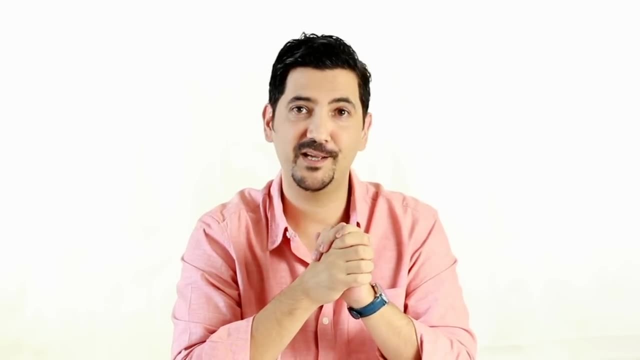 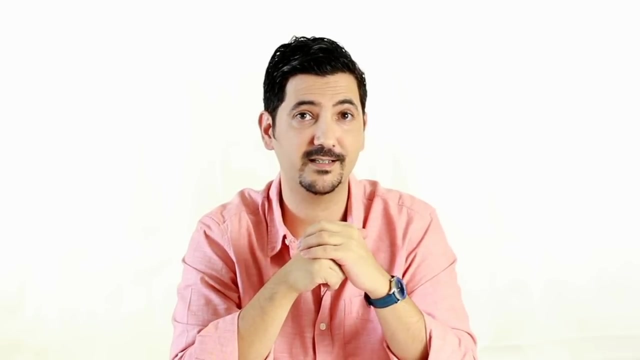 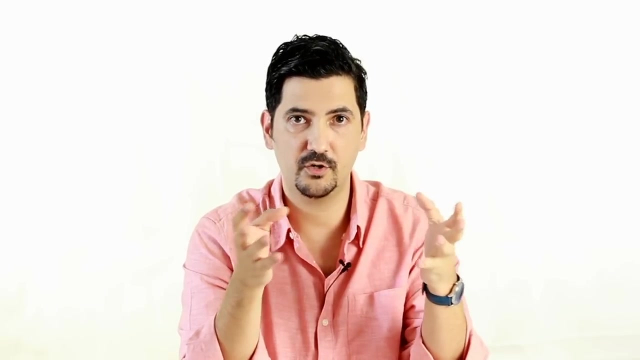 46., 47., 47., 48., 49., 50., 51., 52., 53., 54., 55. I'd love to connect with you And finally, as I mentioned earlier, if you are looking to make a big jump in your career, 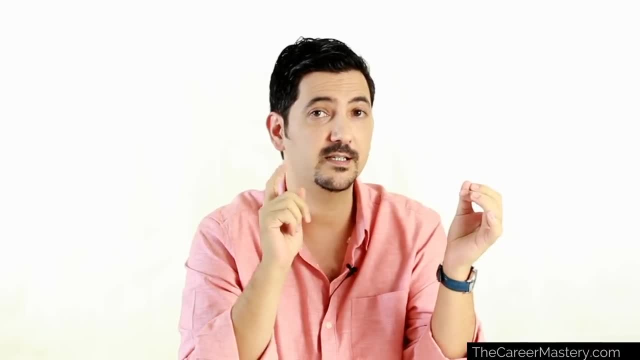 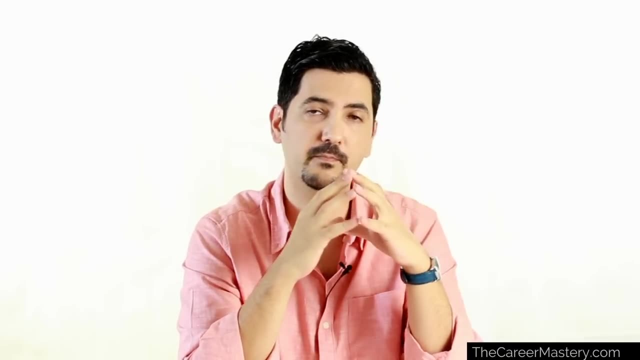 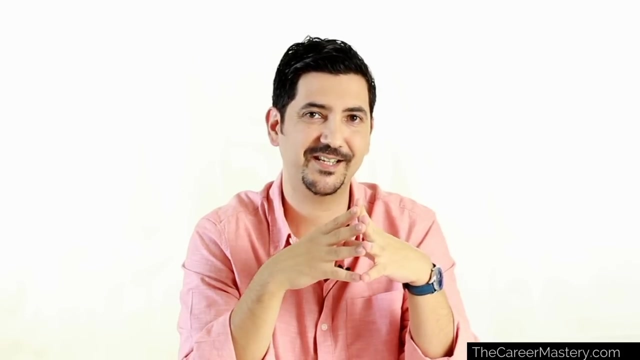 and explore working for a multinational organization companies, consider joining my LIG program. that's where I share some of the advanced strategies to getting yourself employed by amazing multinational firms. It delivers great results And alright, we're done. See you next week. Subtitles by the Amaraorg community. 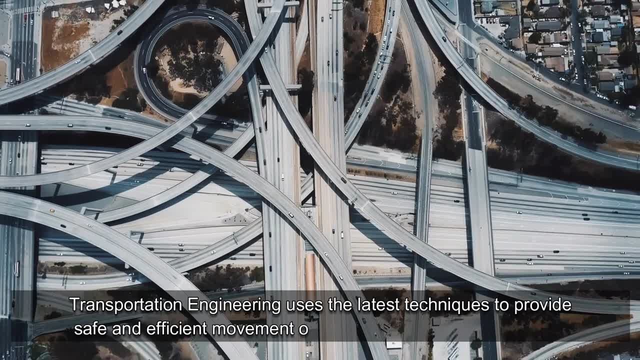 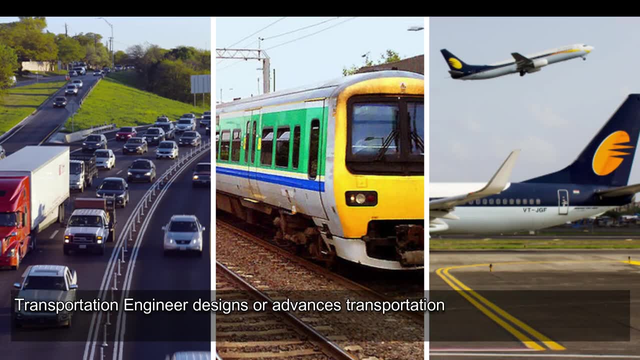 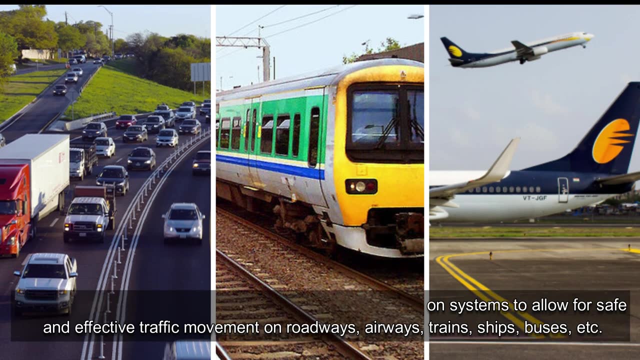 Transportation engineering uses the latest techniques to provide safe and efficient movement of traffic from one place to another. Transportation engineer designs or advances transportation systems to allow for safe and effective traffic movement on roadways, airways, trains, ships, buses, etc. Why transportation engineers are in demand and